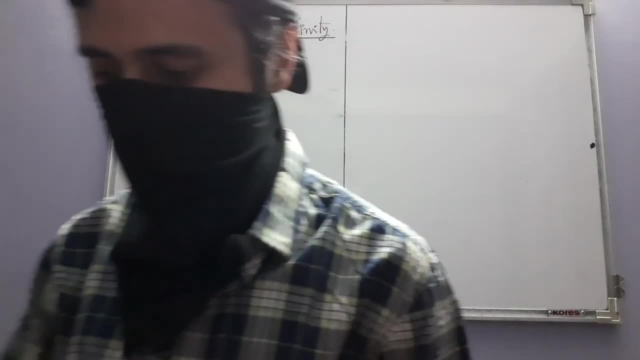 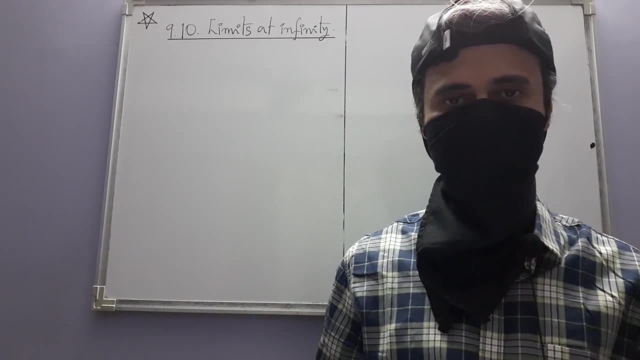 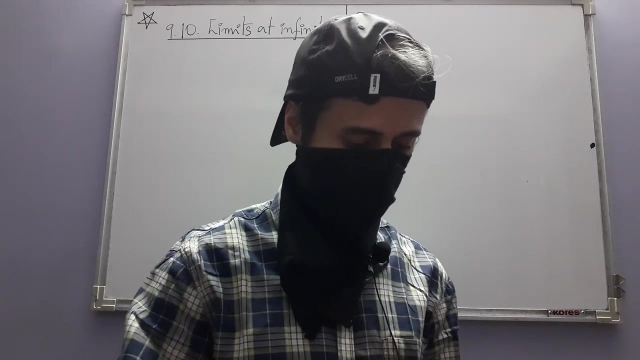 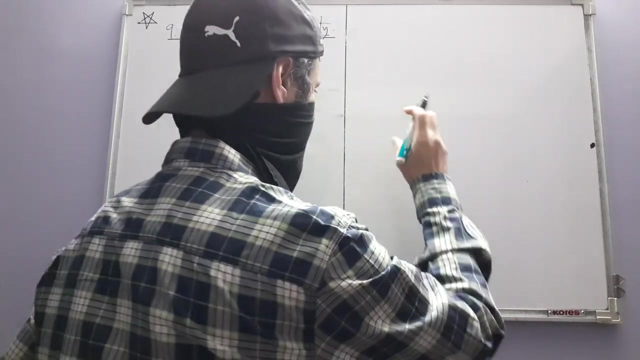 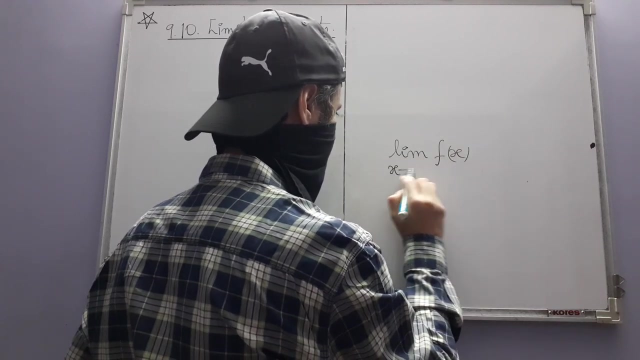 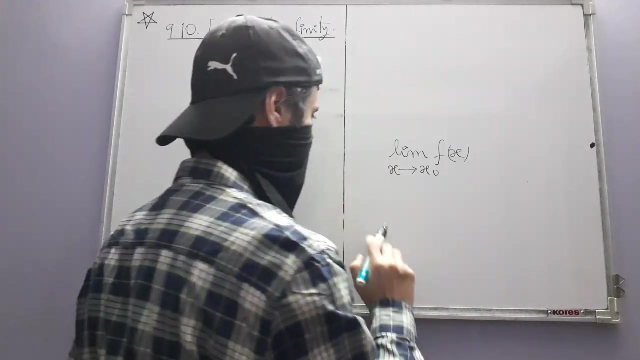 Okay, so we have reached the last section of this chapter, And this section mainly just defines one thing, that is, limit at infinity. Note that we have already seen this limit of a function, f as x approaches x naught. We have already seen this when x naught is. 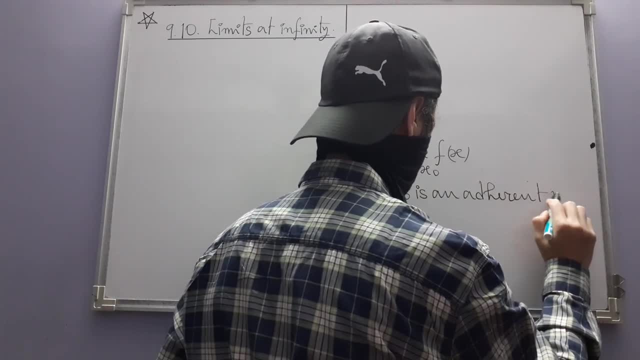 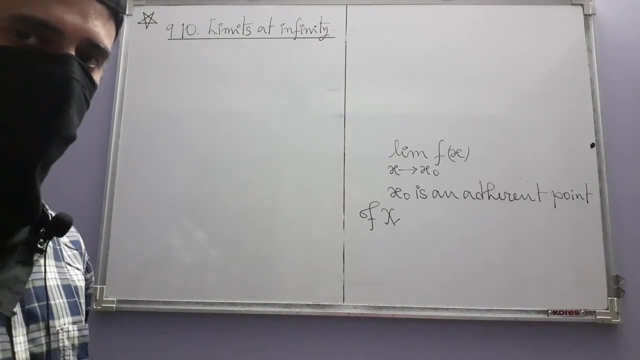 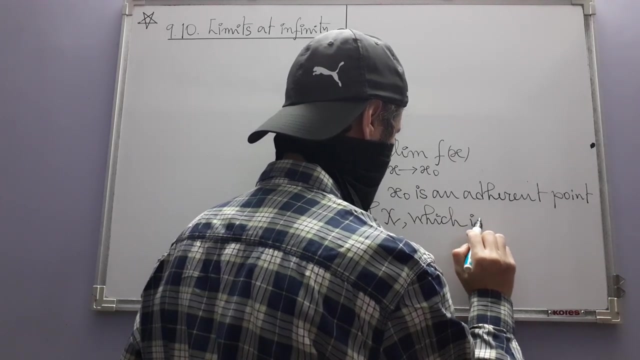 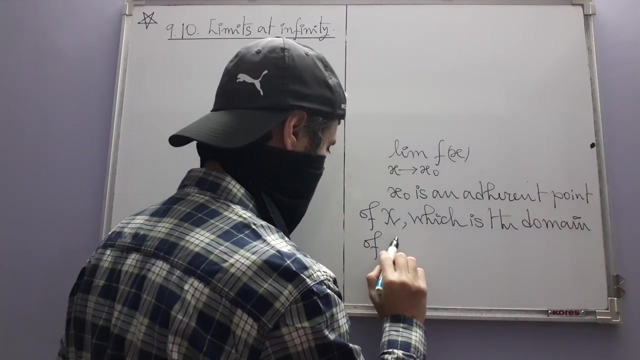 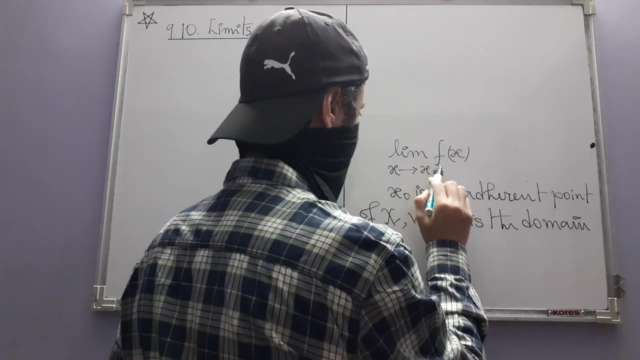 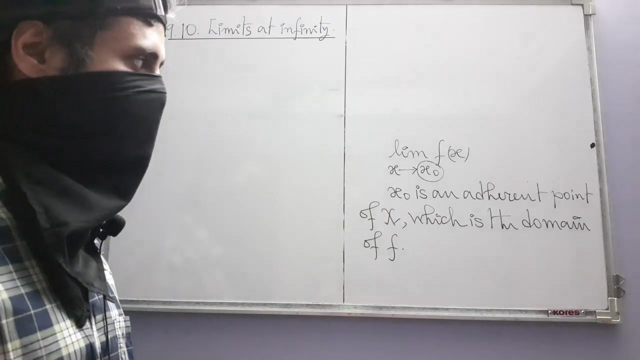 an adherent point of capital X, which is the domain of the function f. f, of course, is real value. Now, what we are going to do, we are going to consider plus infinity and minus infinity in place of x, naught, And then we are going to ask the same. 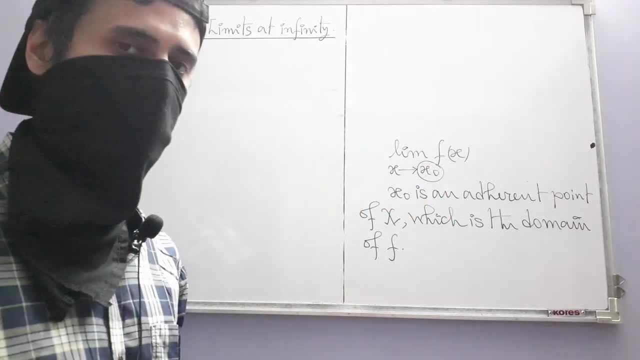 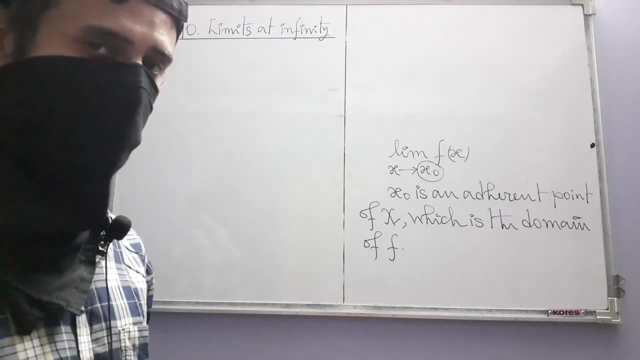 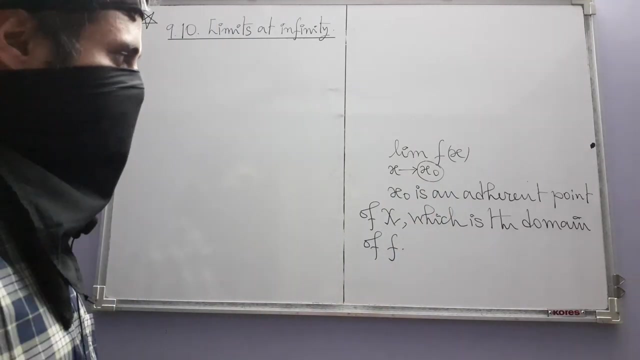 thing. What possible meaning can we assign to this notation, this symbol? Can we somehow meaningfully define limit in that case also, or actually in two cases, namely: here you can have plus infinity and also minus infinity. So for that we need this first of all. X naught originally. 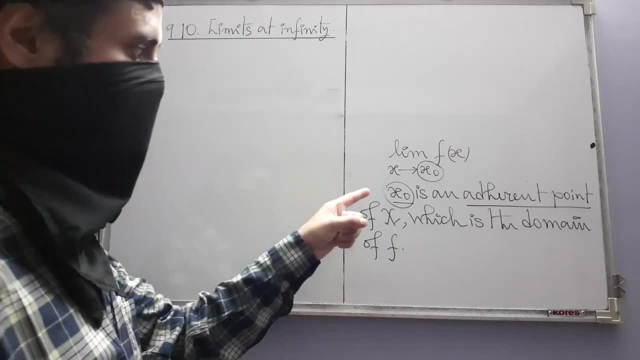 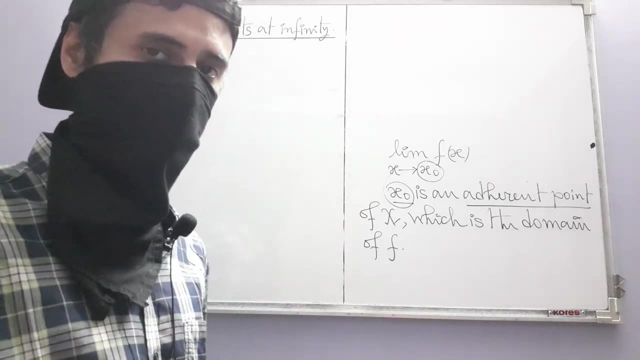 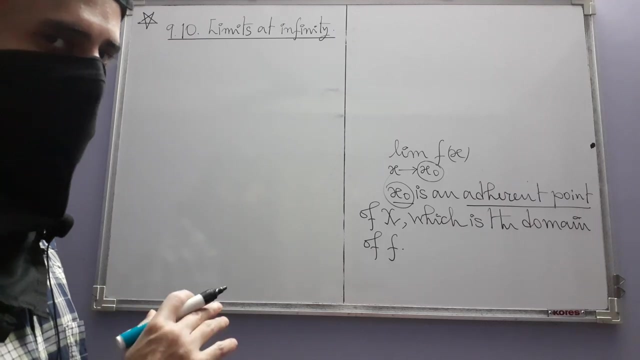 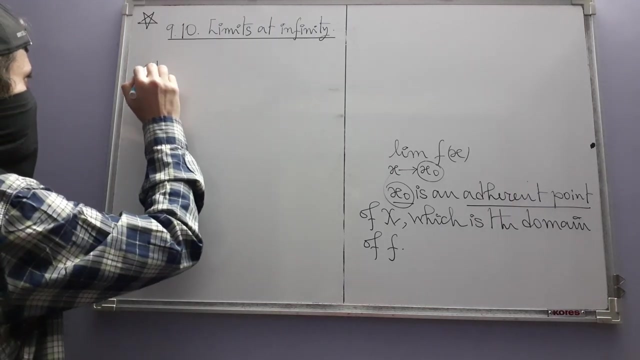 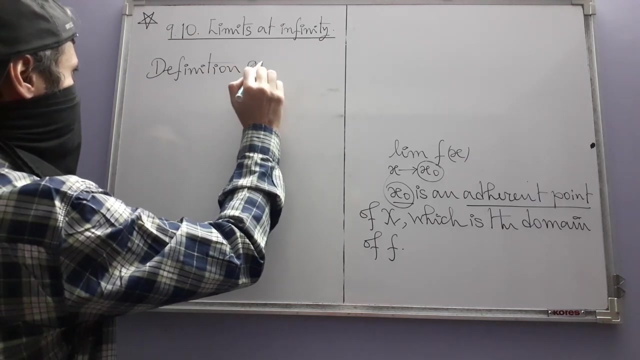 in our old definition, the original definition of limit, in that x naught is after all a real number. But now we want plus and minus infinity to be adherent points of the domain of f. So it is with that definition that this section starts. So let us start like that. This is: 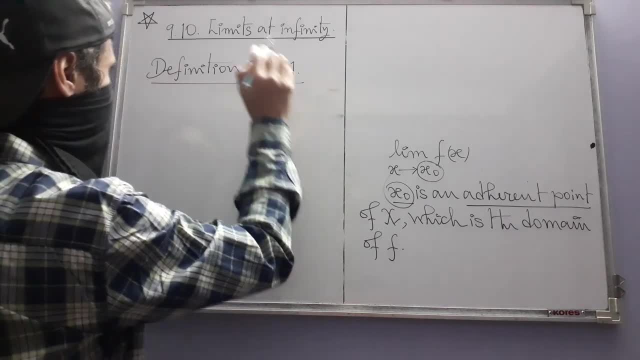 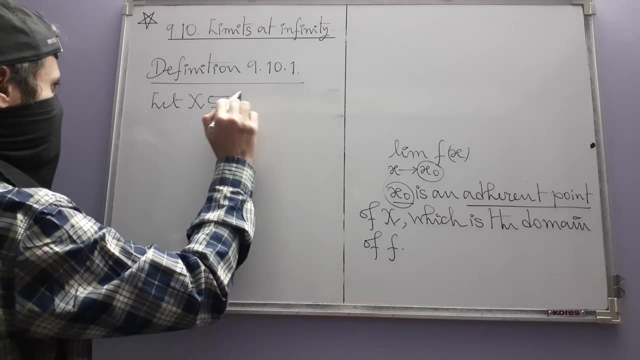 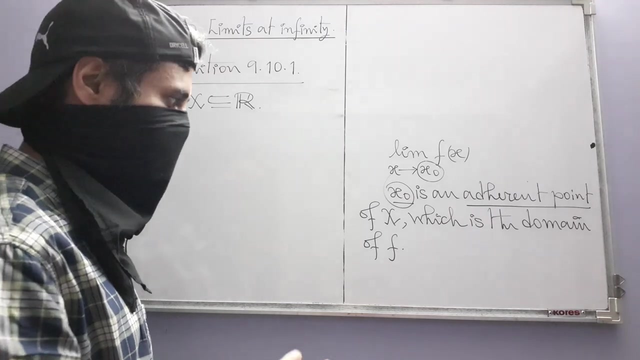 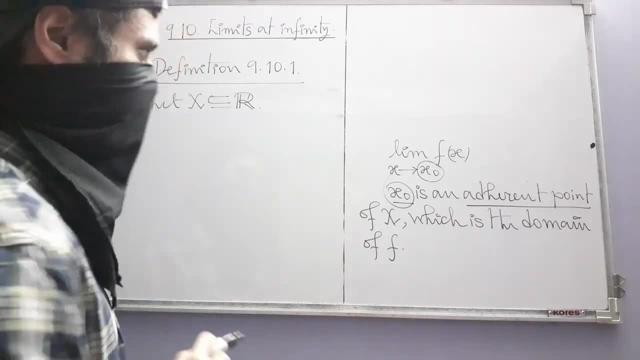 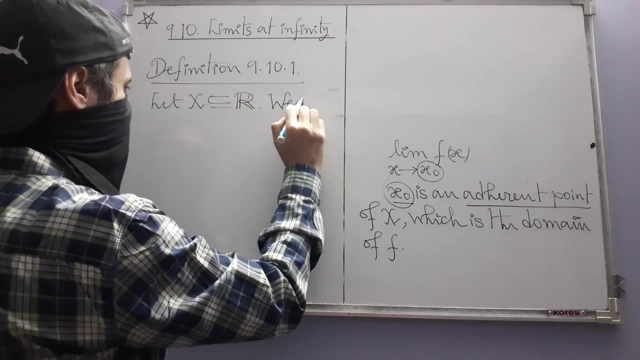 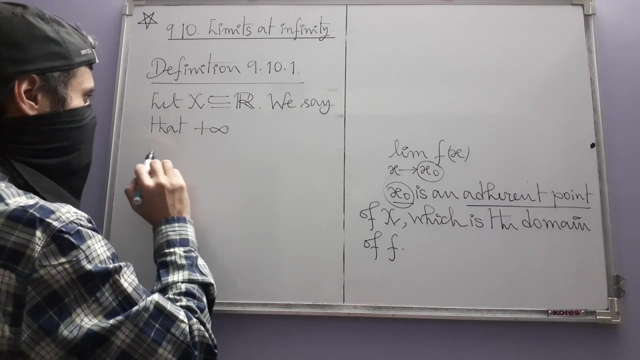 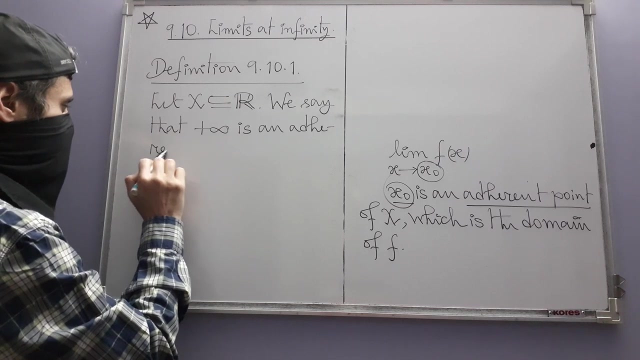 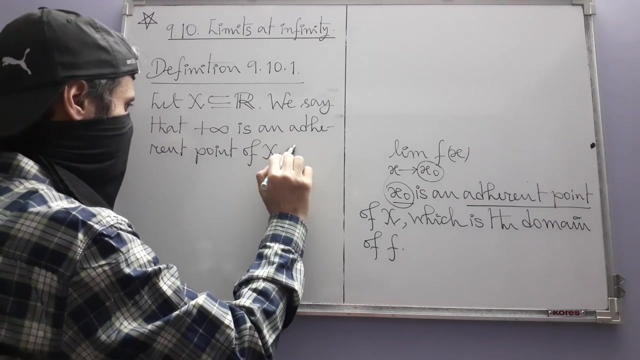 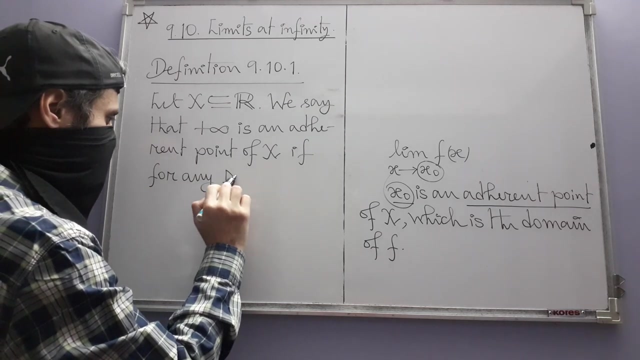 function. but then while defining limit, function will have to be considered. So let x be a subset of r. We say that intfcr minus infinity, Exception 9.10.1.. plus infinity is an adherent point of x. if for any real number m. 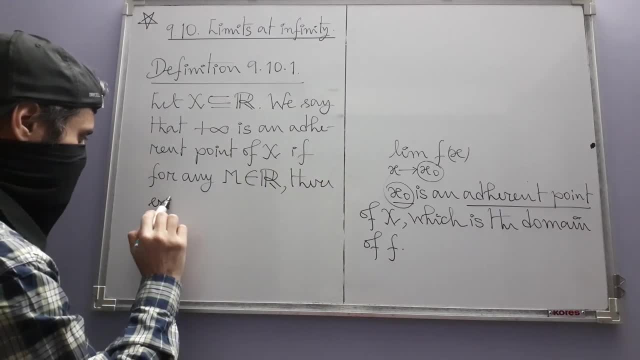 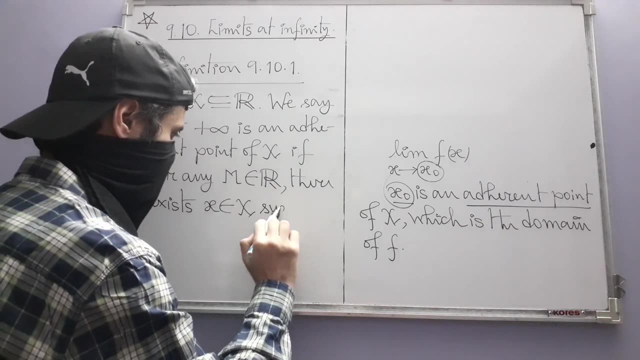 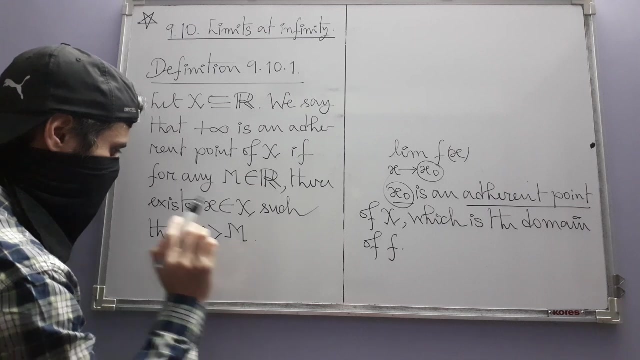 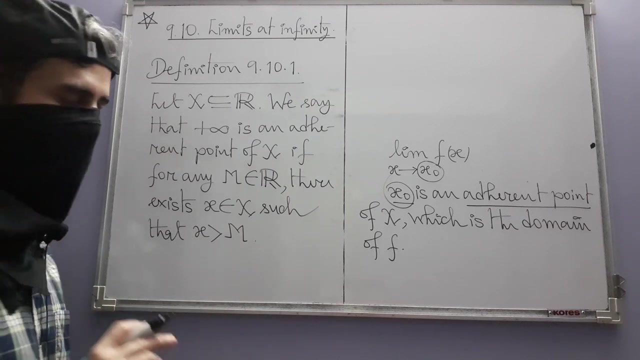 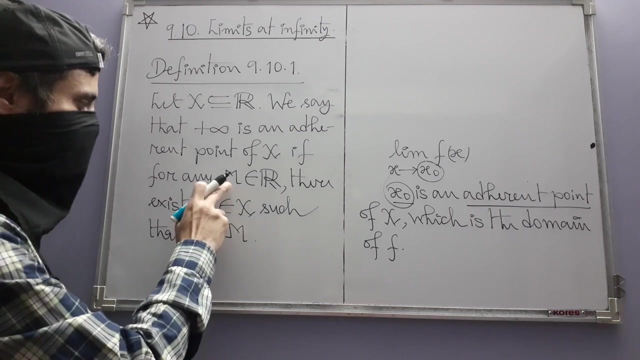 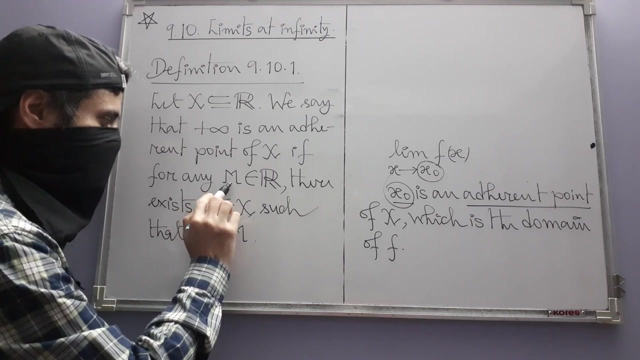 there exists x belonging to x, such that x is greater than m. x exceeds m. so, putting it more simply, this condition just tells us that, no matter what m we take, choose- and in fact our tendency is towards choosing large and large, larger and larger m. no matter how large m is, x still has a larger point in it, so x is. 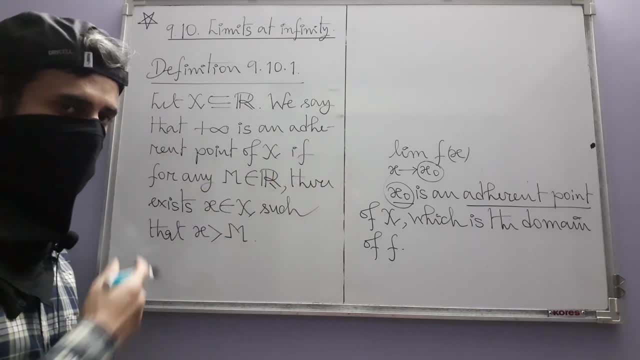 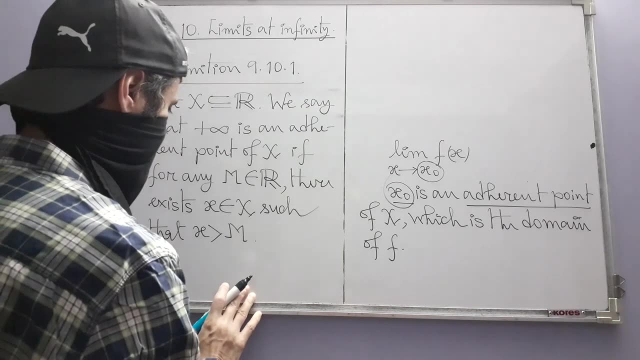 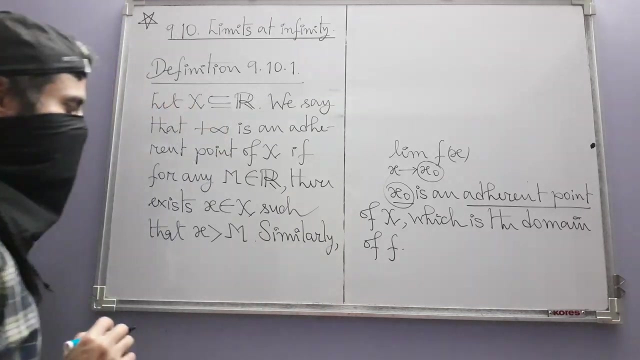 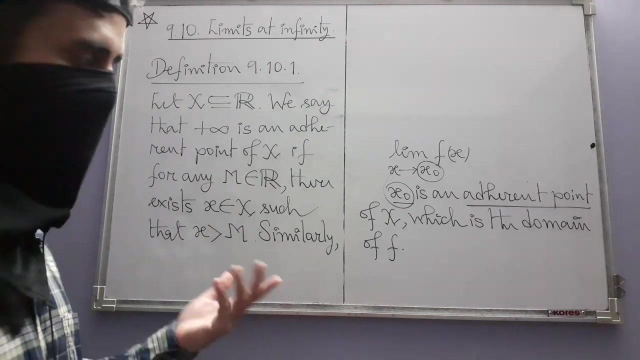 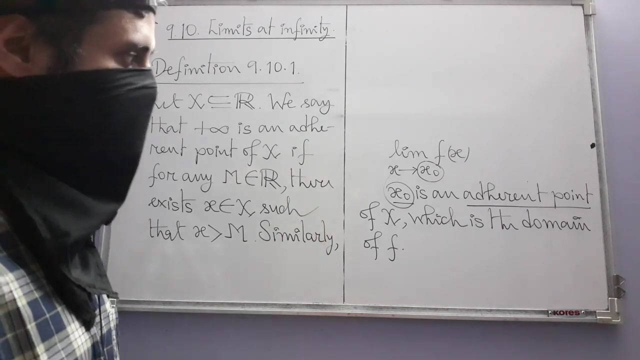 unbounded in that sense, towards that side, okay, towards the positive side of the real axis. similarly, and when that happens, we say that plus infinity is an adherent point of x. you can understand why this definition makes sense and why this one also we are calling an adherent point because you see, in the original definition where x 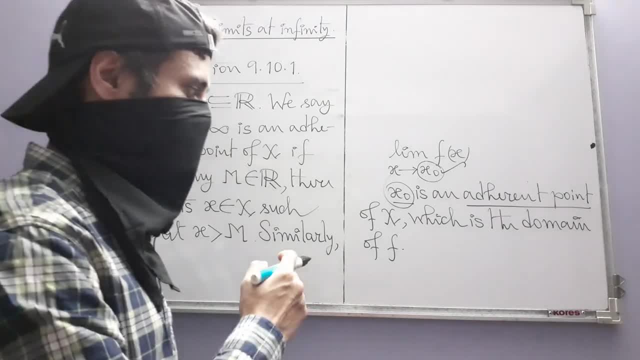 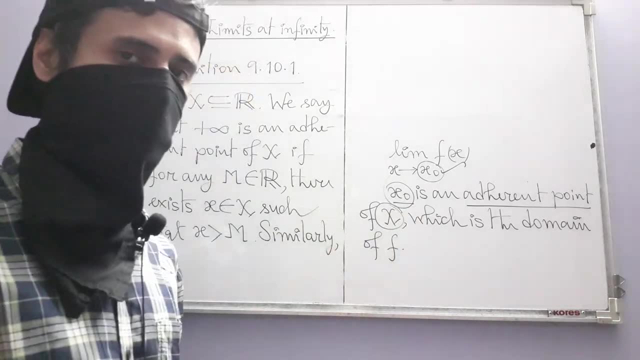 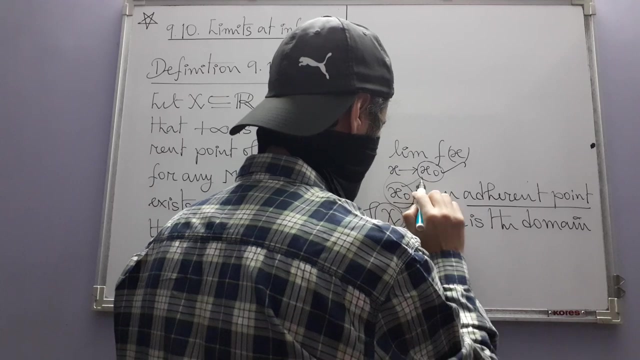 not was a real number there. x not being adherent to x meant what? it just simply meant that x naught is very close to x, as if it's touching x. The precise definition, of course, is that in any neighborhood of x naught there is at least one element of x. In this case, 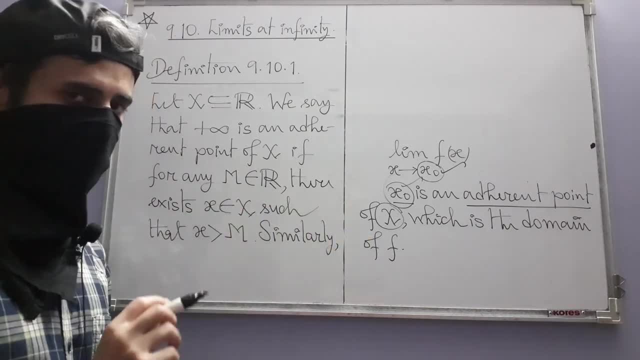 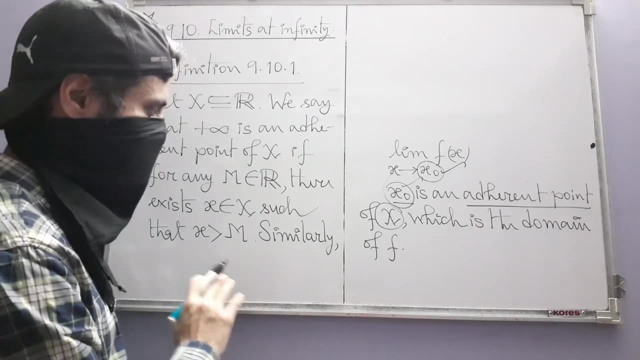 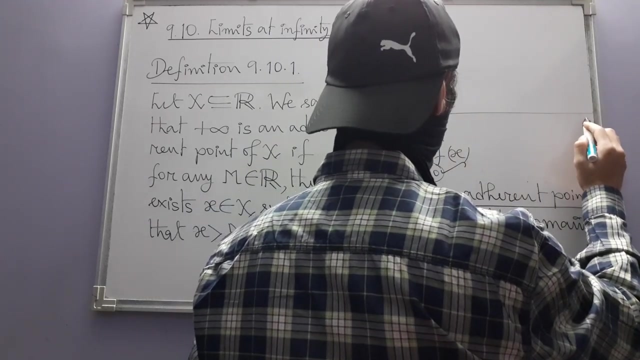 that neighborhood of infinity, of course, I mean we cannot define it in terms of neighborhoods that we have seen so far, But still we can kind of imagine a neighborhood of infinity to be something like this. I mean, infinity, of course, is not something that lies on the real line, It's not a real number. 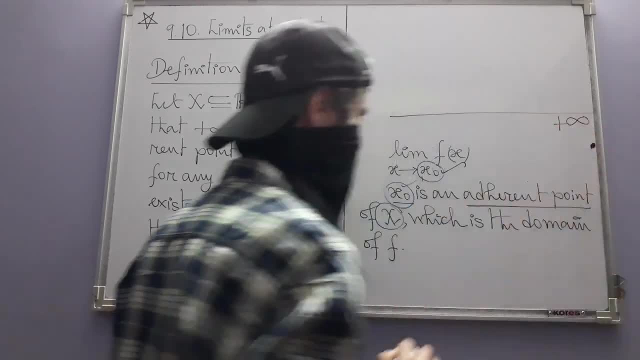 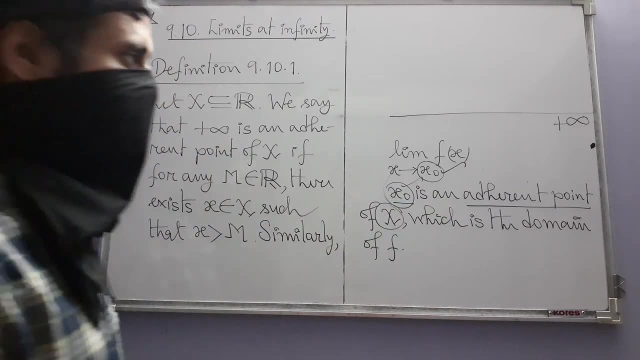 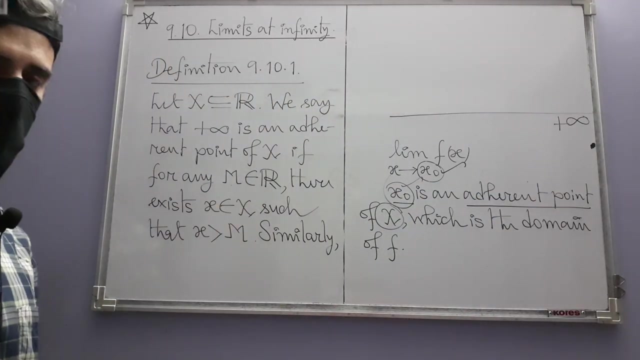 but it's towards that. So this is kind of a vague thing just for us to see that this definition is somewhat like the original one itself. So plus infinity is towards that side. When we say we are taking m in r, actually what that does is that it defines a ray. 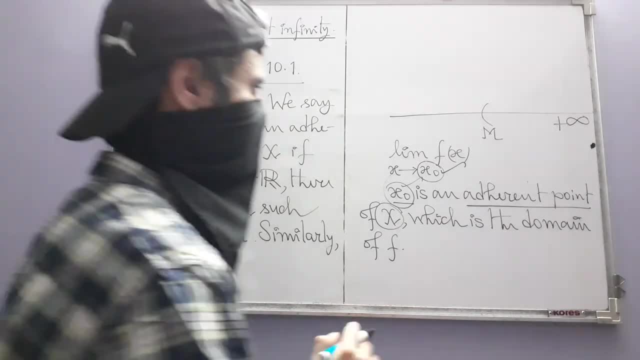 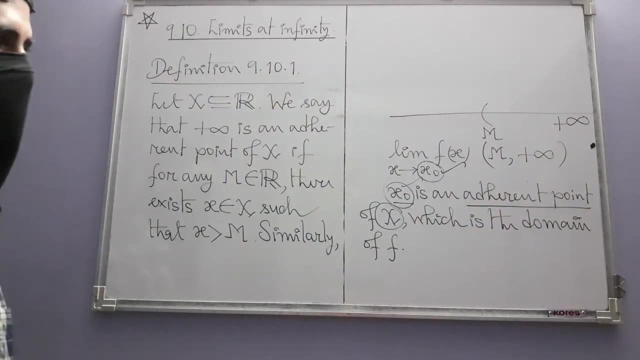 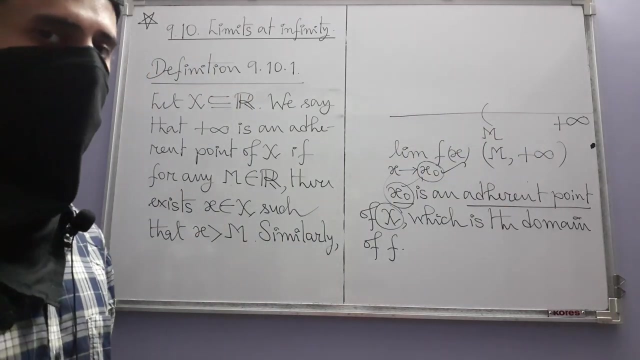 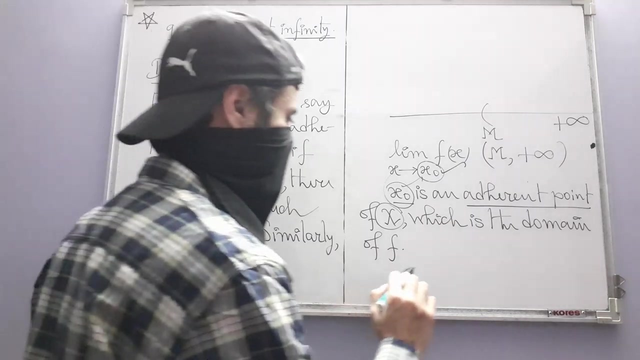 A ray which goes towards that side, and that ray is this: More precisely, it is this open interval. So this itself you can call a neighborhood of plus infinity, although actually it is not Okay, But still it is somewhat like a neighborhood of x naught, where that neighborhood looks like this: 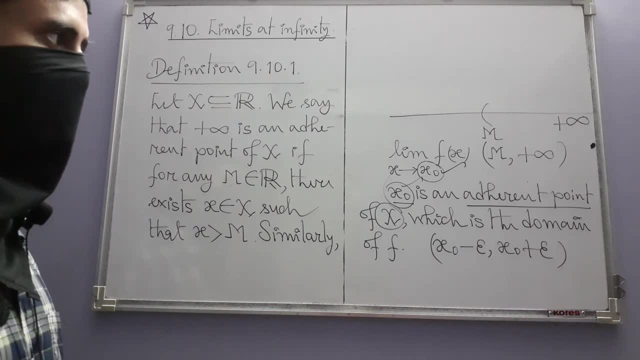 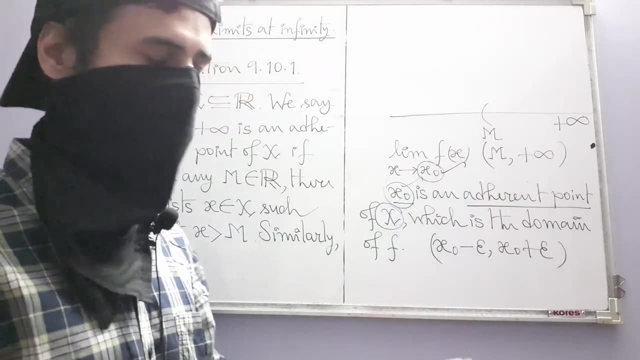 Okay, It is something that contains x naught, and it is very small. This one, however, does not actually contain plus infinity. That's why I said that it's not exactly a neighborhood of plus infinity, but it is somewhat like a region that is very small. So this is a neighborhood of plus infinity. 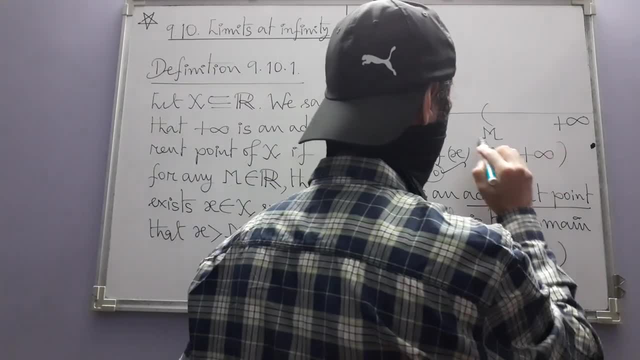 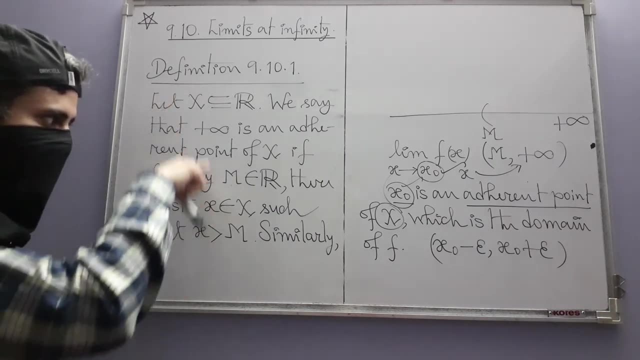 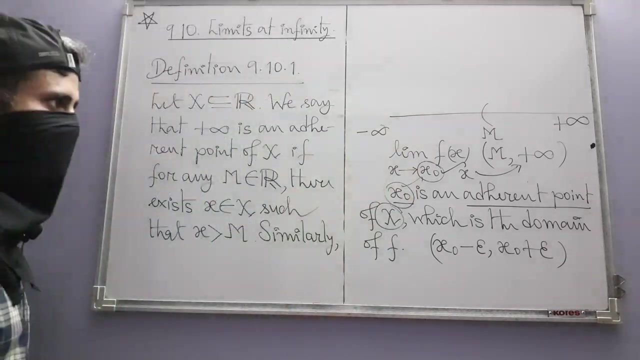 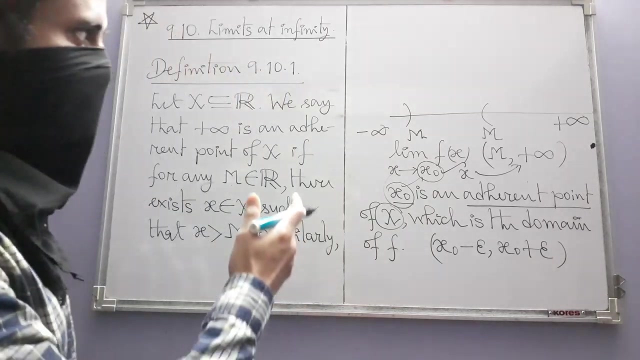 It is towards plus infinity, and that region has at least one element of x because of this inequality. That's why the definition has this condition. Similarly, minus infinity is towards this side. So now we would want again, if you choose an m, some m. In this case, the focus will: 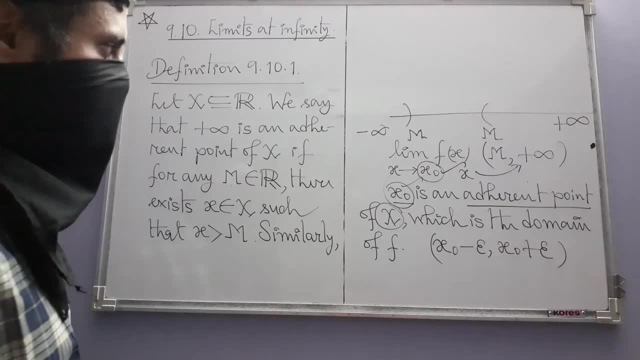 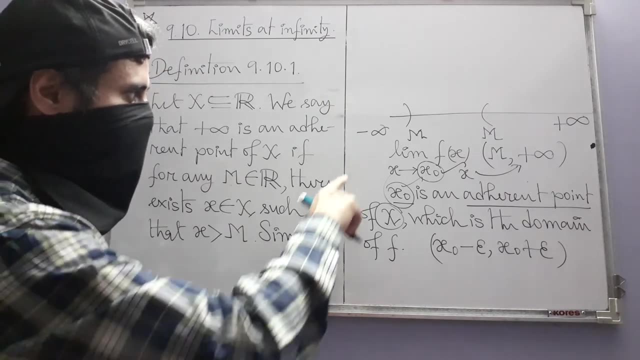 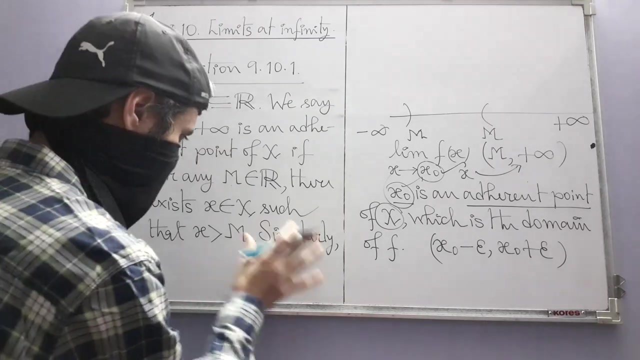 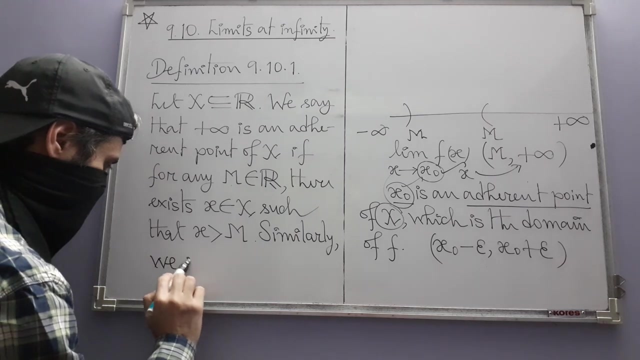 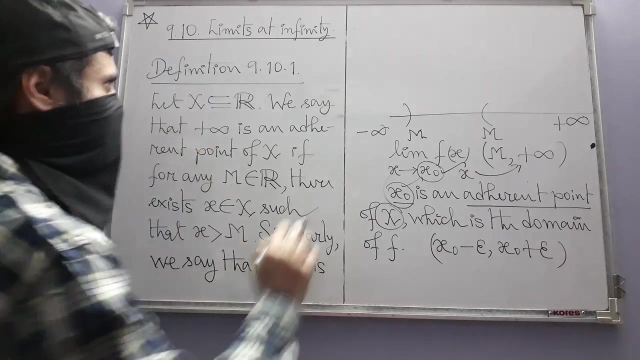 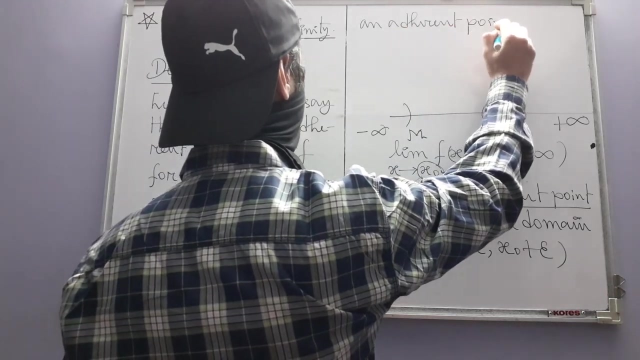 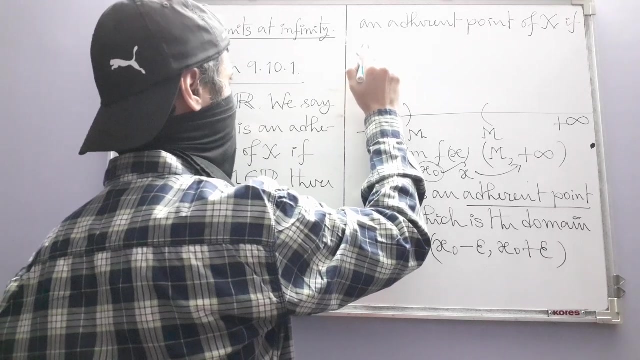 be on the to the left of m, So the state is unbounded on this side. When that happens, we are going to call minus infinity an adherent point of x. The precise statement is this: Similarly, we say that minus infinity is an adherent point of x if, for every m 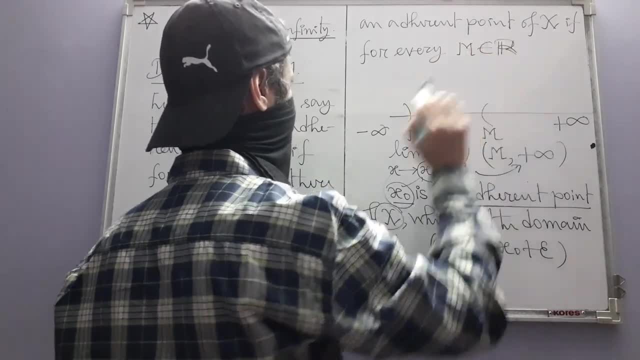 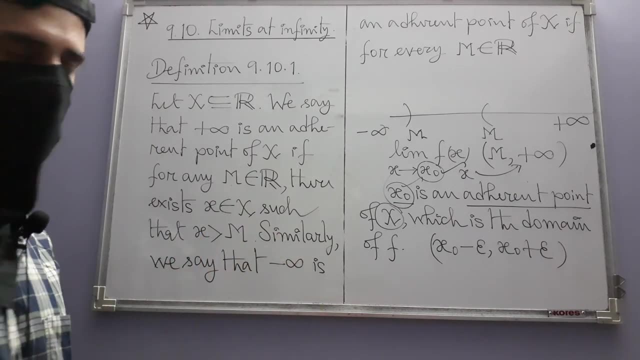 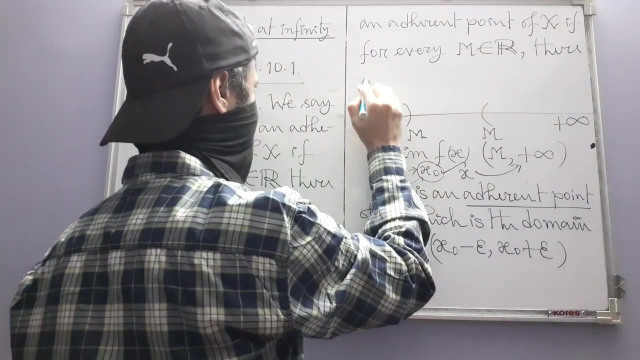 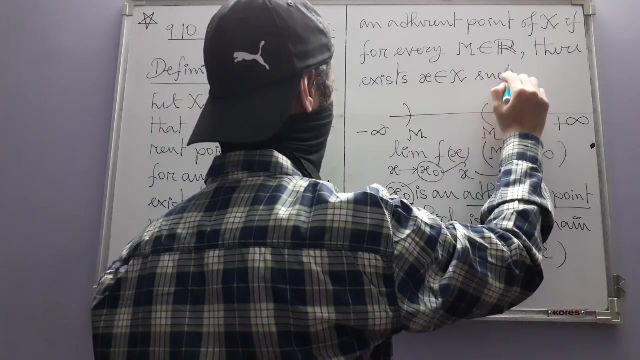 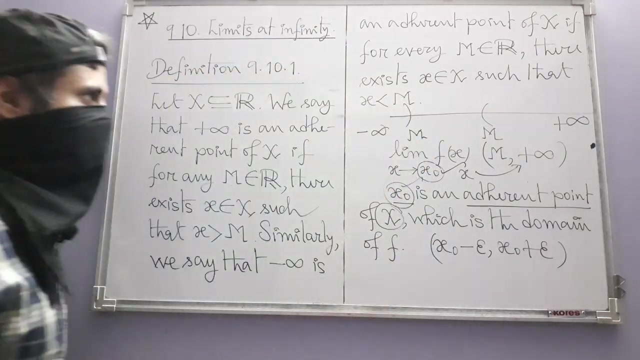 belonging to x. this m has nothing to do with this m. okay, it's another definition. technically speaking, it's another definition. for every m belonging to r, there exists an element x in x, such that x this time is less than m. okay, so this is the definition of. 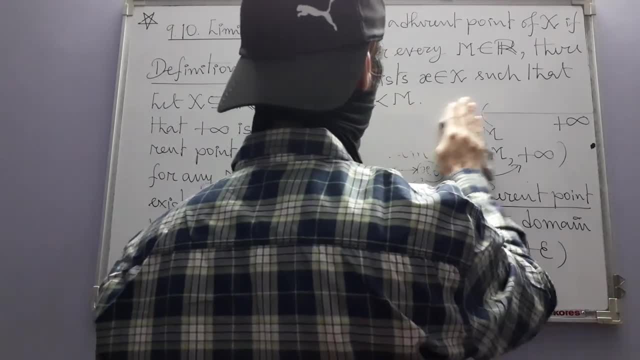 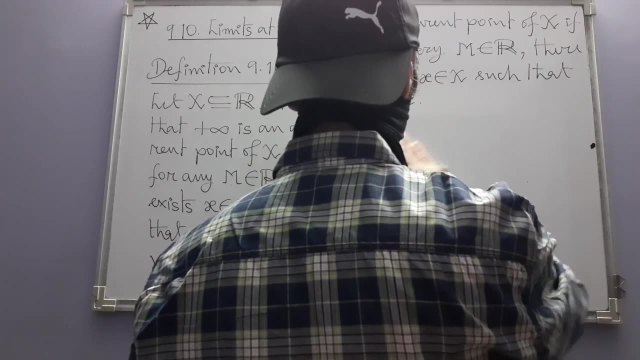 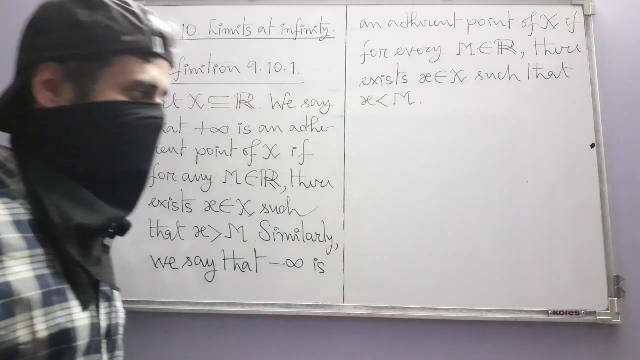 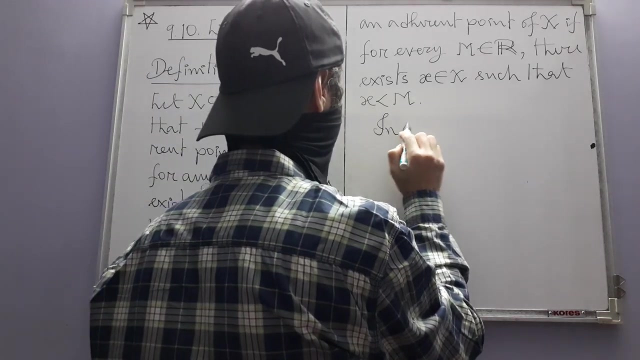 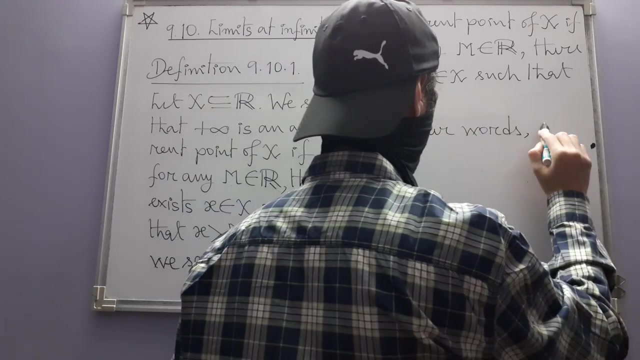 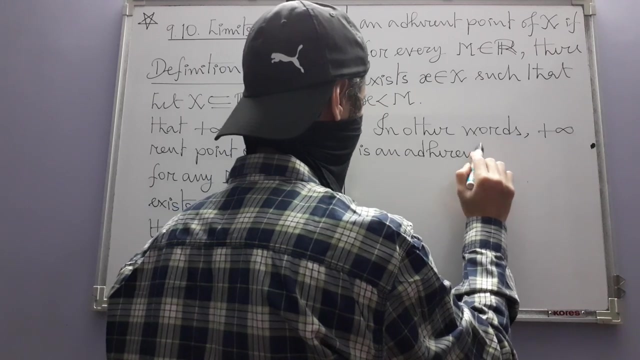 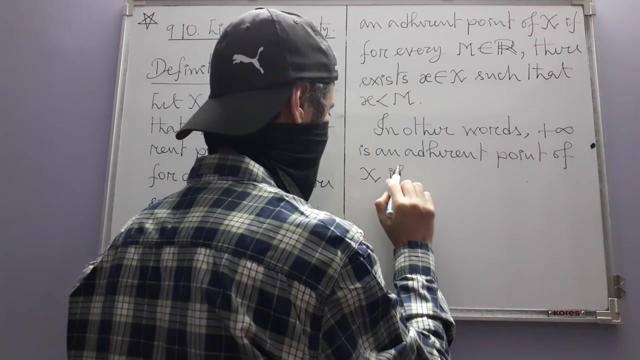 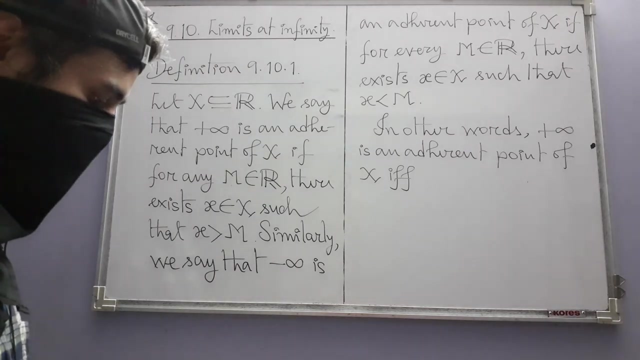 plus and minus infinity being adherent points of a set x of real numbers, so you can understand that the definition implies these things. in other words, plus infinity is an adherent point of x if, and only if. that, of course we denote by i double f, if, and only if, x has 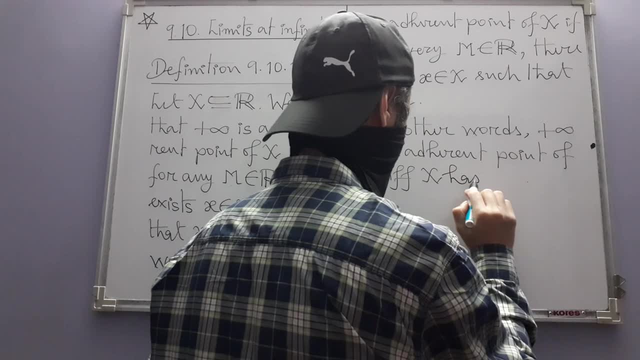 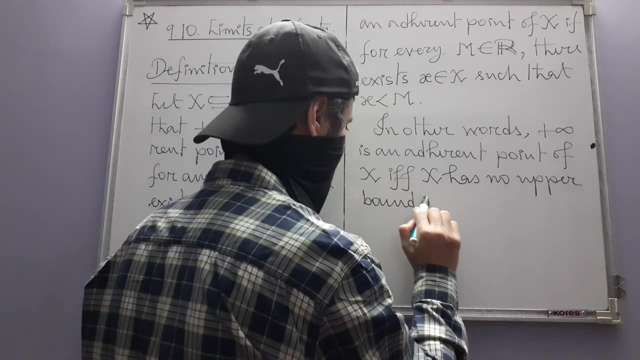 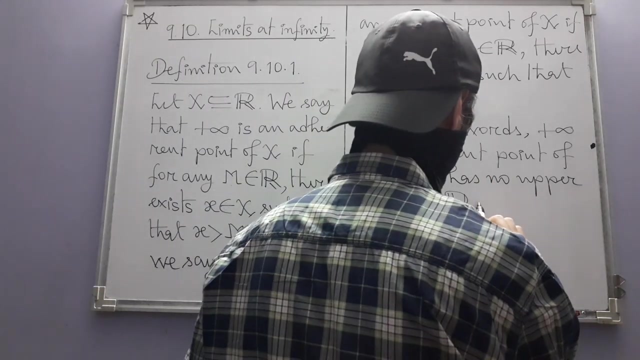 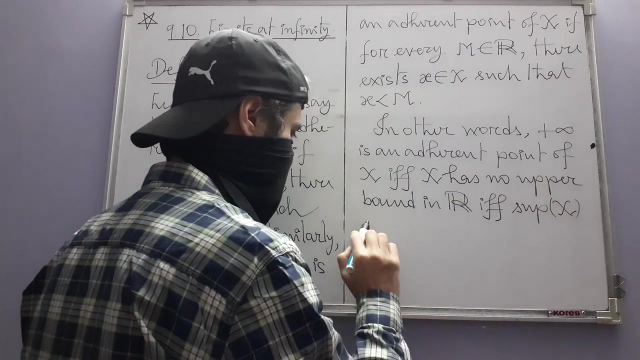 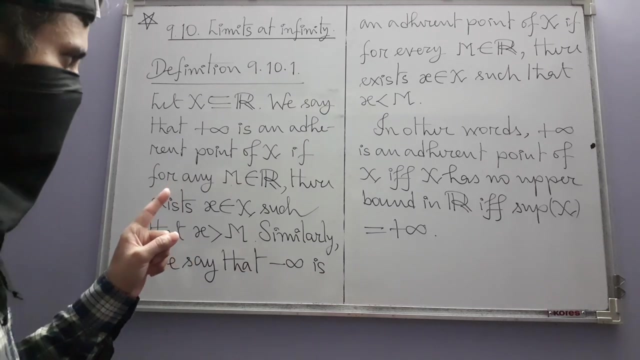 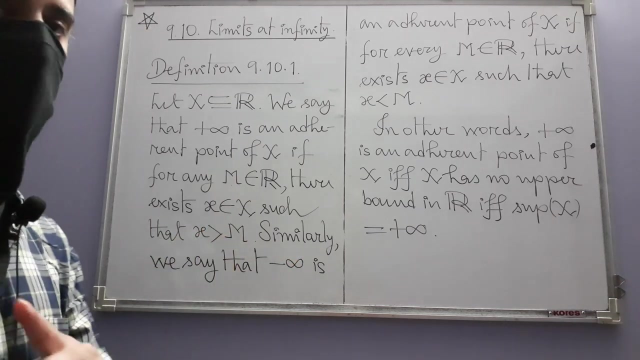 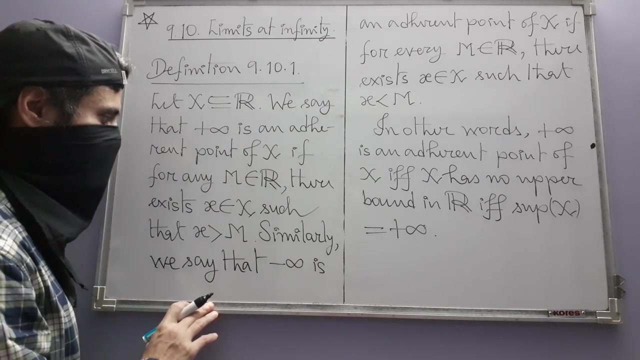 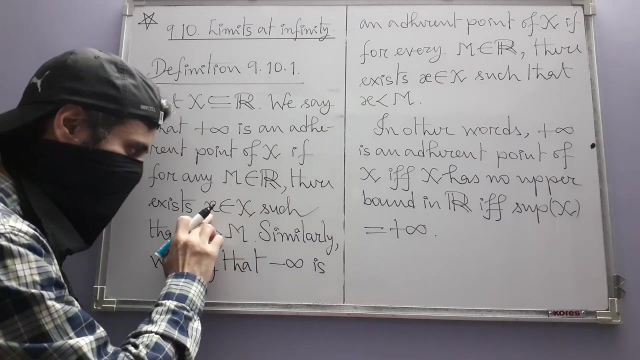 no lover bound in r. that, in turn, is equivalent to this if, and only if. Note one thing carefully: that this definition implies that x is non-empty, although that we have not said anything. Why does it imply that x is non-empty? Because if x is empty, then for any m, then for no m you will find such an x in x satisfying this condition, let alone for all m. 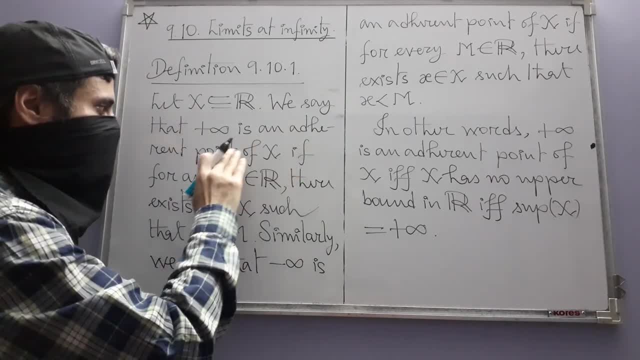 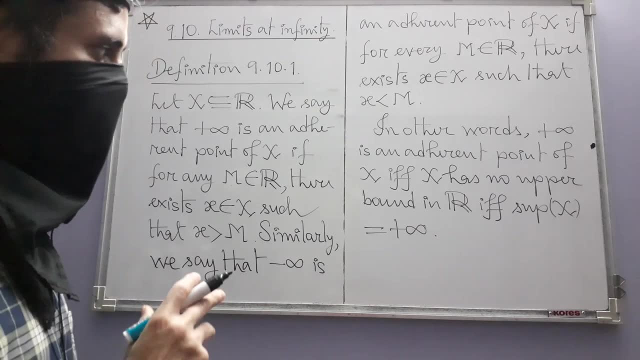 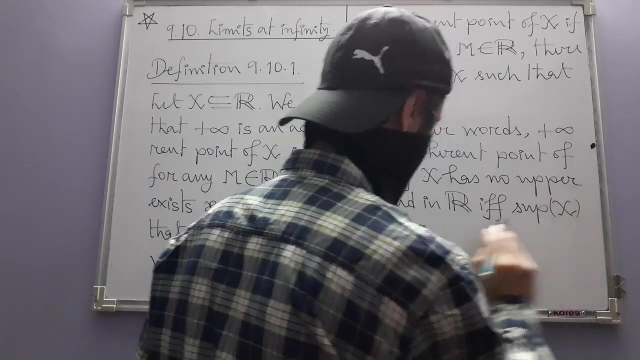 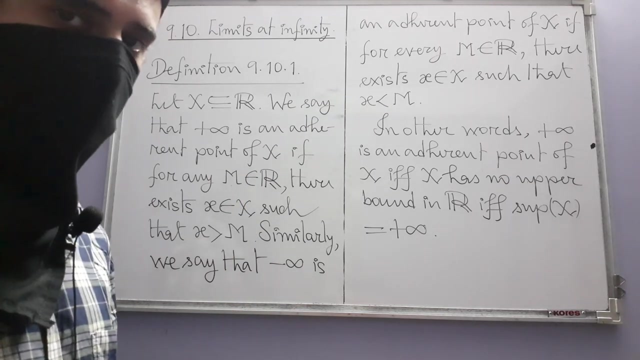 That is why if plus infinity is an adherent point of x, then x necessarily is non-empty. Now why am I bringing this non-emptiness? That is because for a non-empty set the supremum is plus infinity. For the empty set, the supremum, by definition is minus infinity. So that problem is not present here. 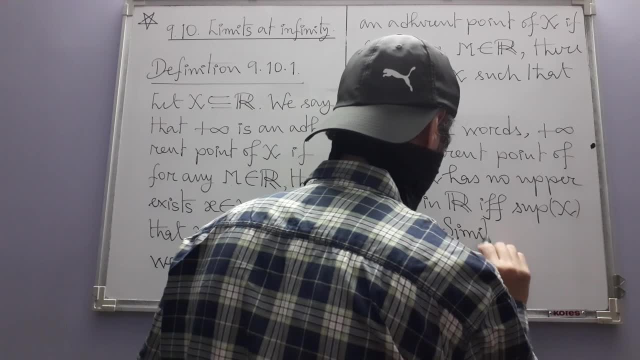 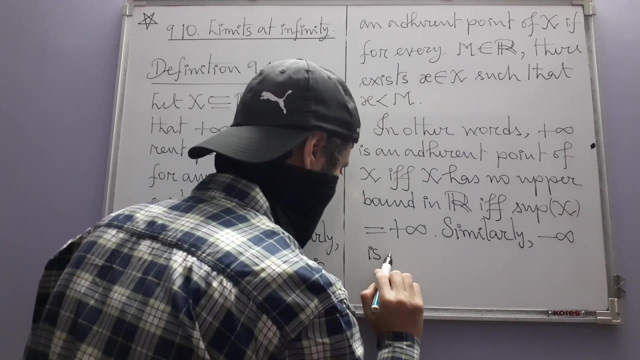 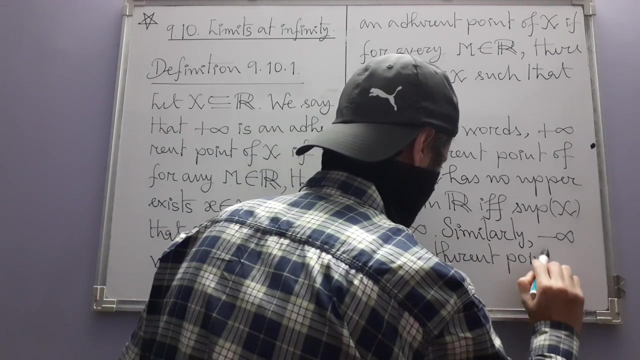 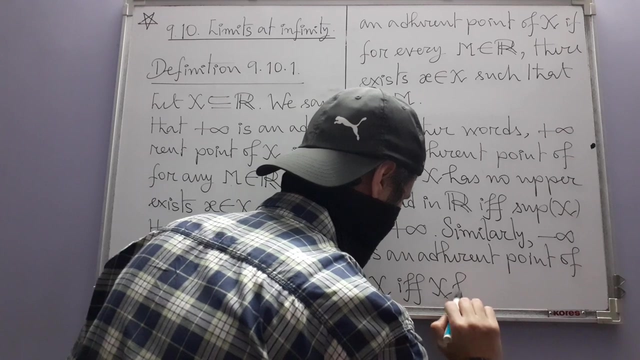 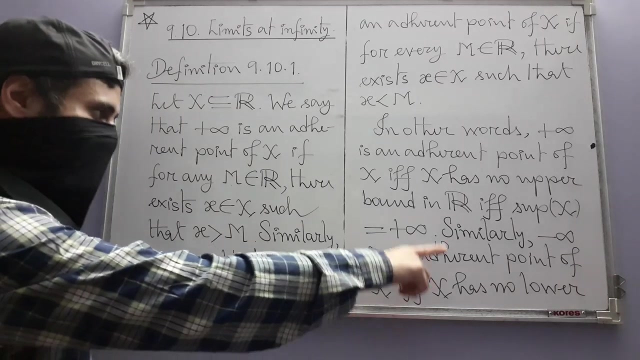 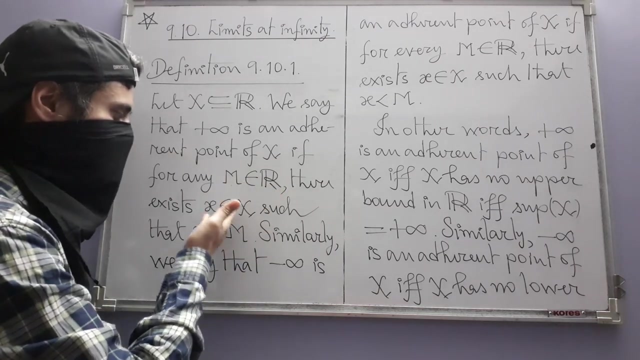 Similarly, similarly, minus infinity, is an adherent point of x if, and only if, x has no lower bound, Lower bound, So that this first if and only if, is immediately clear from the definition, because this is precisely the case in which x is failing to have an upper bound in R. 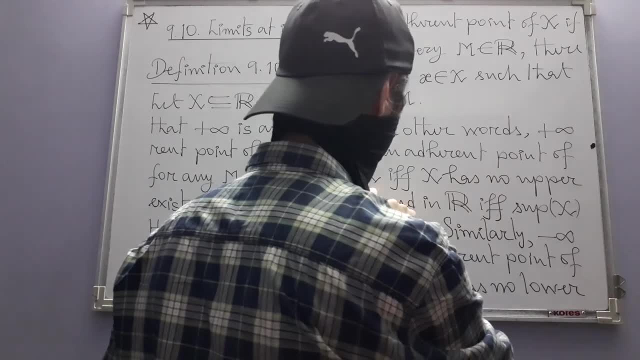 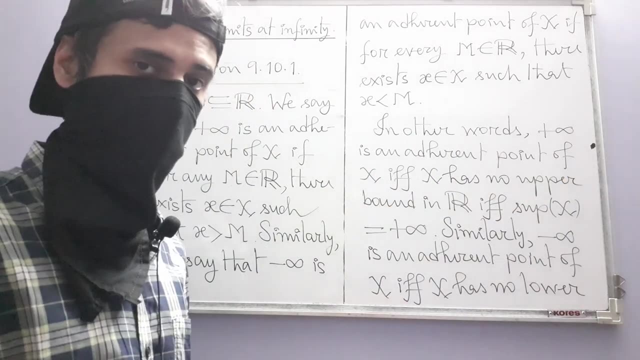 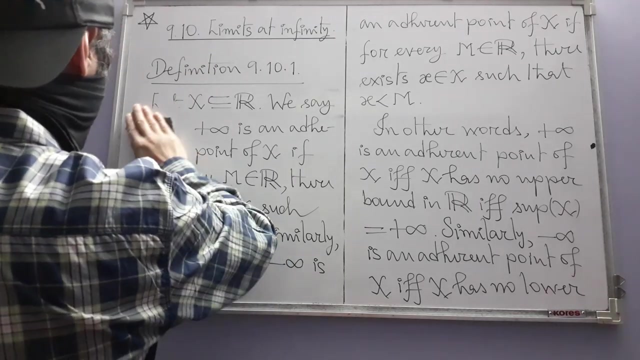 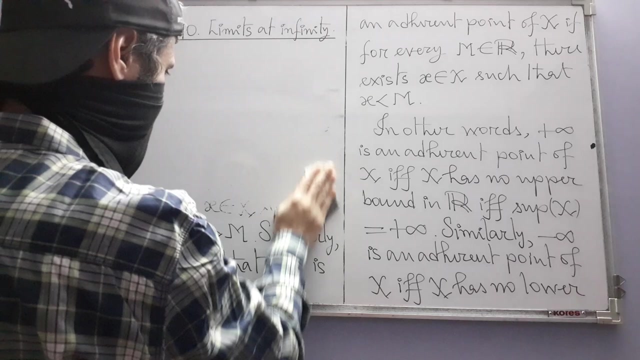 In R. I say because plus infinity is always an upper bound for any non-empty set of real numbers in the extended real number system. And the second if, and only if, is also clear because in that case, precisely because x is non-empty, the supremum is plus infinity. 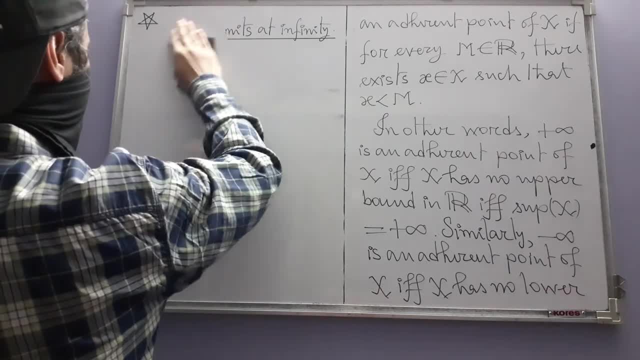 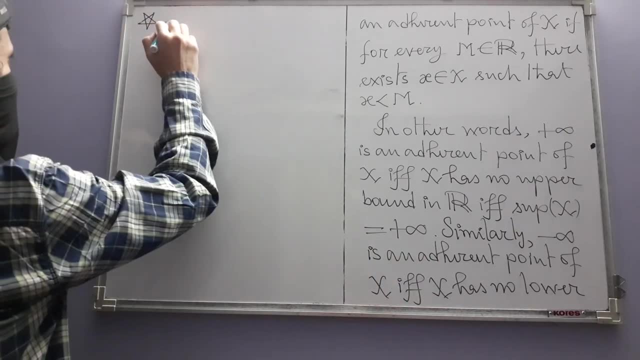 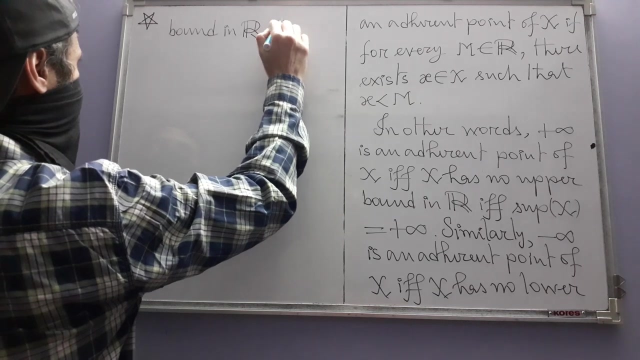 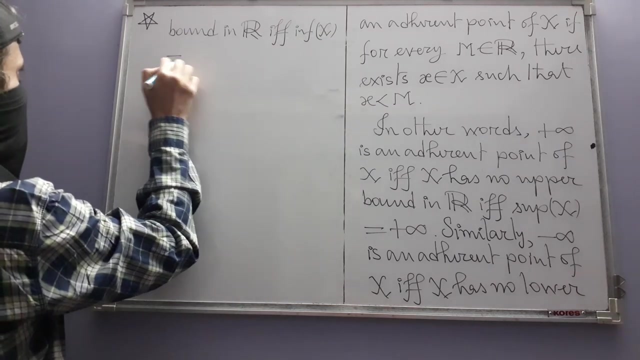 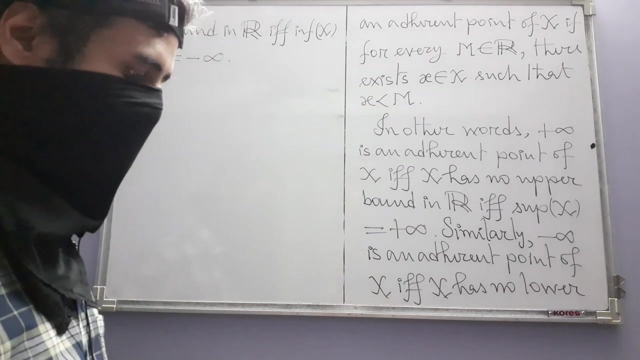 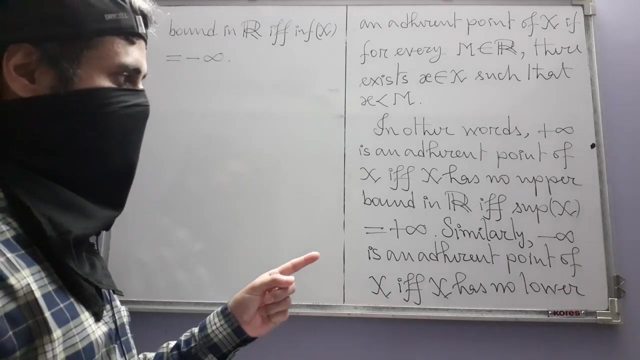 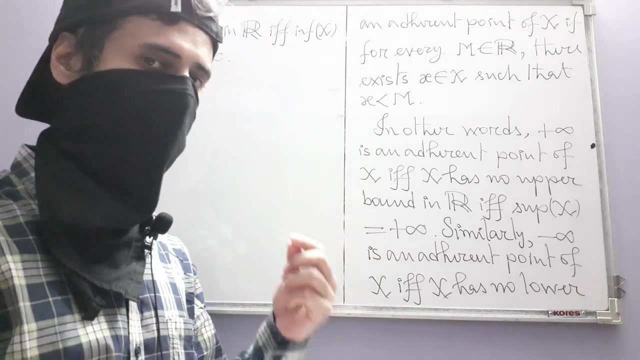 Similarly, minus infinity is an adherent point of x if, and only if x has no lower bound in R, if and only if x has no lower bound in R. But here let us adopt a, Let us adopt a remark, So this is the remark. 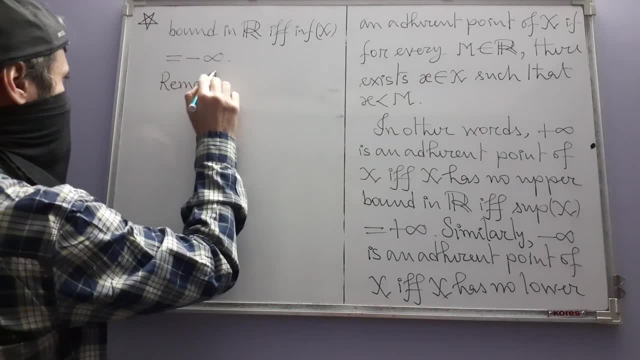 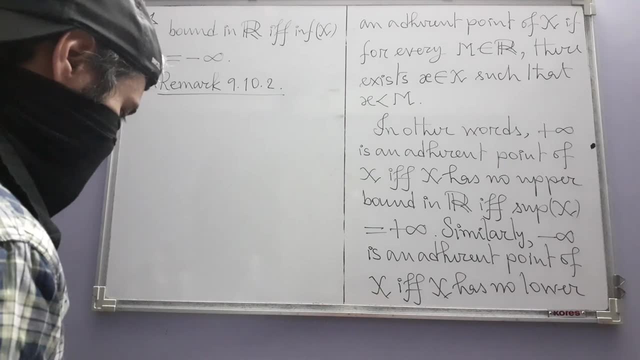 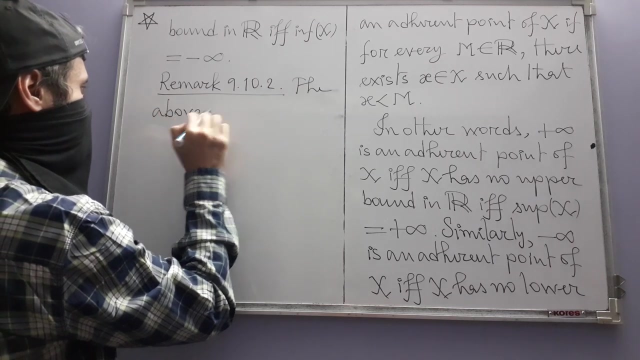 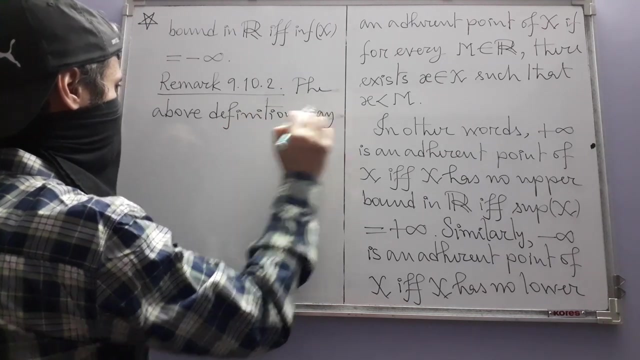 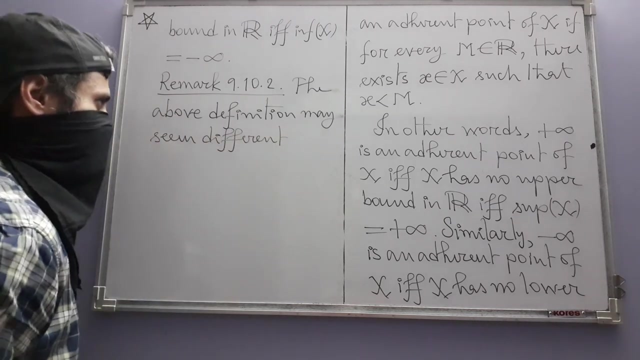 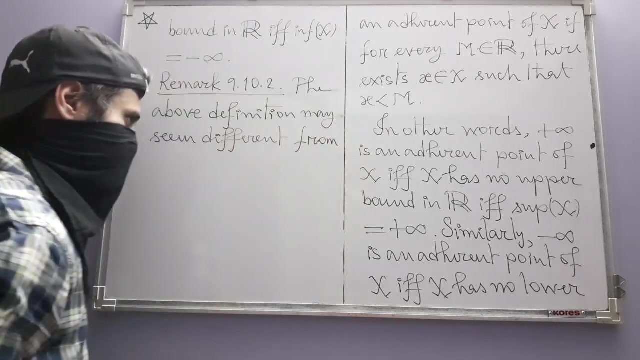 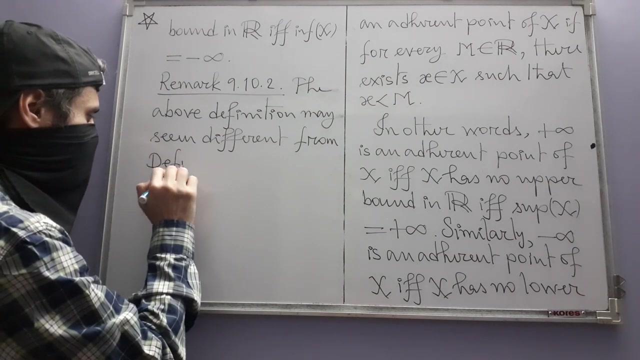 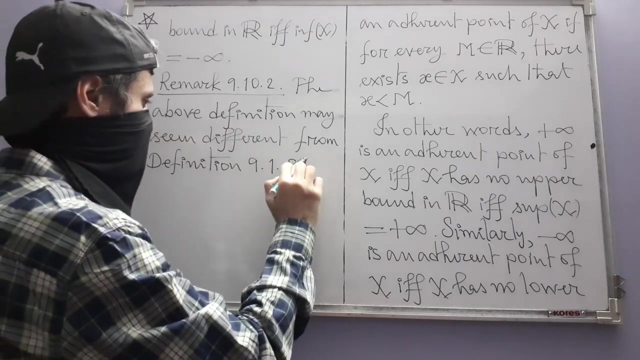 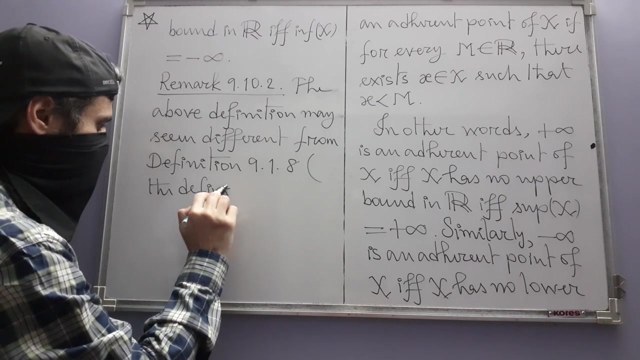 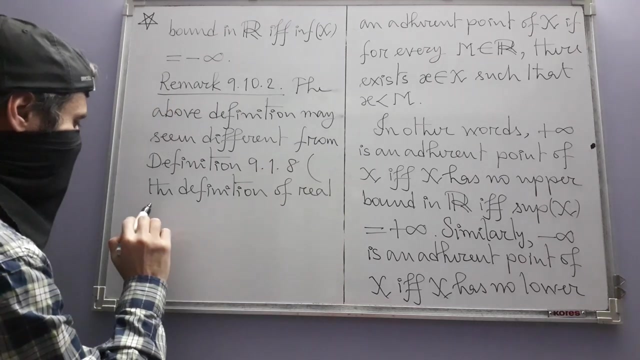 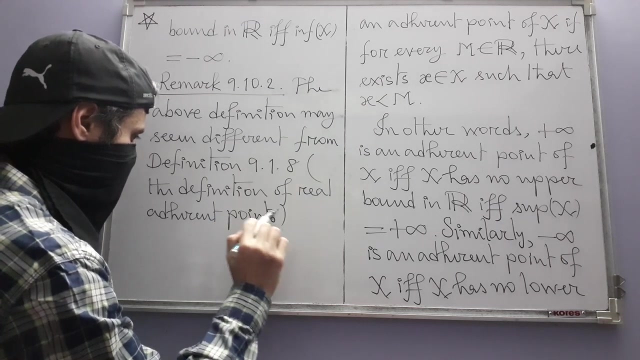 So this is the remark remark. The remark just tells us this: the above definition may seem different, rather different, actually the author writes: may seem different from the original definition of adherent patent, that is definition 918.. The definition of, let me write like this: real adherent points, so that we do not forget. 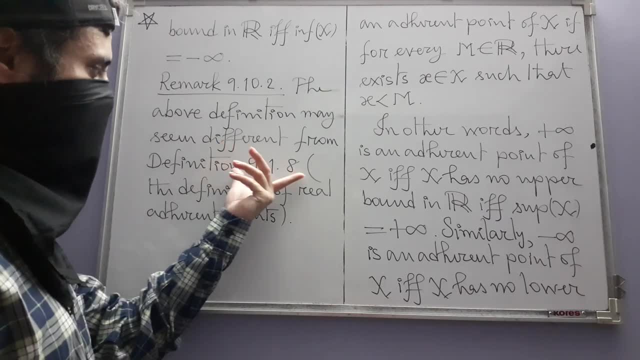 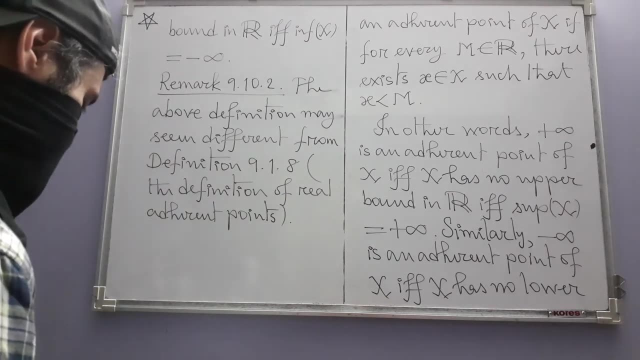 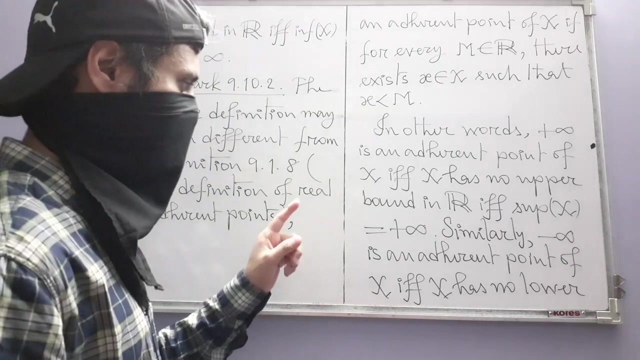 what this actually is. you need not go back and see what the definition is. I mean, you obviously remember- That is why we are writing like this- but can be unified Now. you see, it can be unified. I mean actually. 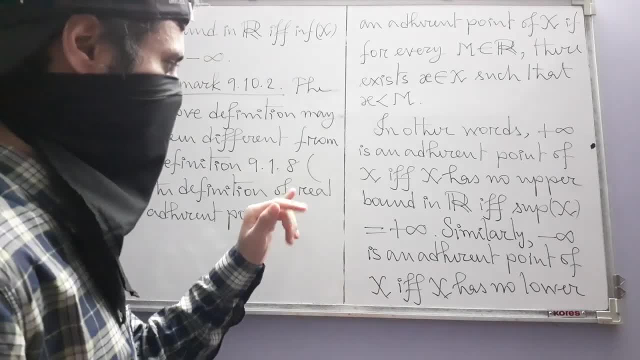 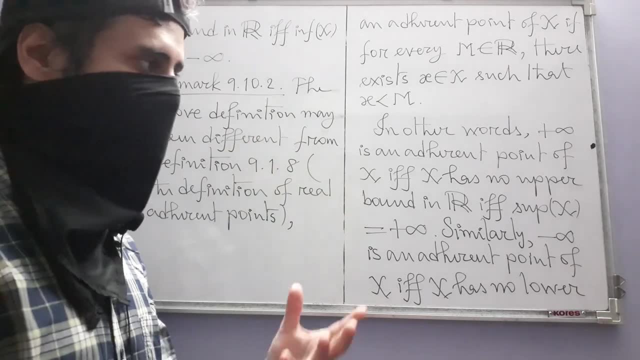 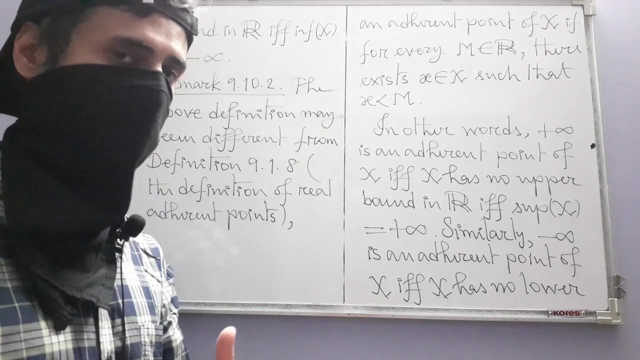 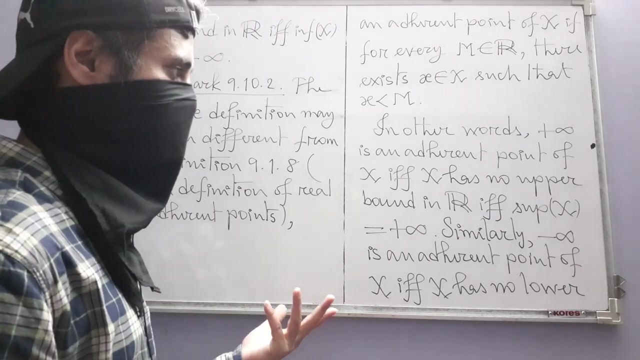 truly speaking, there is no distinction between this new definition that we have seen just now and the old definition, provided we think of the extended real number system. using the topological structure of that extended system, You will be able to see that the two definitions 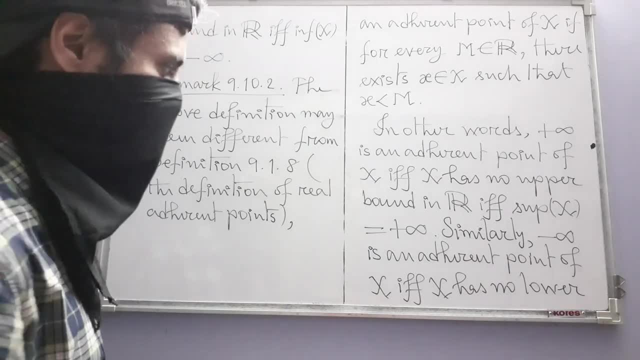 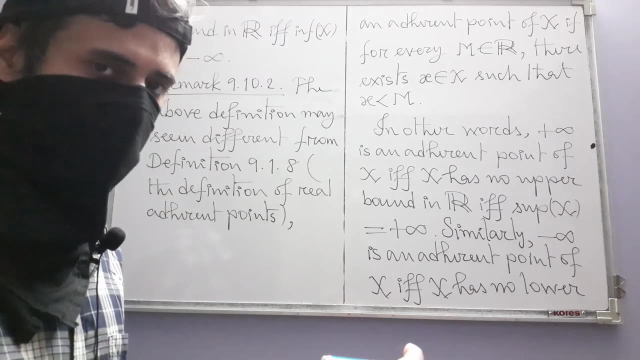 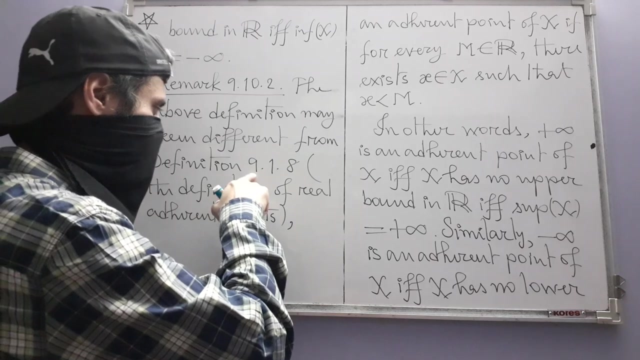 are in fact the same thing Here only we have the points which we want to call adherent points as plus or minus infinity, the smallest and largest elements in that extended system respectively. And in the old definition we just have a real number. 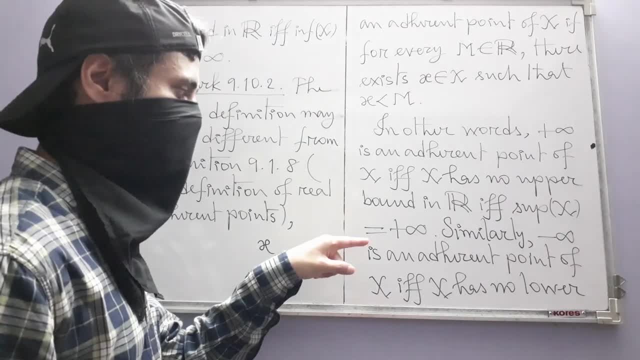 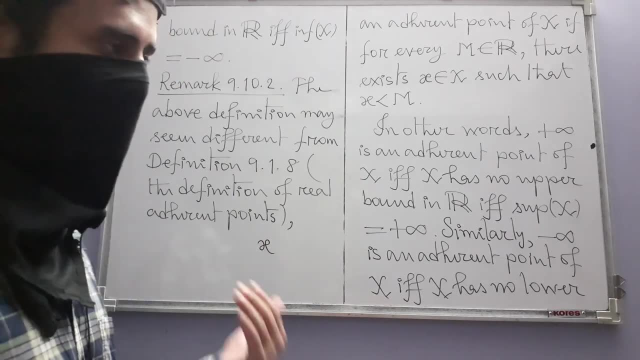 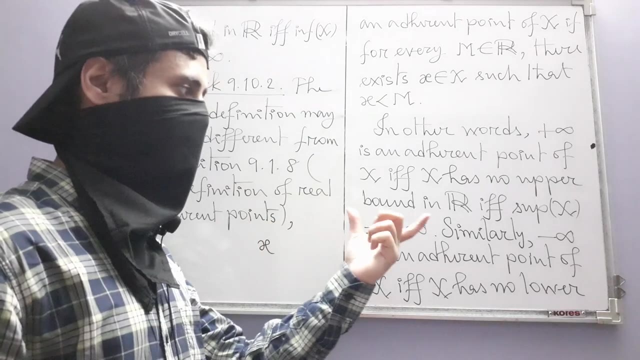 So the point here is that these new adherent points are also extended real numbers and actual real numbers are also extended real numbers And using the topological structure. we say, or the author says, using the topological structure because that idea of neighborhood. 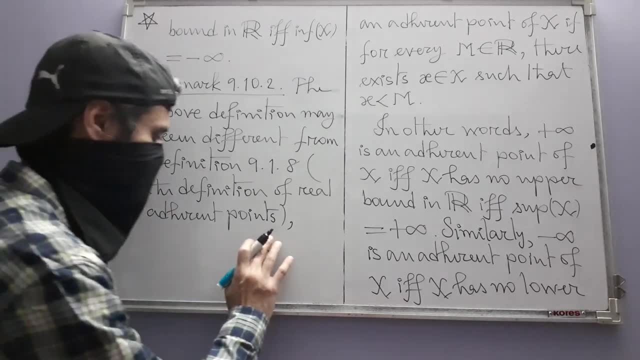 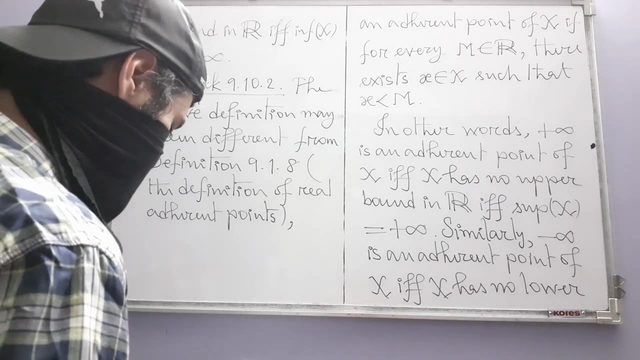 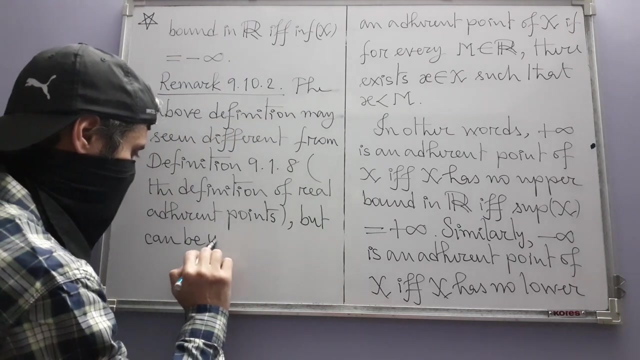 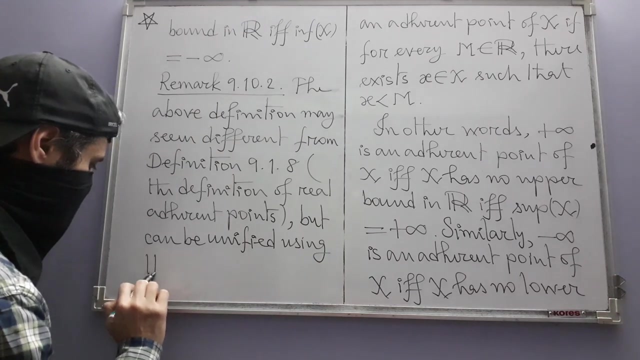 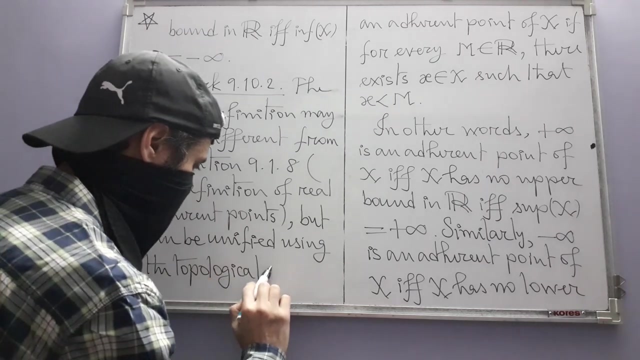 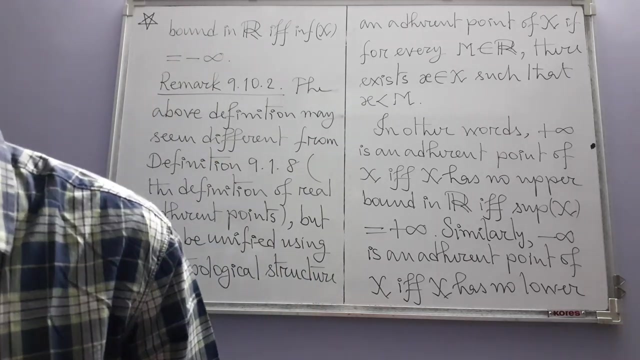 comes up. That's why. But we won't do this. There is no need to see that these two things are the same. So what does tau say? What can be unified? Yeah, But can be unified using the topological structure of the extended real number system. 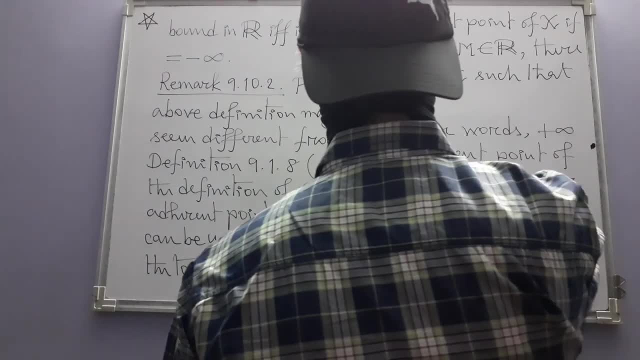 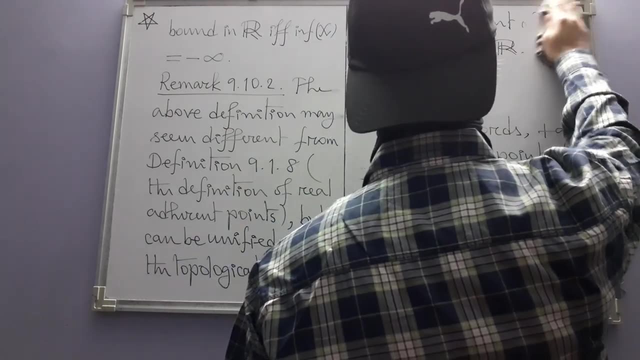 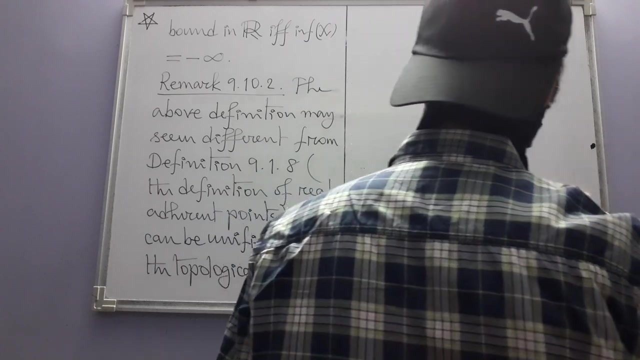 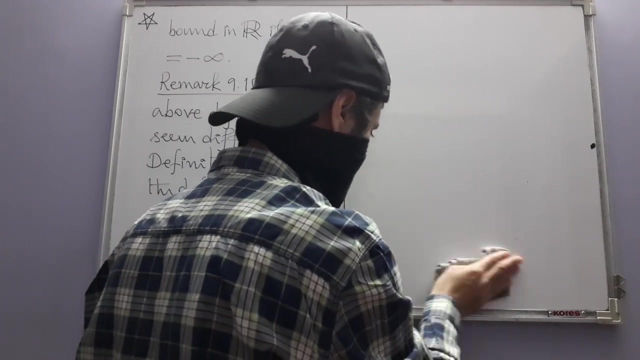 Okay, Okay, Okay, Okay. Let's start. When you view things in light of topology, many things which may seem like totally unrelated actually become the same thing, Just different aspects of the same thing. However, at this elemental range, you can also study that the elements are totally unrelated. So you 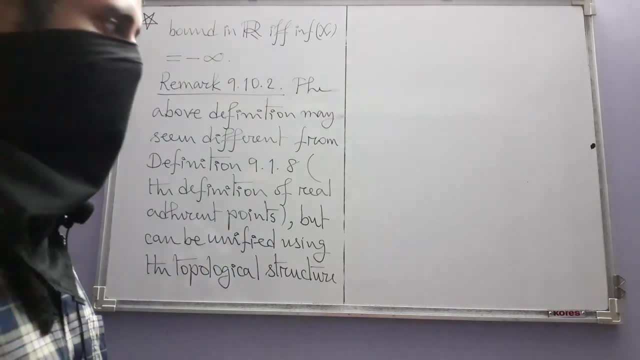 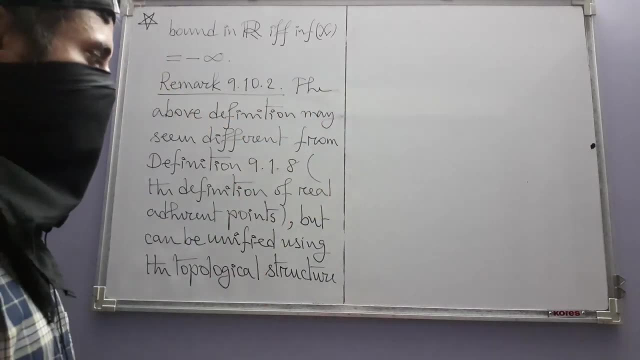 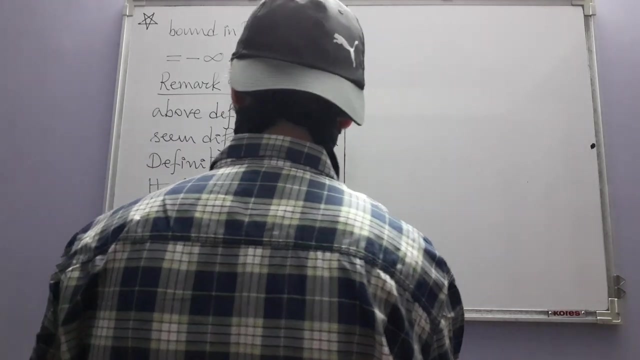 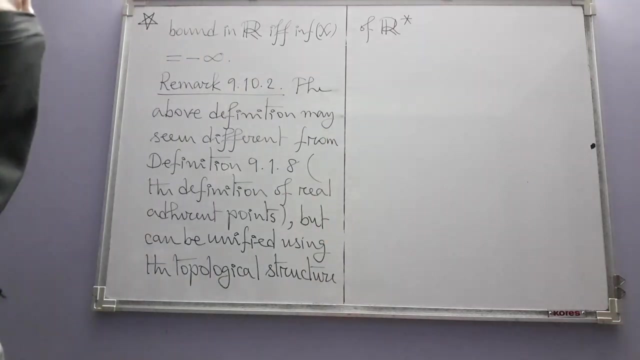 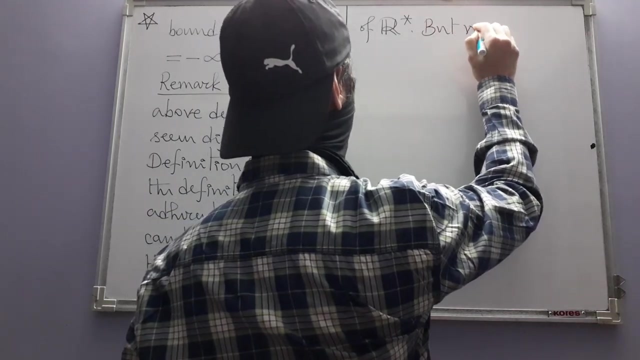 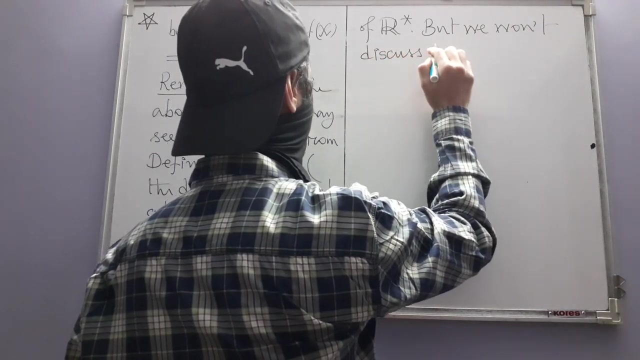 elementary stage, we need not bother too much about topology. we still have time to see why that is important and, moreover, we haven't yet seen the notion of topology itself formally okay, so let's just forget about those things of r star, but we won't do so, yeah. 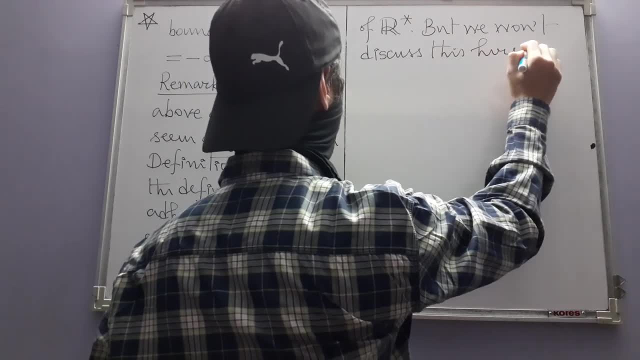 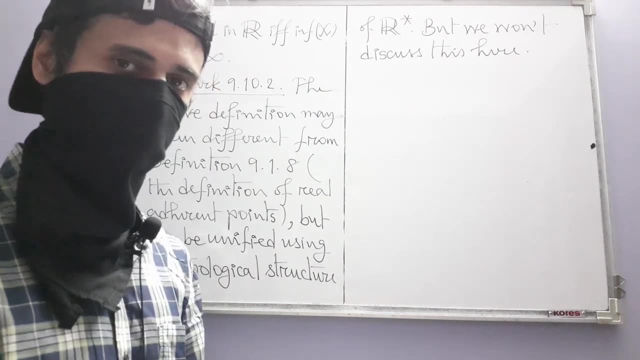 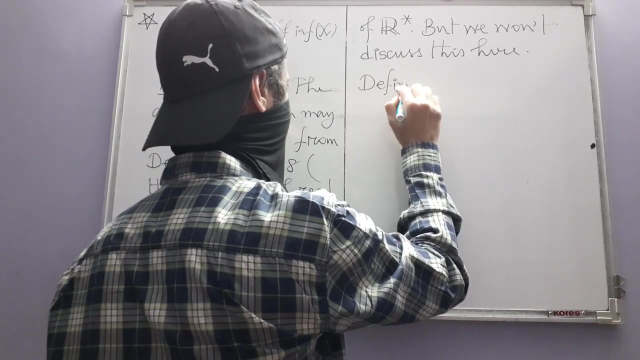 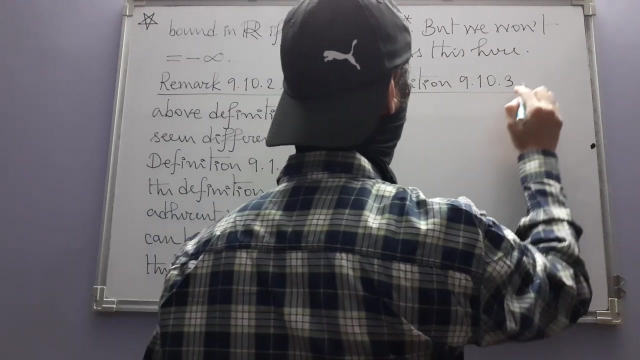 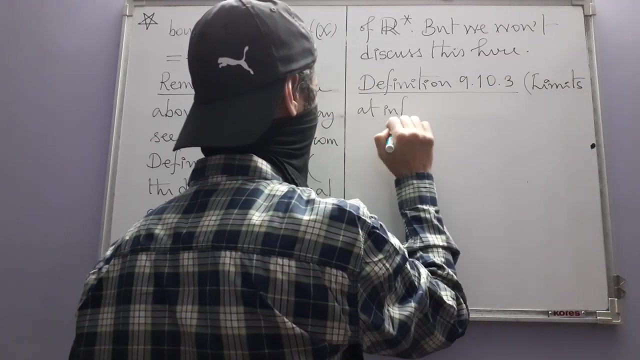 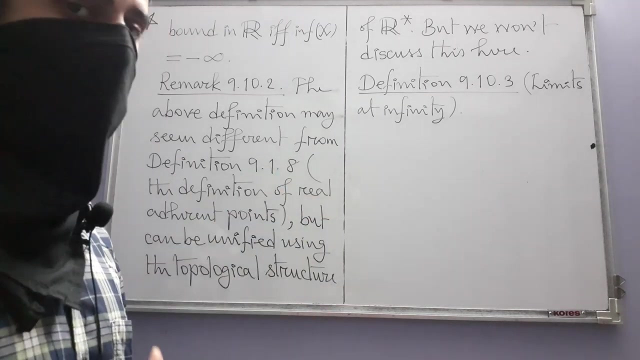 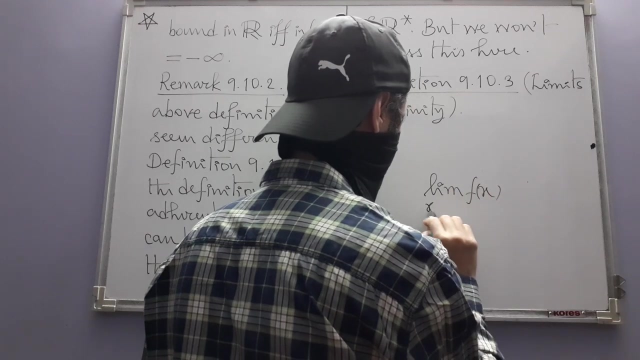 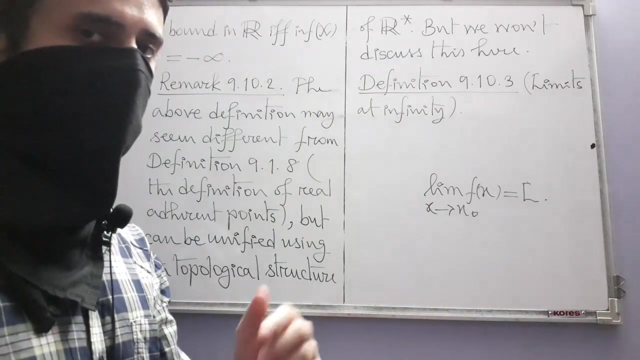 we won't discuss this here, okay, this is not the right time for that. and now we come to our actual definition: limits that infinity, limits at infinity, not infinite limits. limits at infinity- limits at infinity- okay, limits at infinity. so our x naught in this equation, in this familiar equation, our x naught is going to be either plus infinity or minus infinity, not 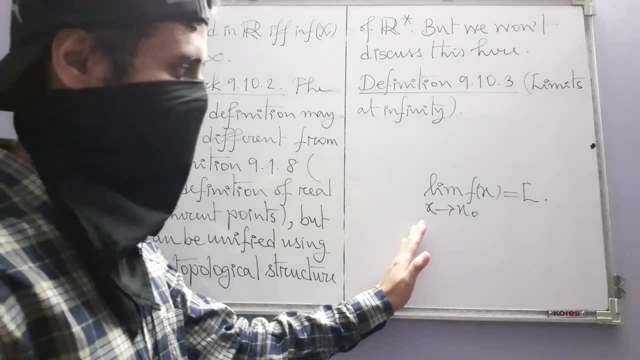 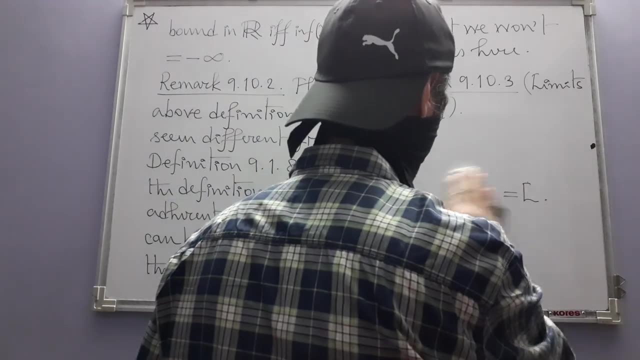 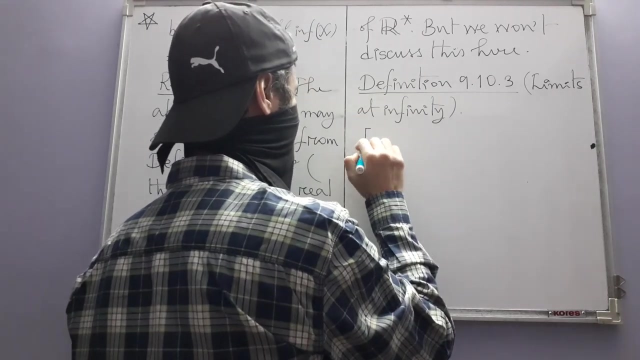 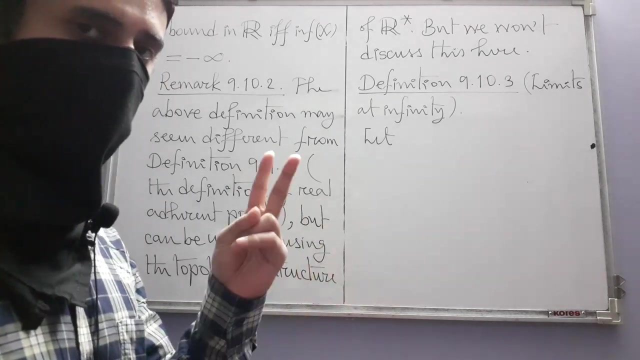 the l, that l also can be made plus or minus infinity. that is a different thing altogether. we won't need that here, okay? so the definition of curves starts like this: let, so you can imagine that actually we are going to write conditions for two definitions, depending on whether x naught is plus infinity or minus infinity. 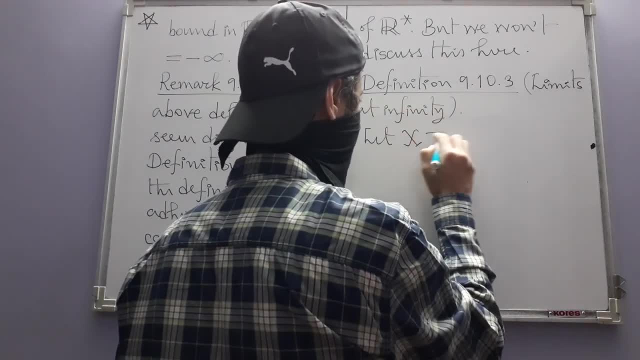 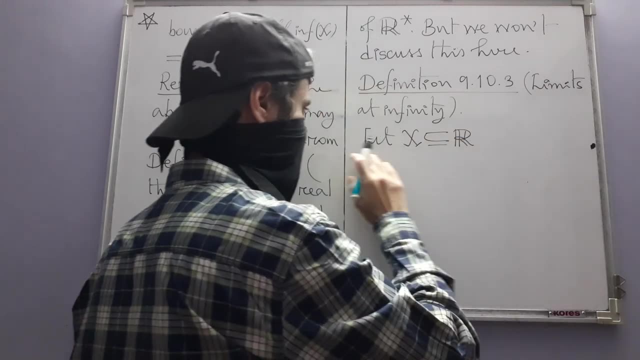 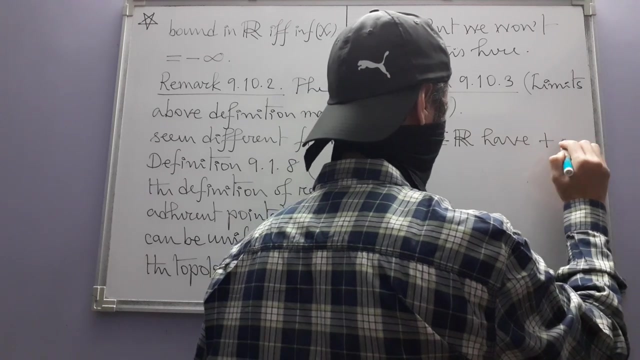 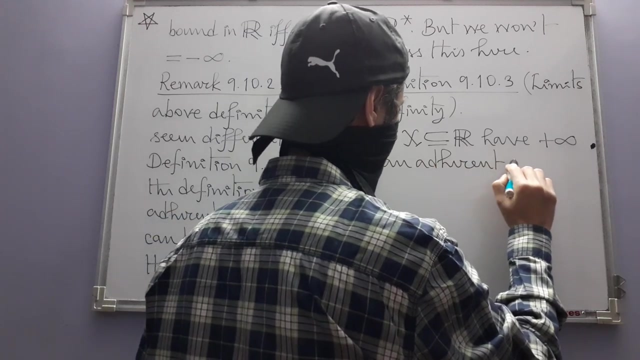 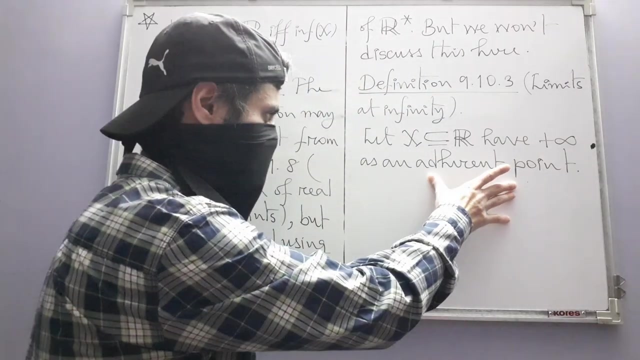 let x be a subset of r and let x, let. let us continue like this. Let x, which is a subset of r, have plus infinity as an adherent point. But before I write something else, let me also draw your attention to another thing. Had these two. 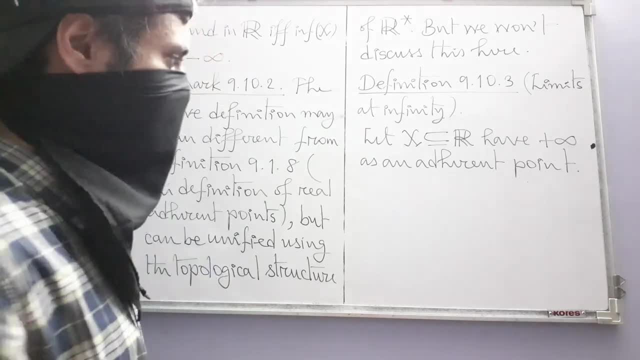 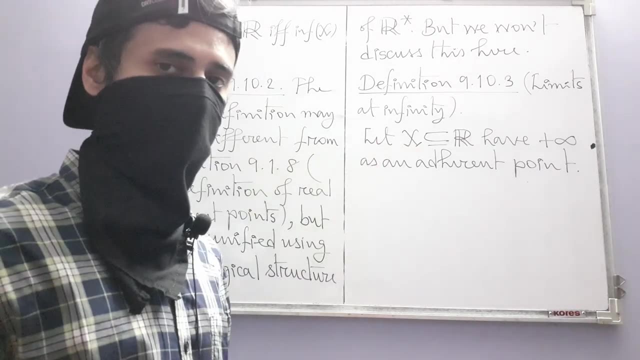 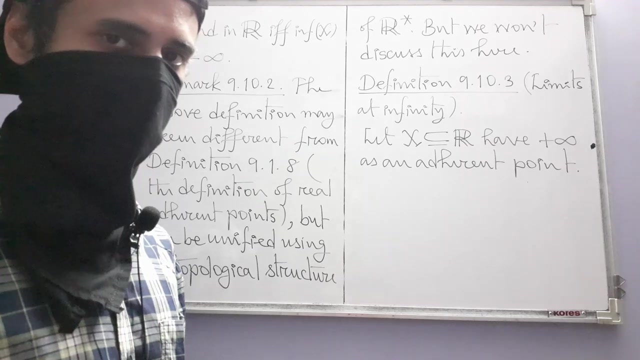 definitions been entirely unrelated and different. say, the old definition of adherent point and this new one have no relation at all between them, then there is no reason for calling these new points adherent point right. And that is why, because there is an underlying relation. that's why we 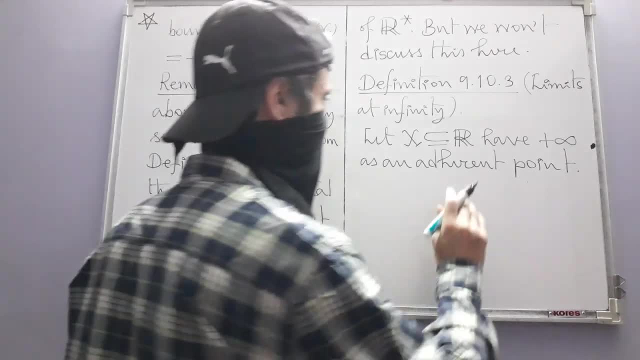 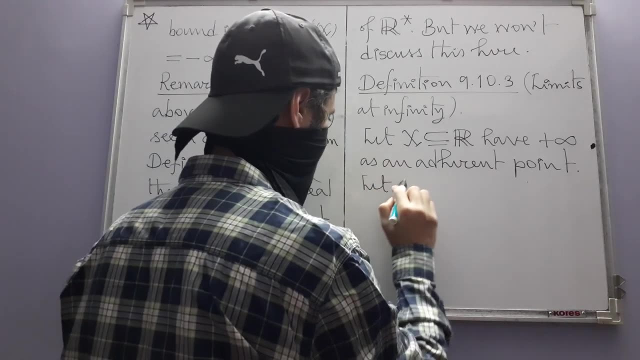 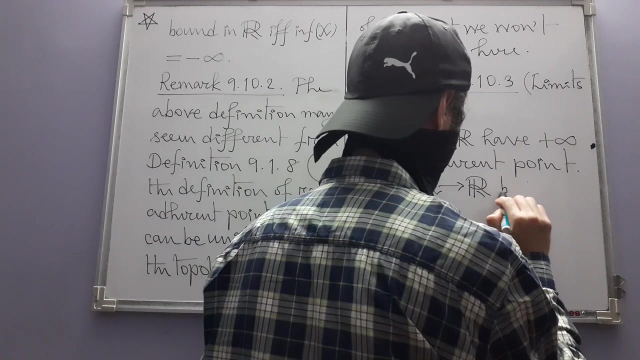 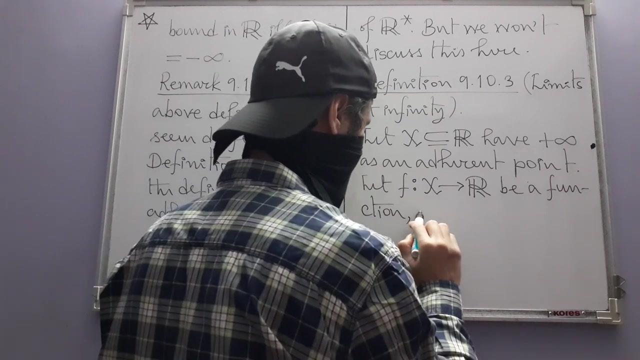 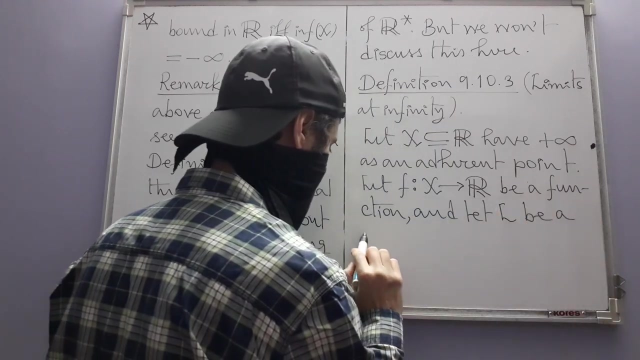 are calling them also adherent points. Okay, so now x has plus infinity as an adherent point. Let f from x into r be a function and let l be a real number. It's important that here l is a real number, not plus infinity. 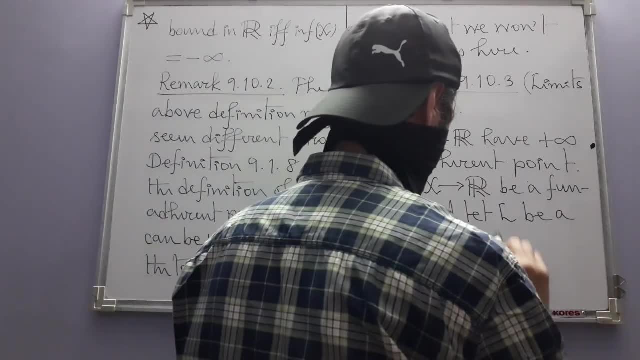 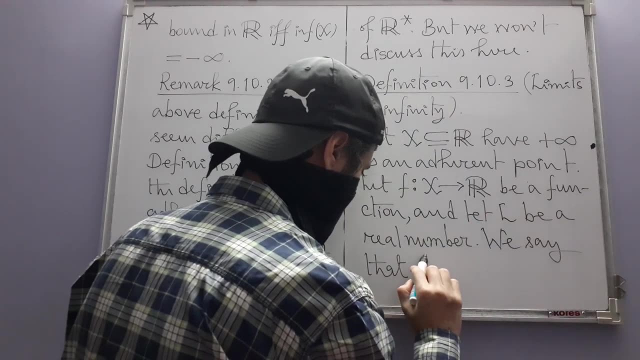 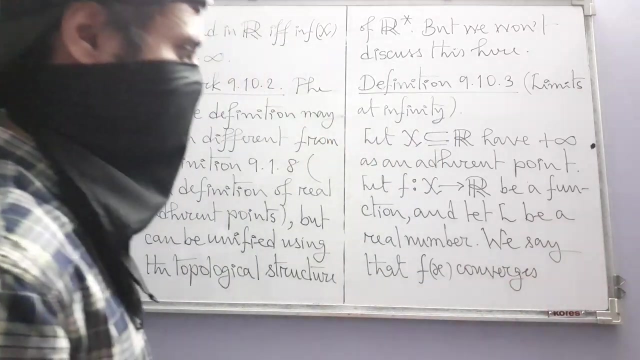 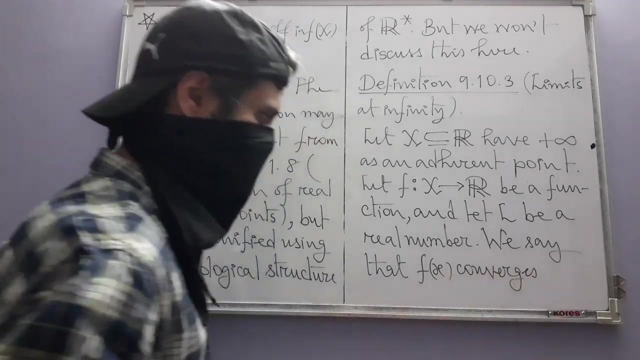 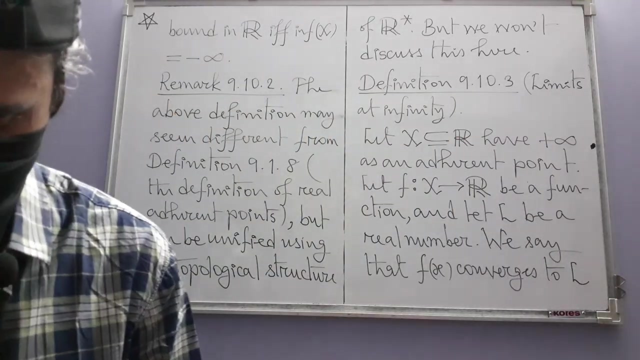 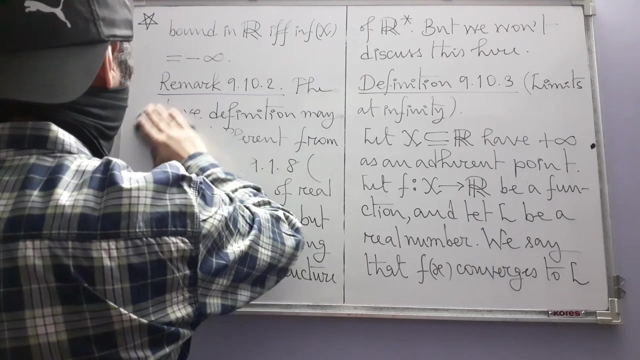 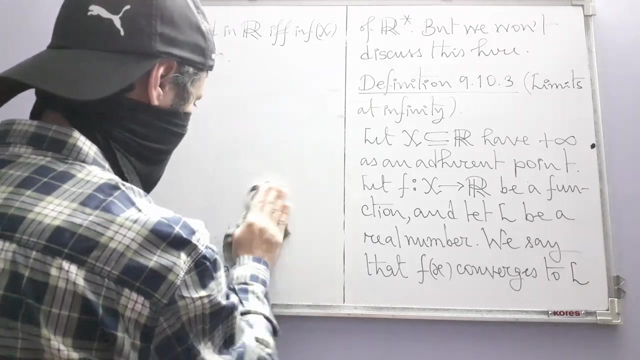 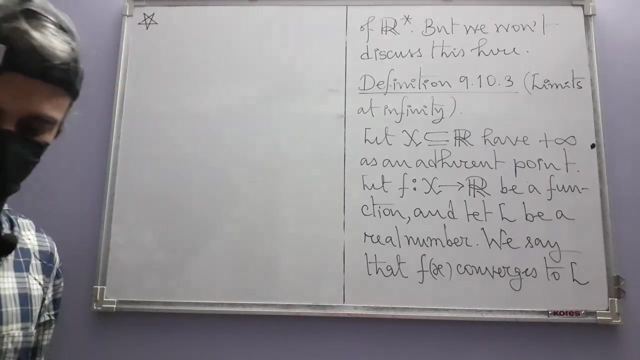 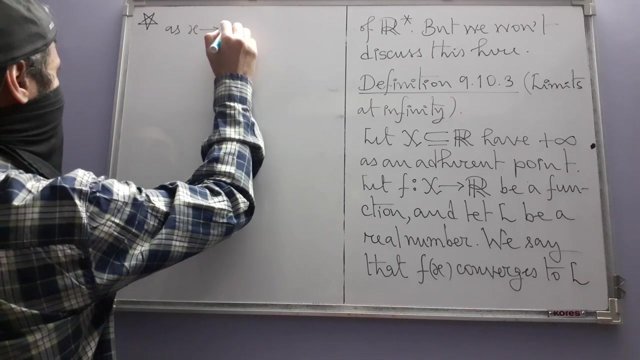 r minus infinity. That's what I was saying just now. We say that f? x convert. this is a very strange way of saying this thing, but the author for some reason decided to use this word. f? x converges to l as x tends to x naught. 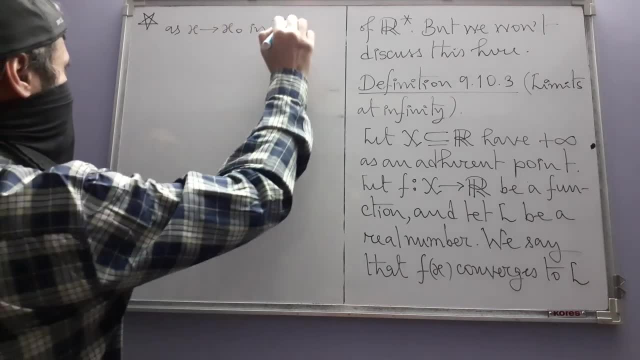 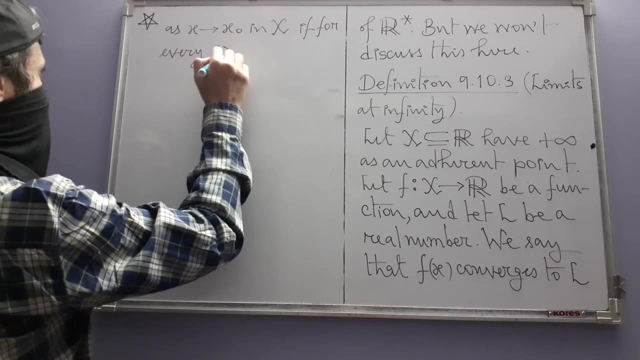 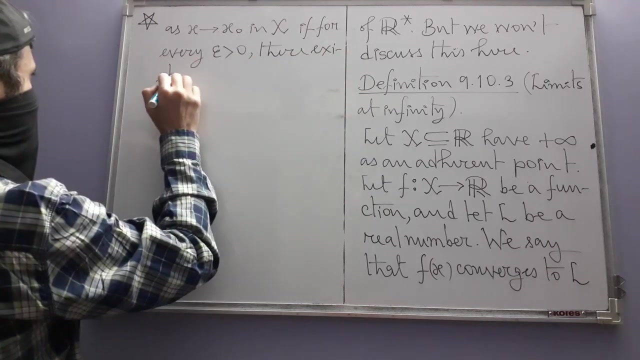 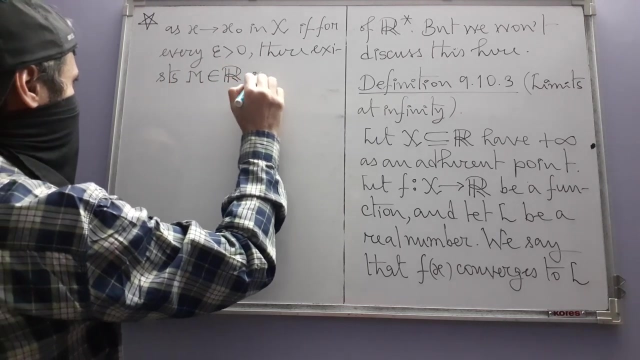 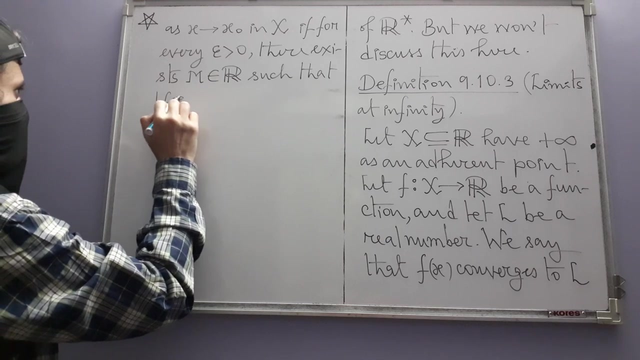 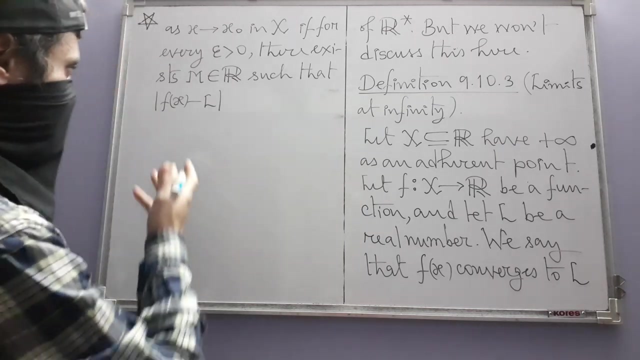 In x, if for every positive epsilon there exists a real number, m, such that if x is greater than m, then l is greater than m. Tau writes the next thing in words, but ultimately that just means this, such that what he writes is: 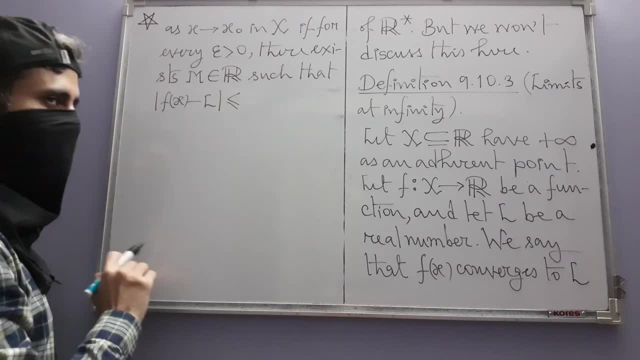 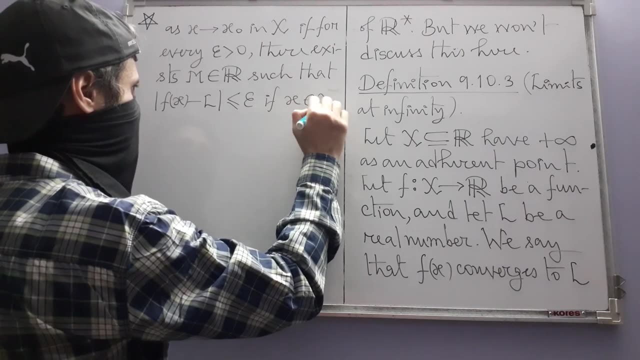 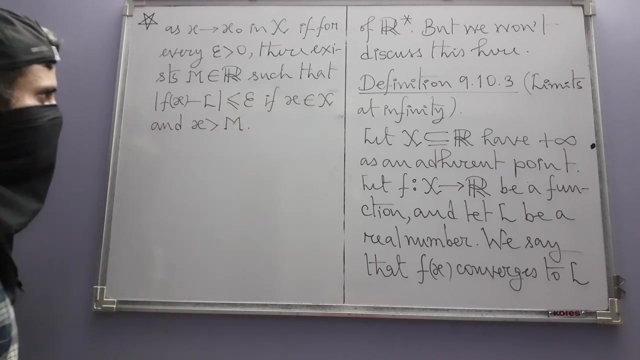 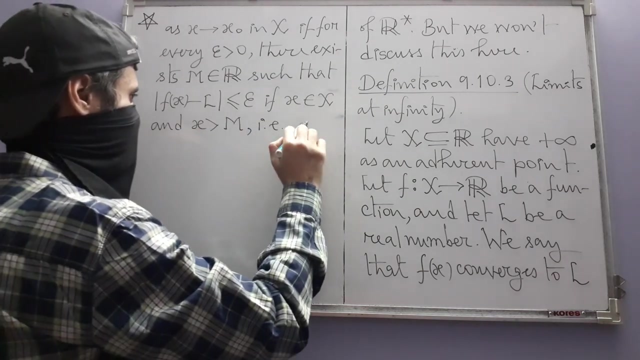 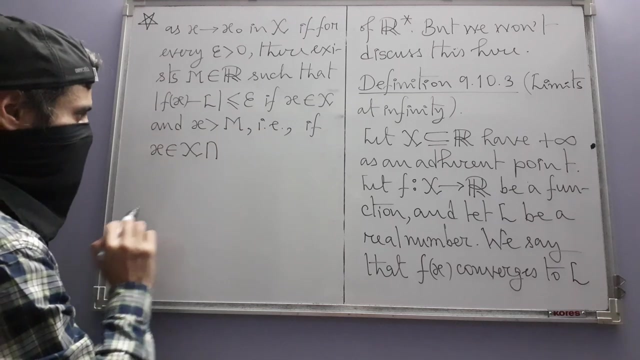 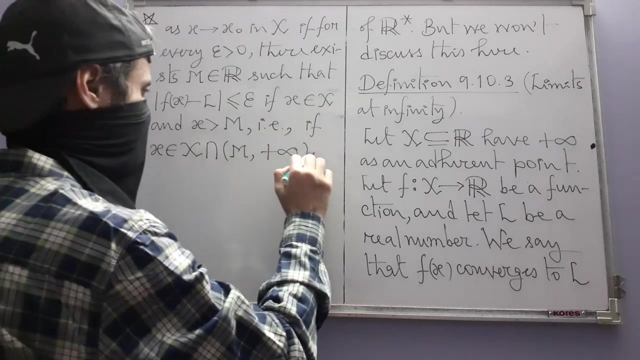 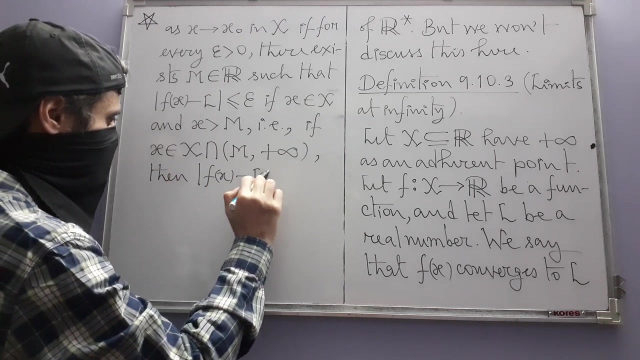 that, such that f- x is epsilon close to l. but that just means this: If x belongs to x and x is greater than m, That is I e. if x belonging to x intersection this open ray, then the distance between f, x and l is greater. 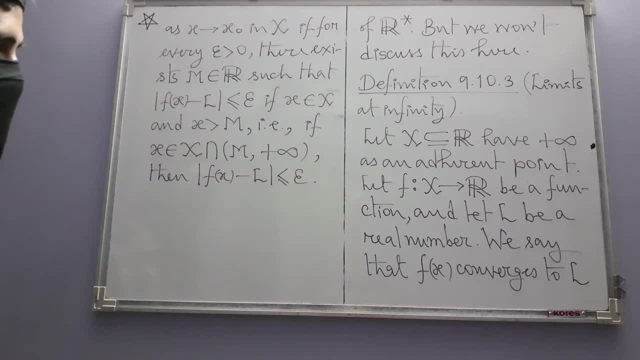 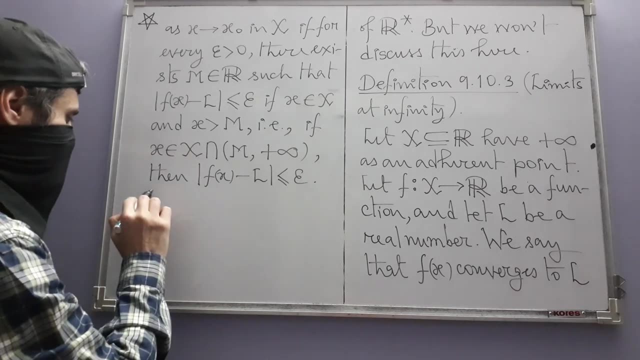 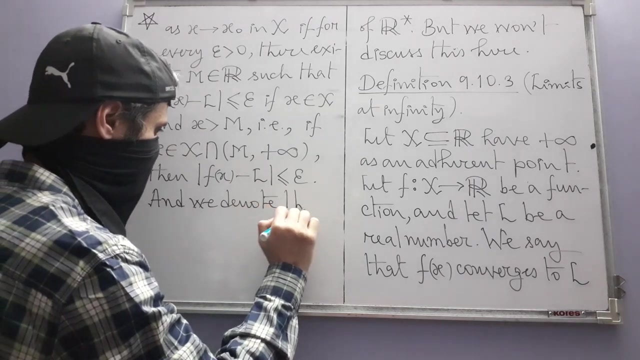 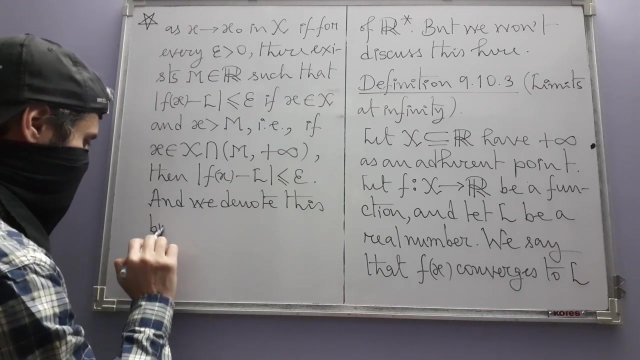 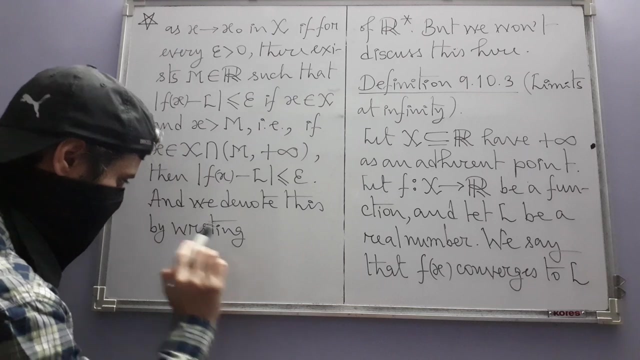 is at most epsilon. When this happens, then we say that f converges to L as x tends to x naught in x, and we denote this entire thing, we denote in symbols like this by writing this: Our usual notation, actually limit of f of x is L as x tends to plus infinity in. 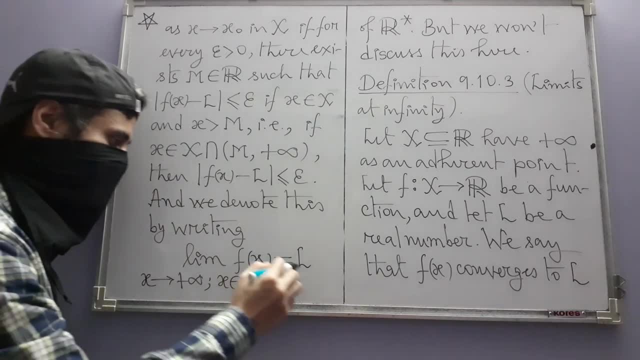 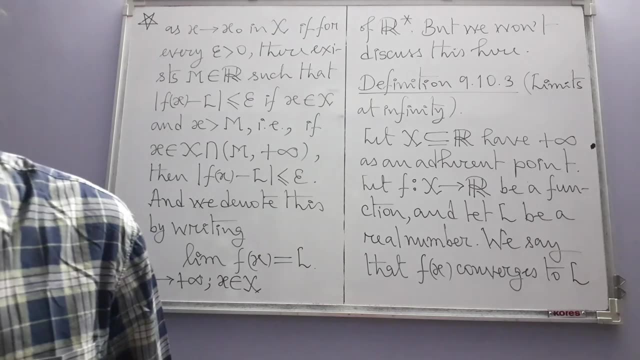 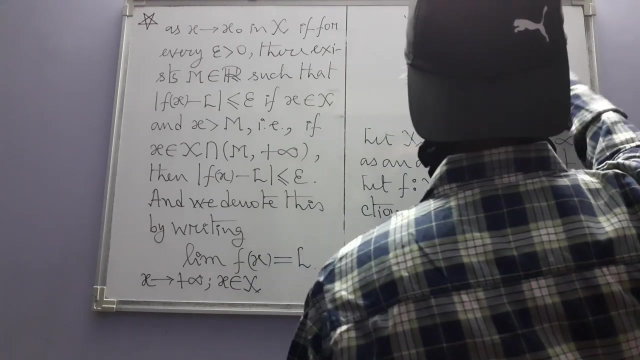 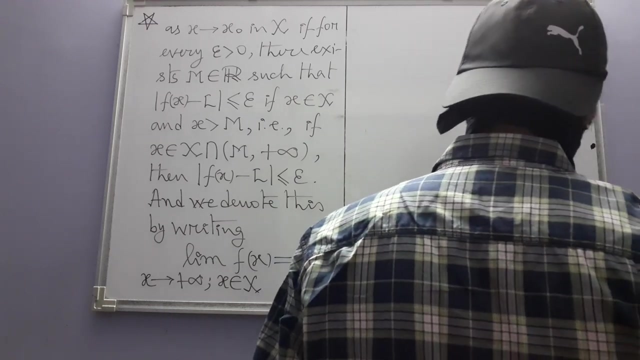 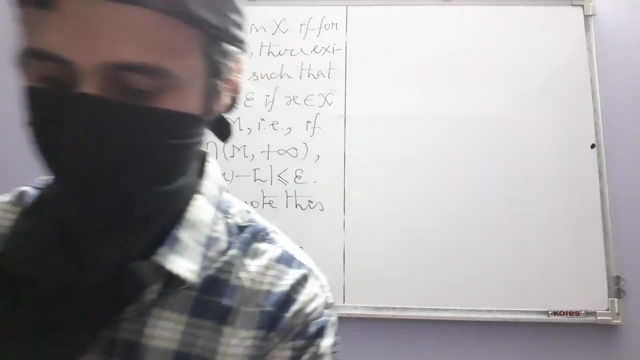 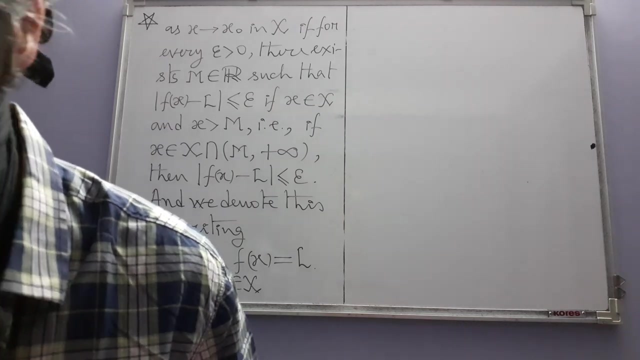 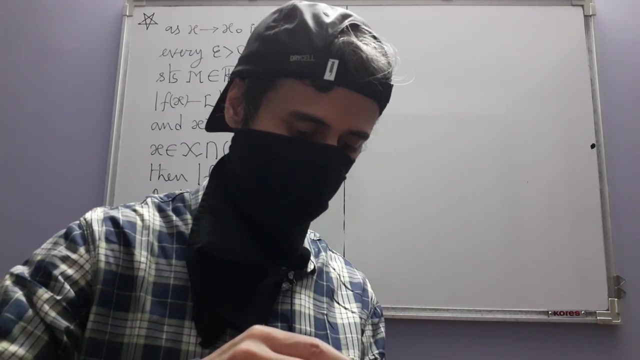 capital X. So this is the notation and this is only one half. So now we are going to also define limit of f at minus infinity. I think I need a little ink. The weather is extremely dry. Even if I do this before starting the video, it just dries. 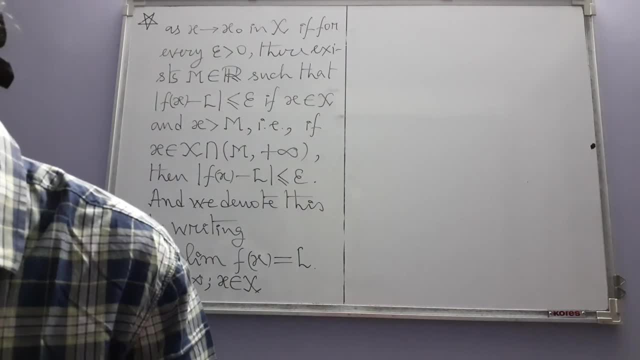 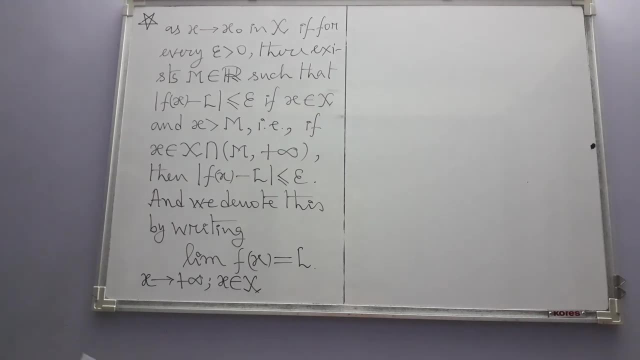 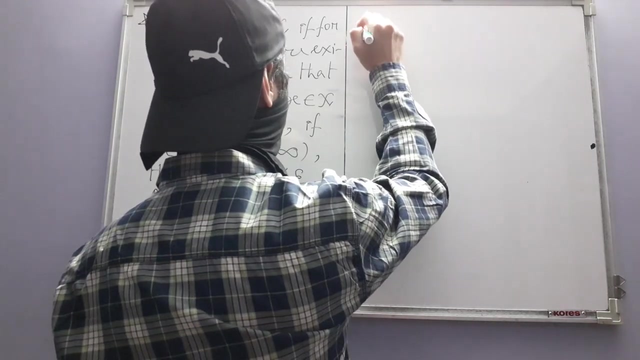 up. That's the problem. And if I put too much ink then the thing will get messy. Alright, and for the second part we have to again write all those things. Let x, which is a subset of R, have minus infinity as an adherent point. 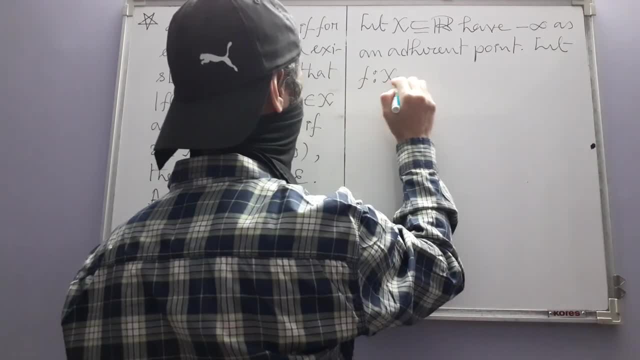 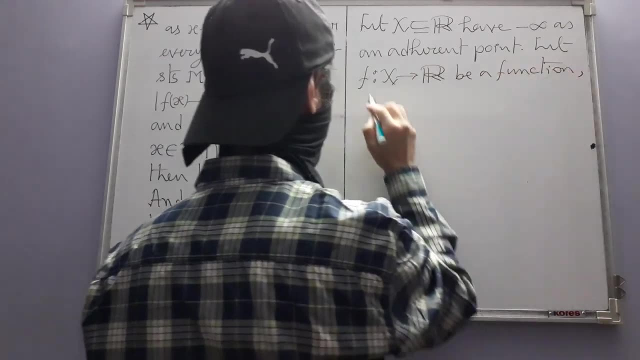 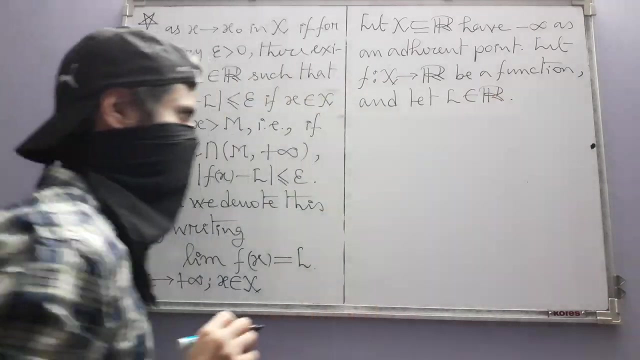 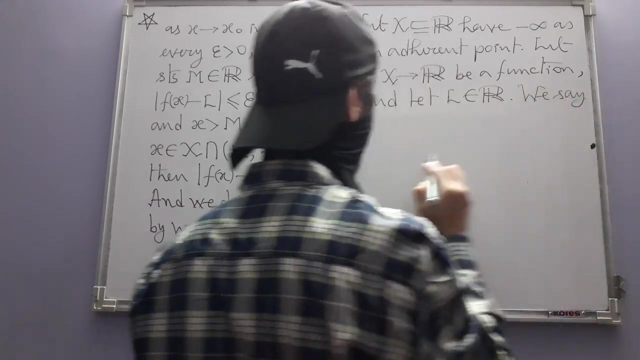 So let f from x to R be a function and let L be a real number. There is no need to write in words, You can just write: L belongs to R. We say that f, x is equal to L belongs to R. So if I say that f, x converges to L, as O See what is x naught? It is plus infinity. 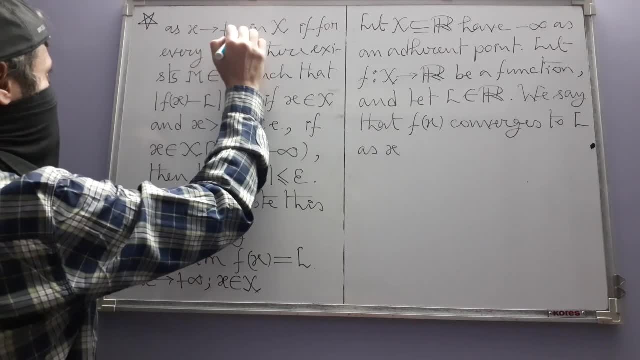 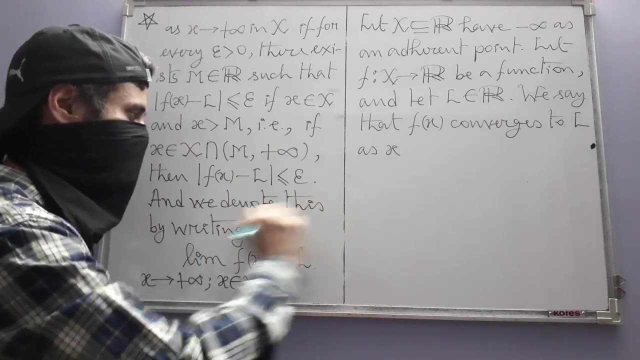 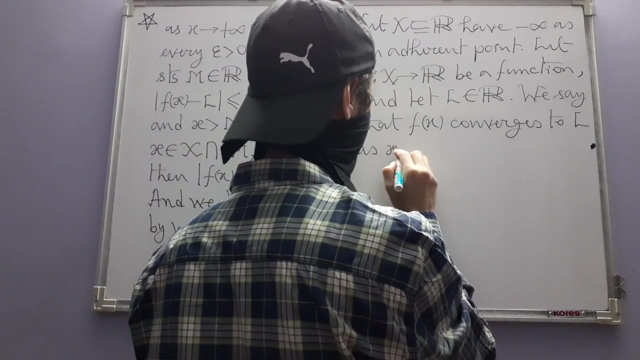 This is how we make mistakes. I was thinking of plus infinity, but writing x naught is a habit, As x tends to minus infinity in x. if for every epsilon greater than zero there exists a real number, M which is equal to f, x, I am writing x, cos x of x and x. 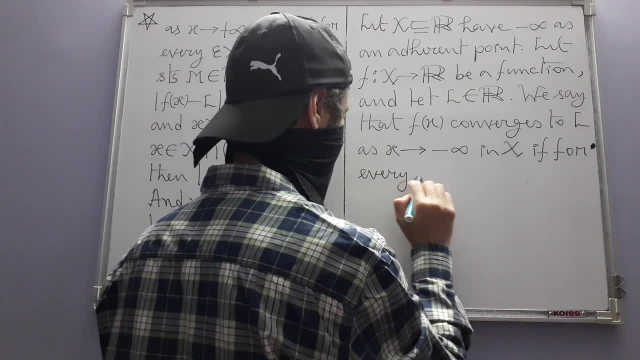 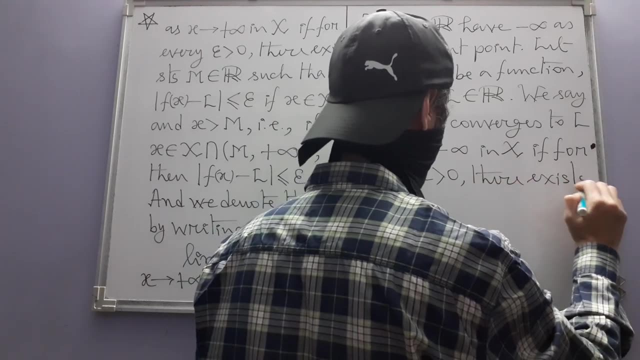 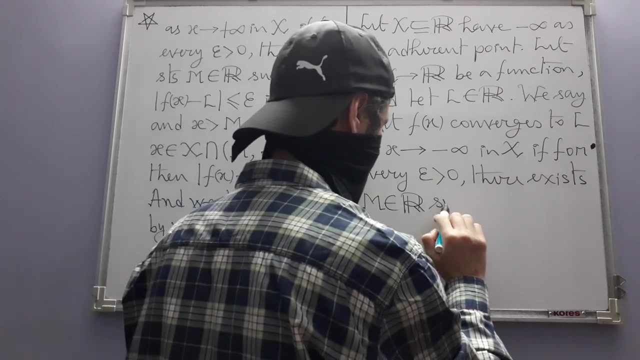 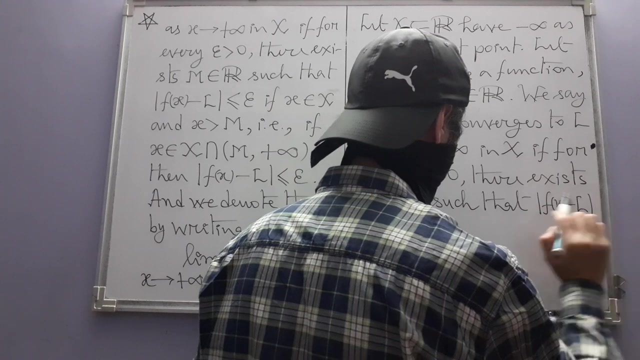 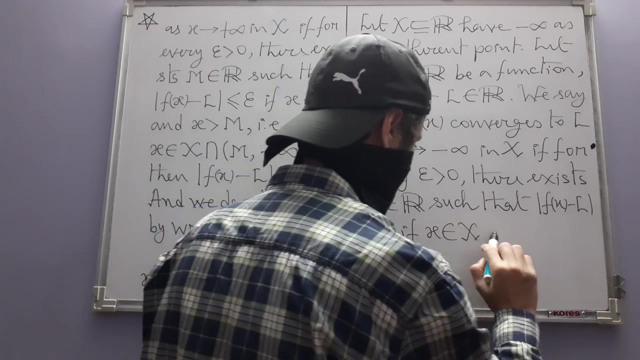 is f? x? This is my question. If I have every epsilon greater than 0, as x tends to minus infinity, I will write as such that f, x and l are epsilon close if x belongs to x, and this time x is less than. 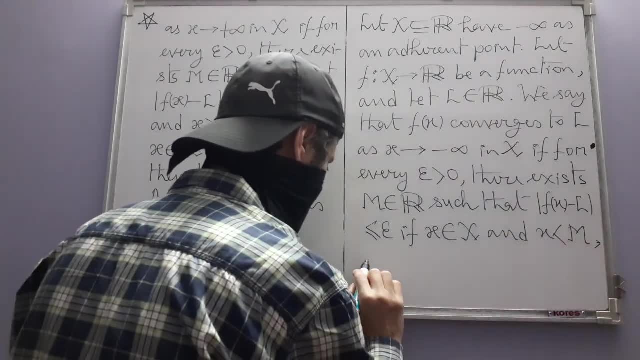 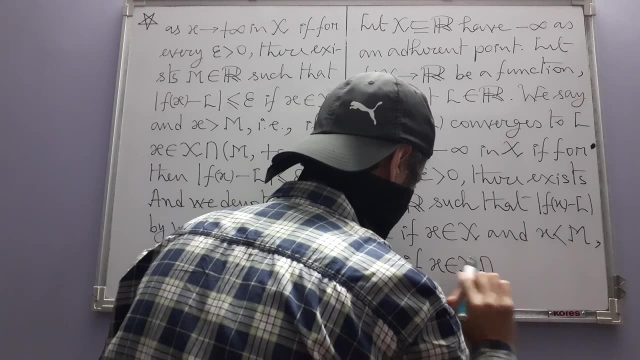 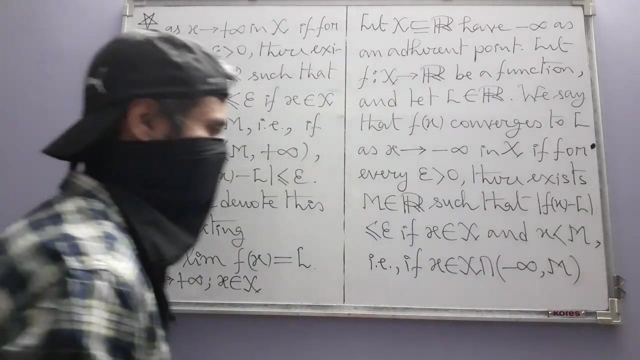 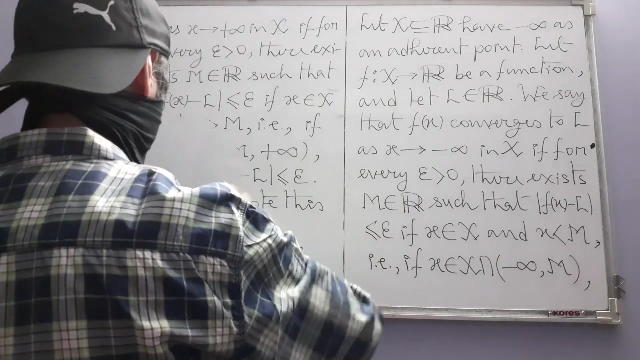 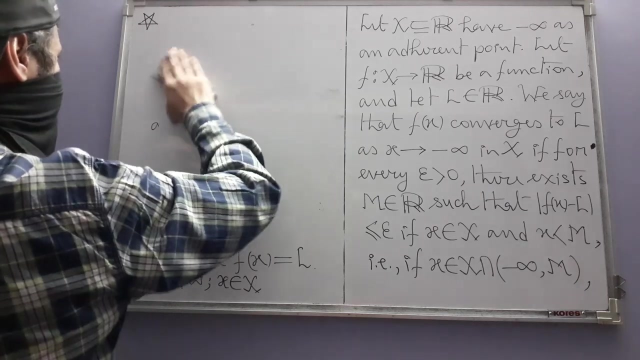 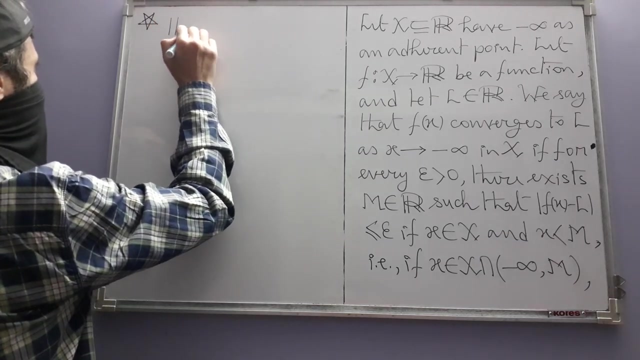 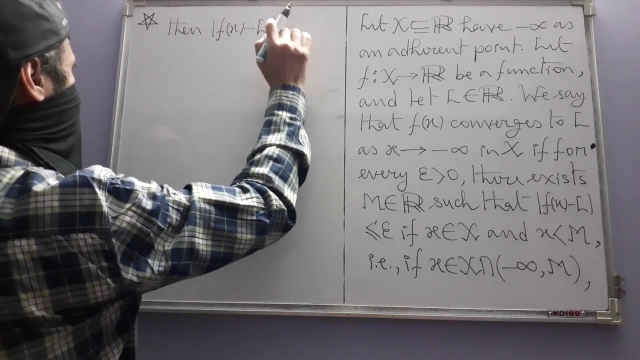 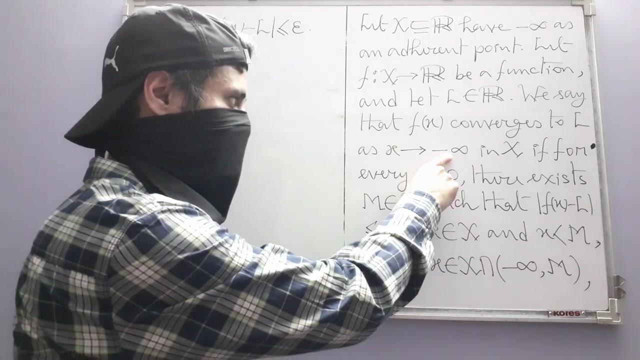 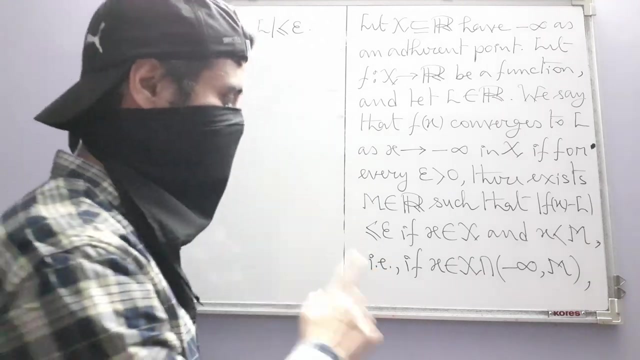 i, e. if x belongs to x intersection, the open ray minus infinity comma n, then then f, x and l are epsilon close. The reason we need x to have minus infinity as an adherent point for this to for this definition to make sense, is because you see: 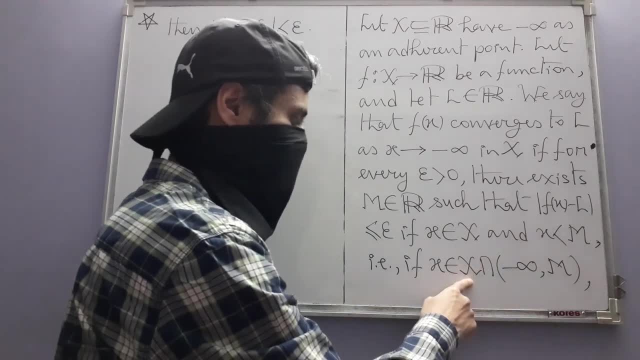 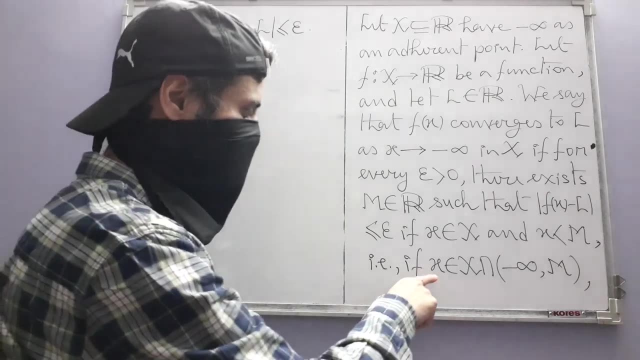 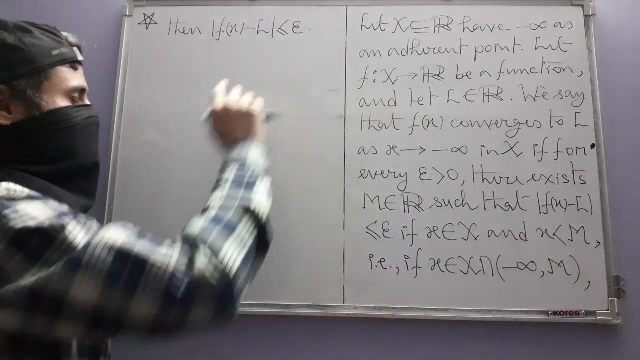 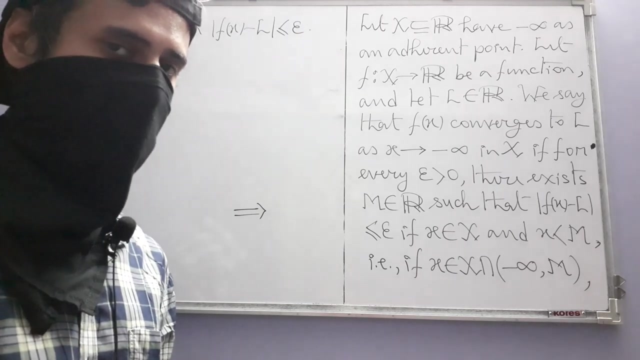 The fact that minus infinity is an adherent point of x makes these intersections non empty. So actually, if you look carefully, you are looking at an implication here. If this happens, then this happens. If this intersection is empty, then the implication will become vacuously true and in that case, 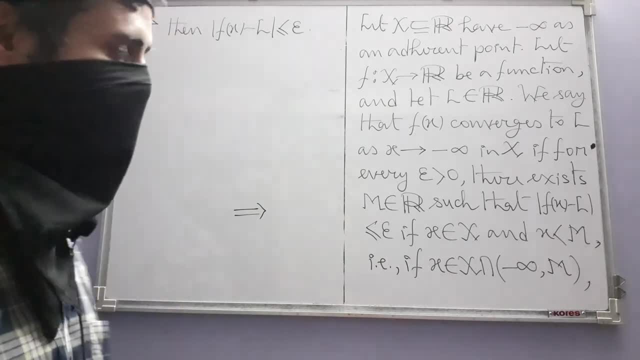 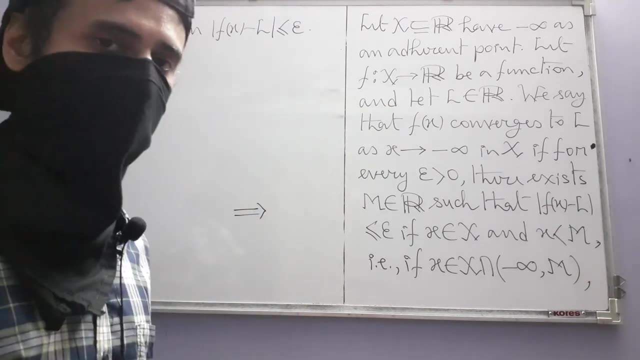 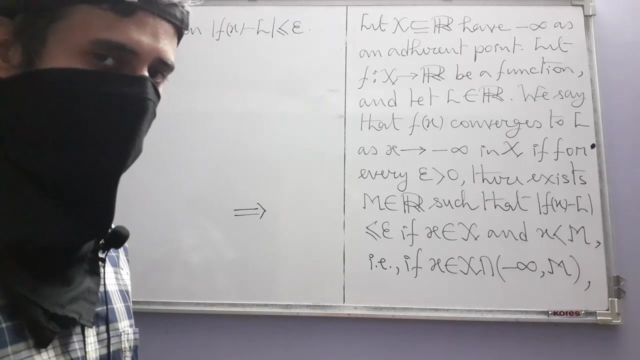 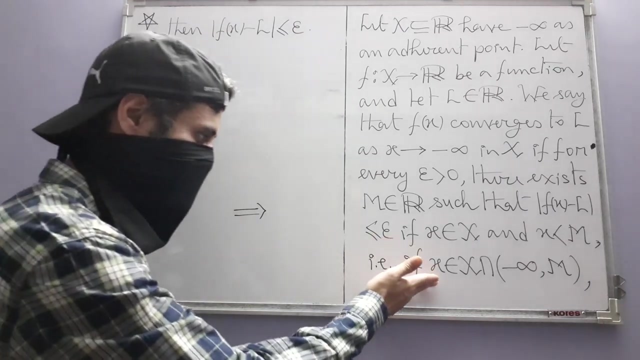 all strange things will happen. For example, in that case the implication will be true no matter what your l is. So it will be actually true for all l and the notion of limit entirely. I mean it is just gone. What we know or what we think limit should be, that idea itself is gone. when such vacuously 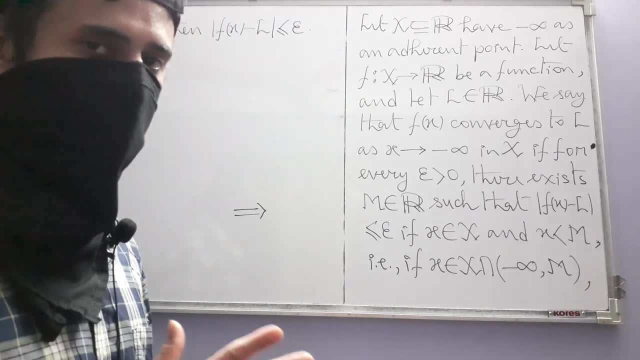 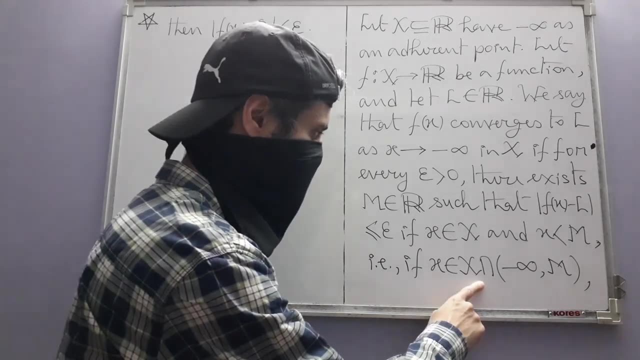 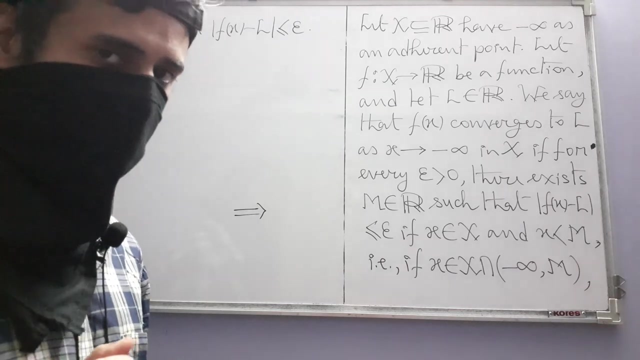 true implications are allowed- I mean technically they are true- But that just makes the whole thing lose meaning. That is why, to avoid that situation, we consider minus infinity to be an adherent point when defining limit at minus infinity. This was also the case for the original definition of limit. 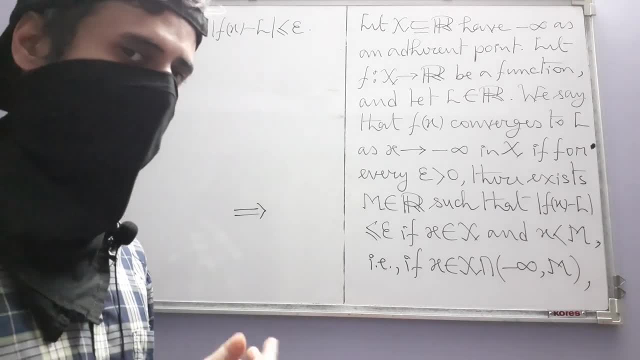 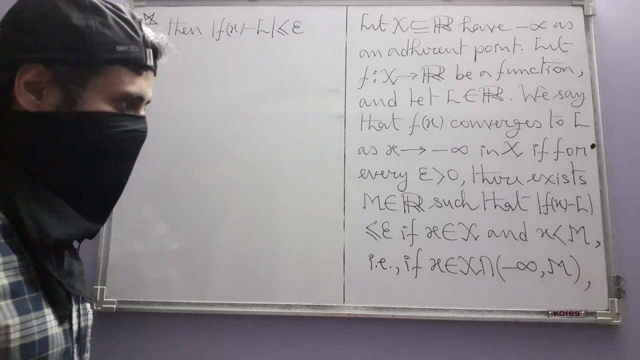 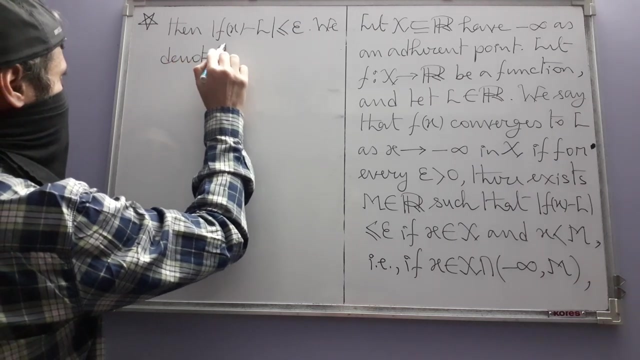 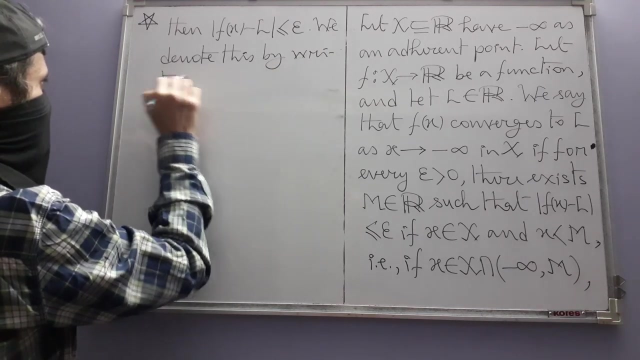 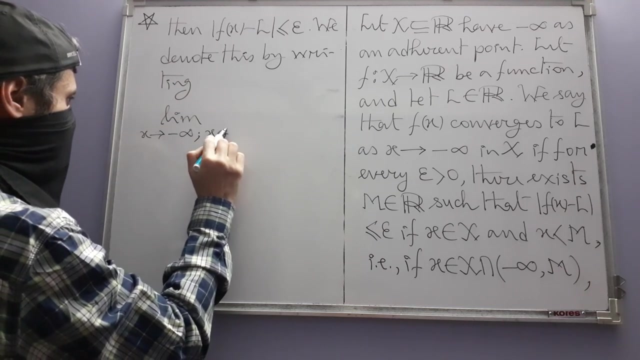 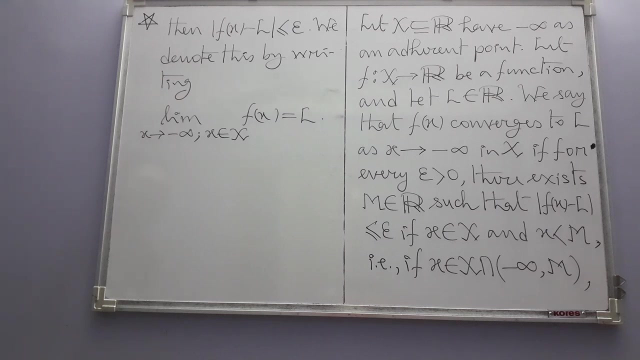 That is why we need x not to be an adherent point of x. We have already discussed this before, So in this case also, same thing happens. We denote this by writing again. a similar notation is there While reading. you should read it like this: 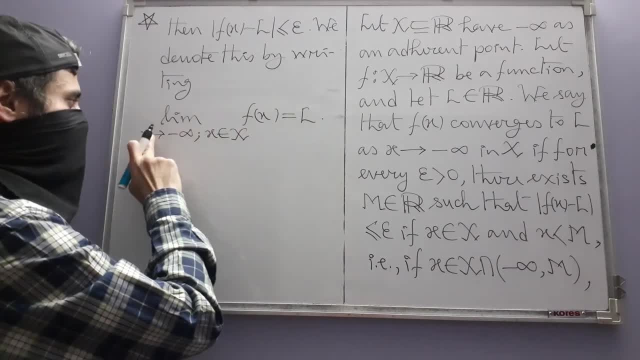 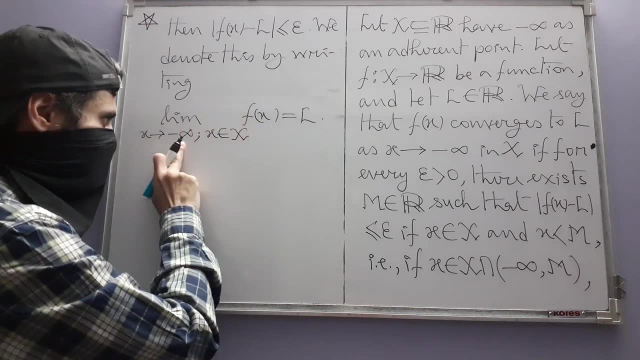 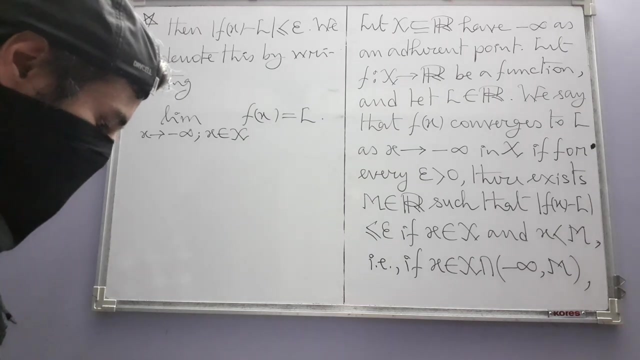 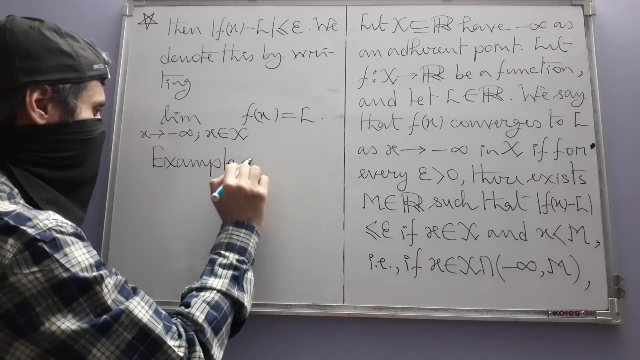 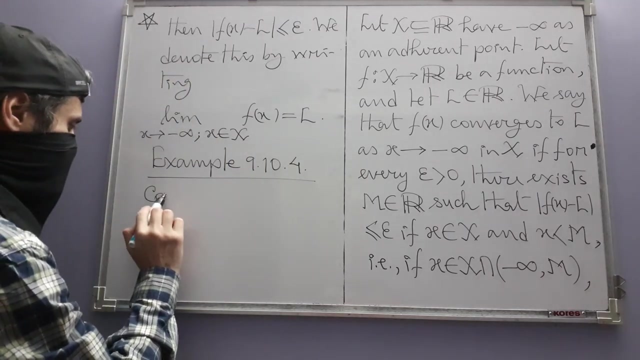 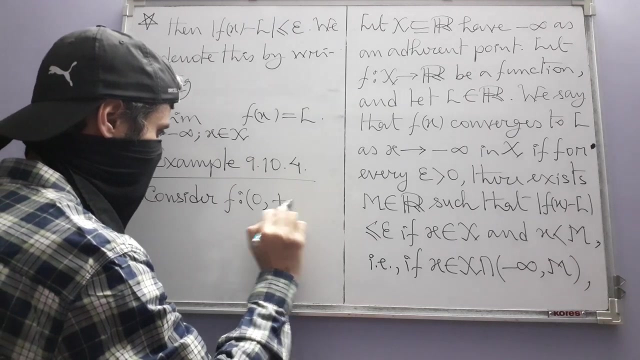 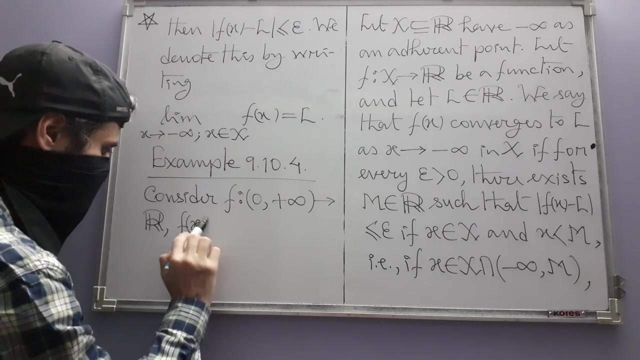 The limit of f x is l as x approaches minus infinity in capital x. or the limit of f x at minus infinity is l in the set x. Let us now see one example. Ok, Ok, Ok, Ok, Ok. You consider this function f from 0 comma plus infinity into r and the rule for the 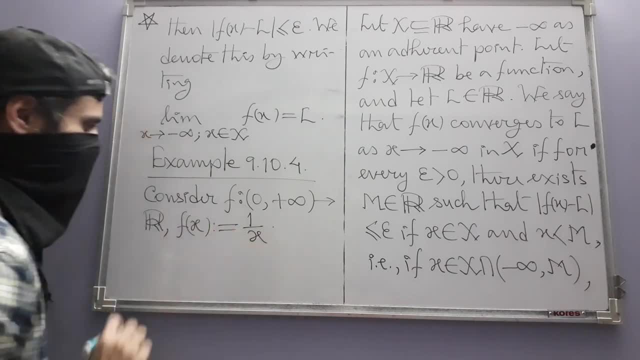 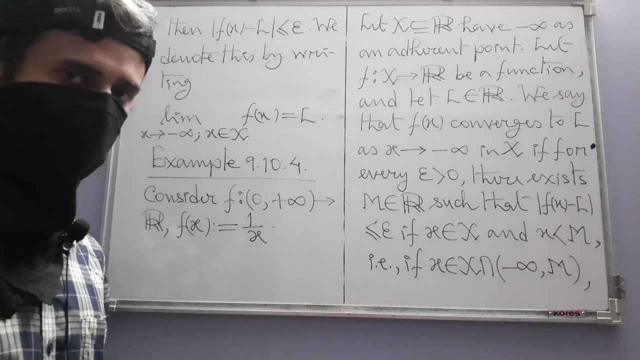 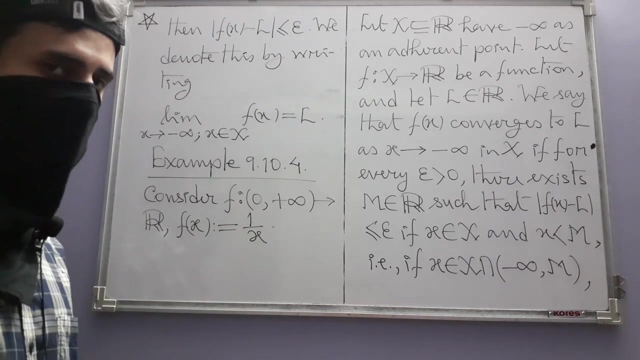 function is? it is just the reciprocal function. The function is well defined because in this interval it is actually the set of all positive real numbers. Every such real number has a well defined, unique reciprocal which also turns out to be a positive real number. So it is a well defined function. 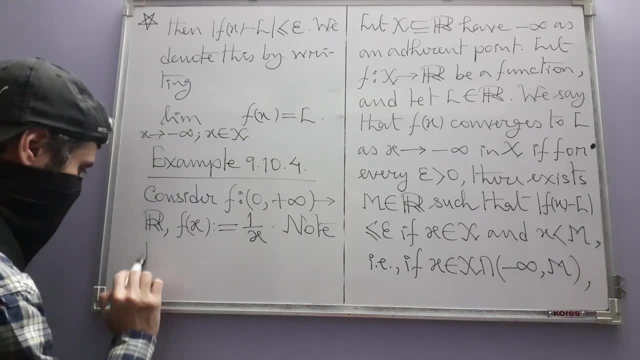 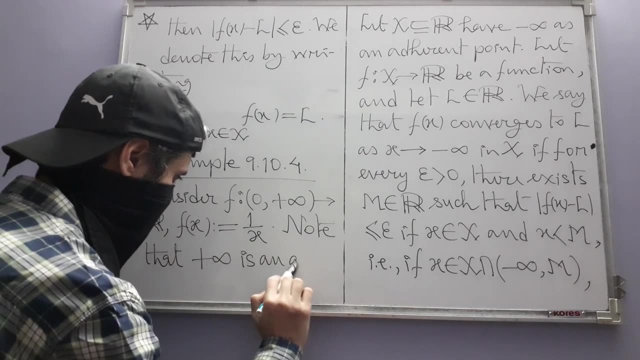 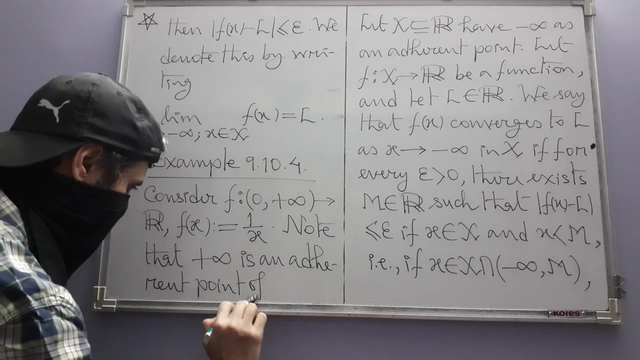 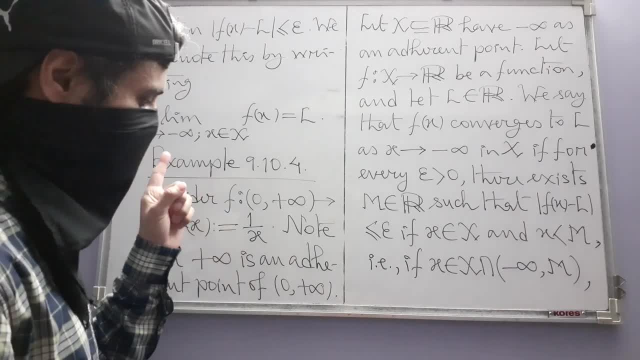 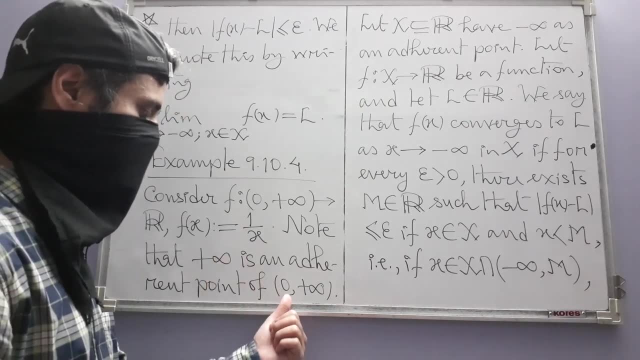 Okay, slogan: subaru flow. So we have just written a function f, the sum of f from 0 to infinity of thatpm times n, k, 3ve, IV over 180, einfach es 0ertado 2x2, 2v 0.. 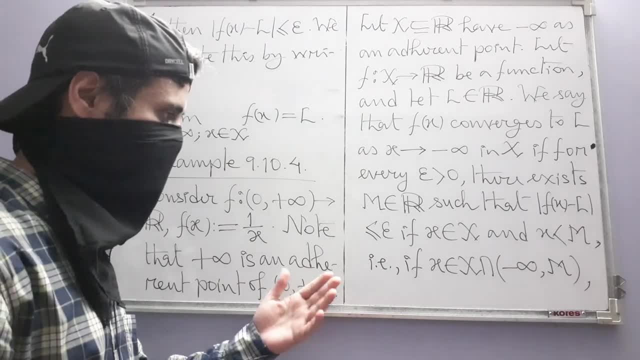 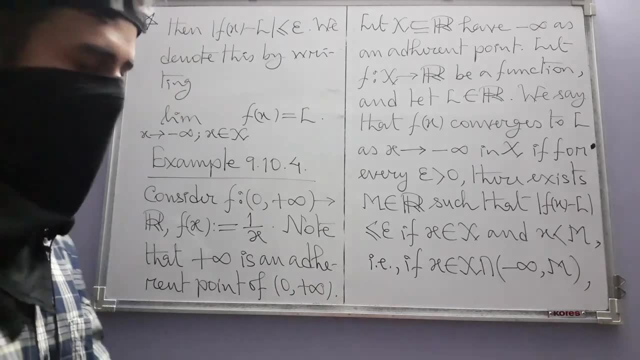 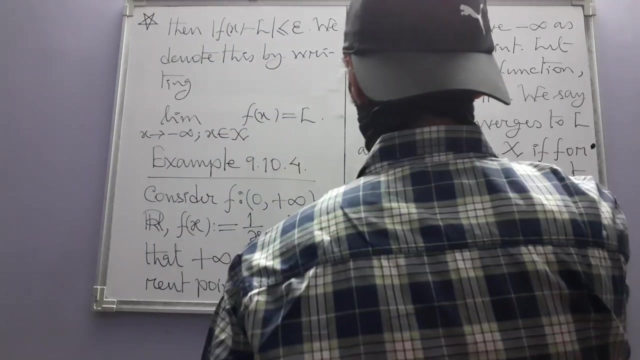 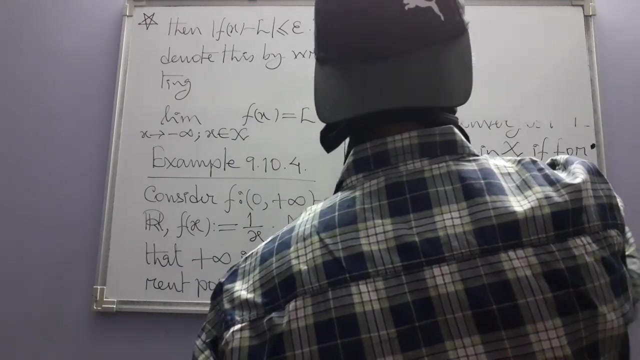 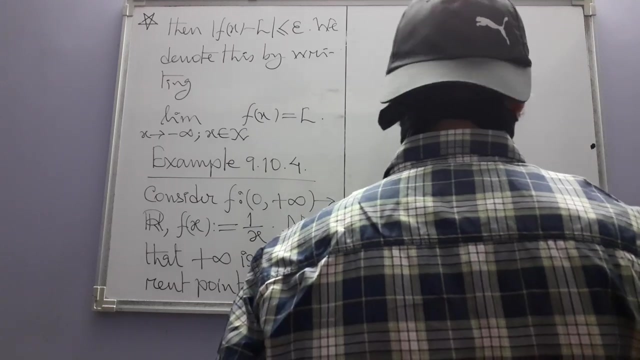 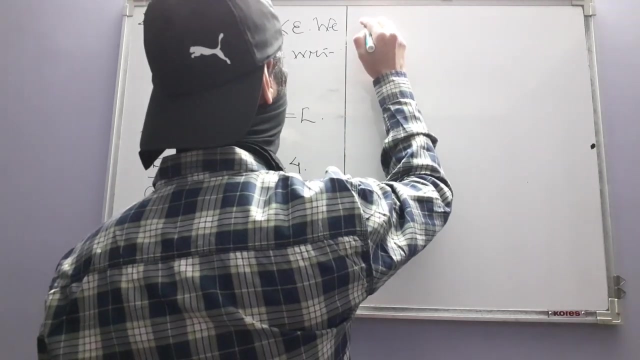 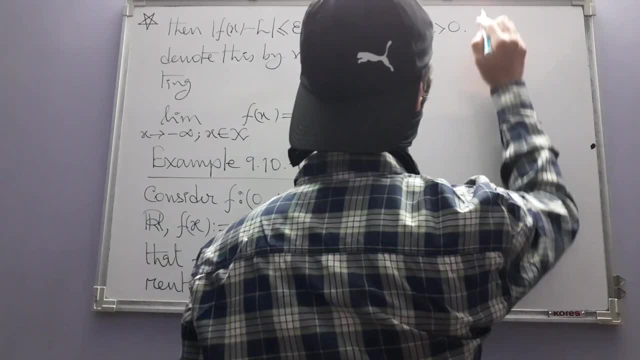 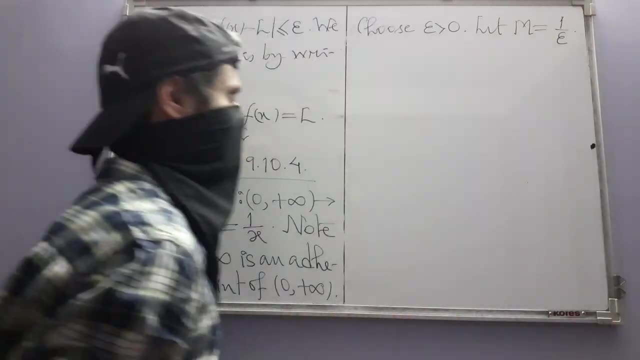 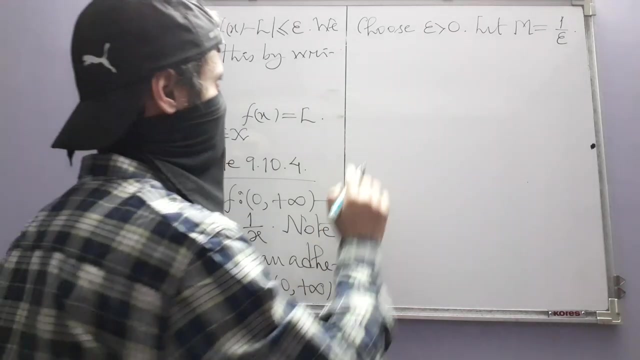 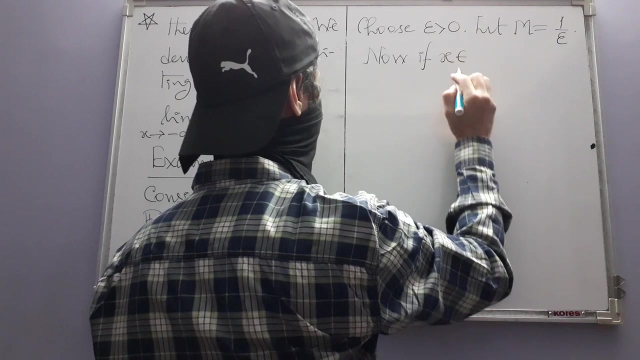 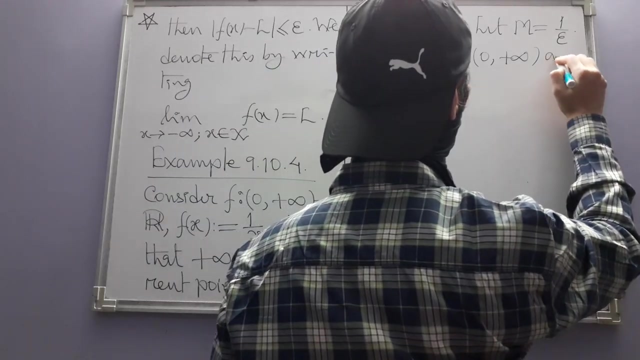 than 0.. Let capital M be 1 over epsilon, which is a legitimate real number, because epsilon is non-zero, So it is reciprocal. exists Now if x belongs to 0 comma plus infinity, and which just simply means that x is a positive. 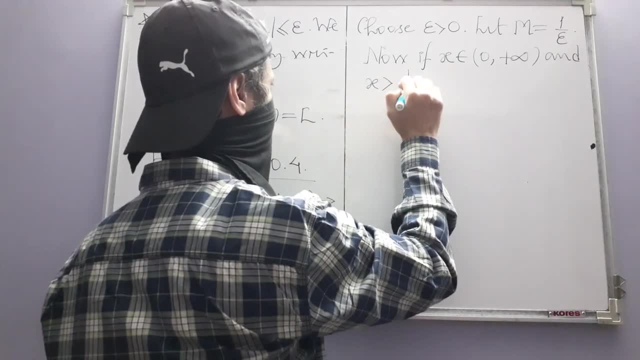 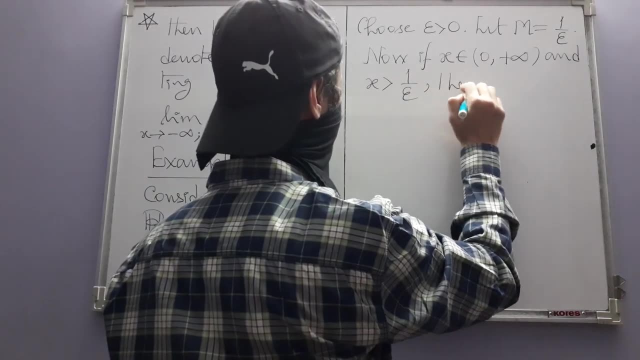 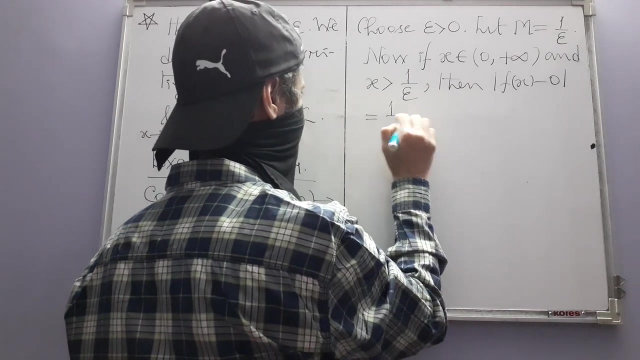 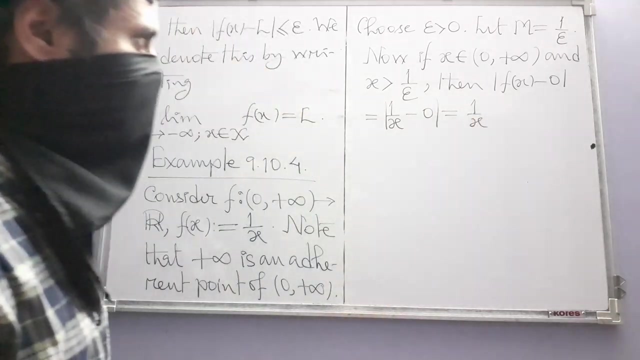 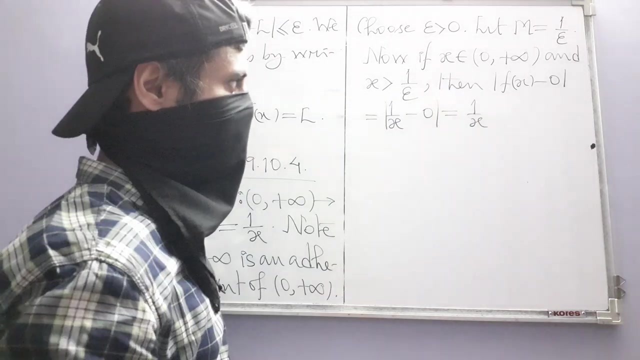 real number and x is greater than 1 over epsilon. Then the distance between f of x and 0, which is this. which is this: Why were we able to get rid of absolute value? that is because x is positive. So mod x is simply x. Now, 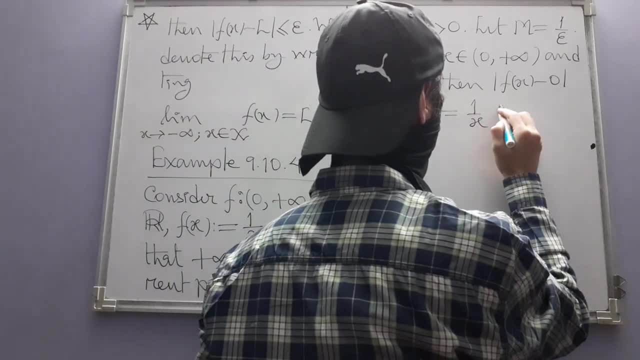 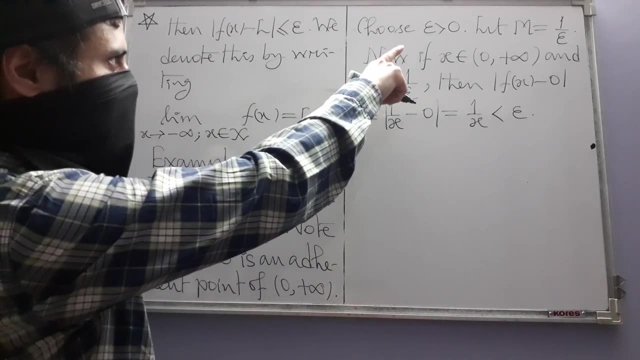 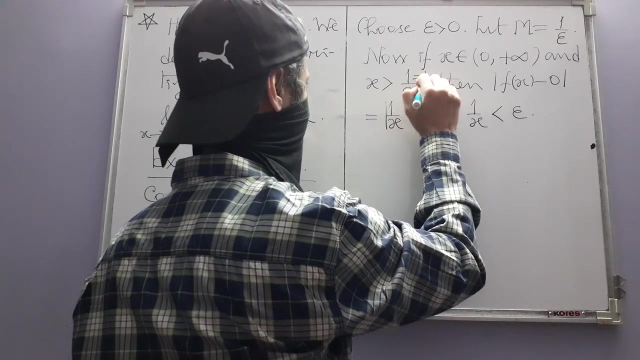 x is greater than 1 over epsilon, So 1 over x is less than epsilon. but you see, what we have shown is that, no matter what epsilon is, there exists an M, such that, if these conditions are true, Actually you can write M here, because we have given this a name now, so that is. 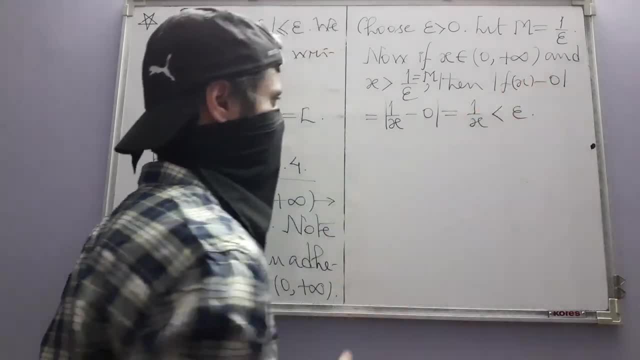 M, Then f. x is epsilon close to 0, but then by our definition. hence this is an root. I think now we are able to write the Monica ripple. This is basically what we see in m. No, Well, that is not all that we know, as of course. we see it here. It is the grains question And in m Sr até, the related product of m and m. What you see here is heater at the moment of decay, b par k, which will give 0 to zero. So if, if, epsilon is 0 and then, instead of that, so that is 0. This is 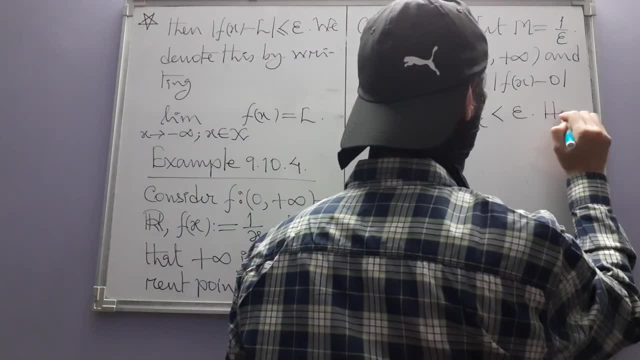 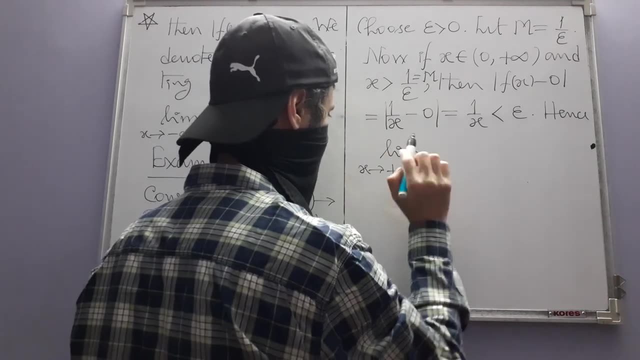 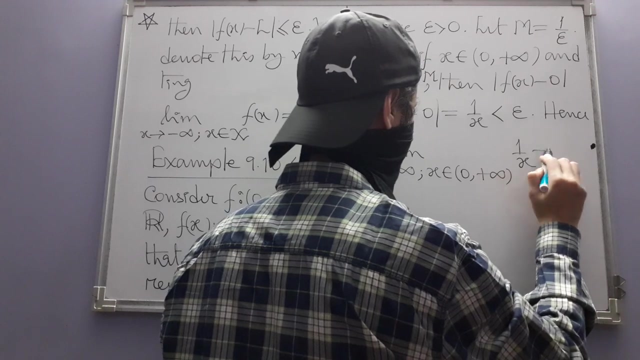 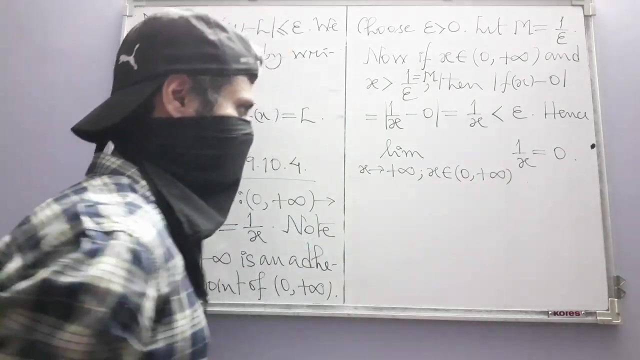 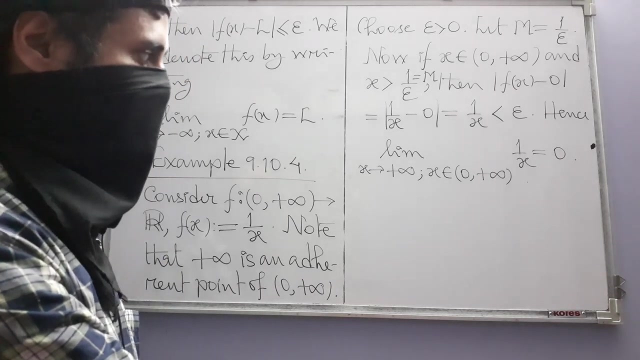 than by our definition. Hence, x belongs to 0 comma plus infinity f of x, which actually is 1 over x is equal to 0. I mean, we already know, or we can guess, that this limit is 0, but now we have the precise formal definition and using the definition, using first principle, 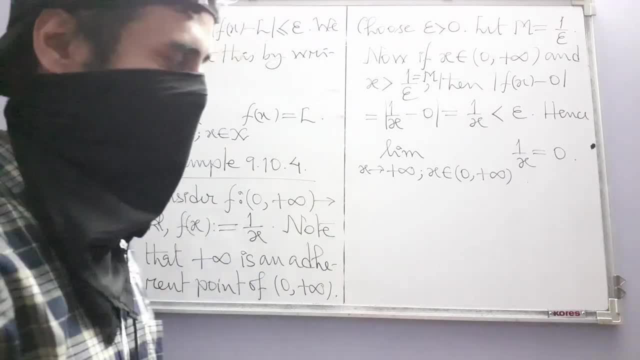 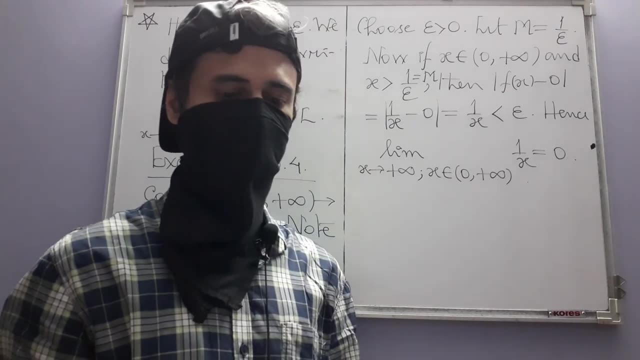 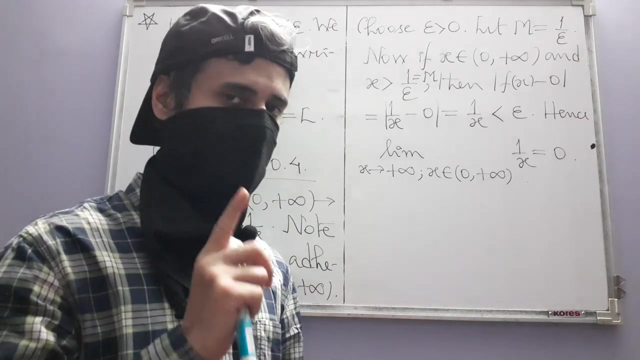 we have shown, in fact, that the limit is 0.. Now it turns out that many of the things that we have seen, many of the properties of limits not at infinity but at some real numbers, x naught. We have seen many properties like 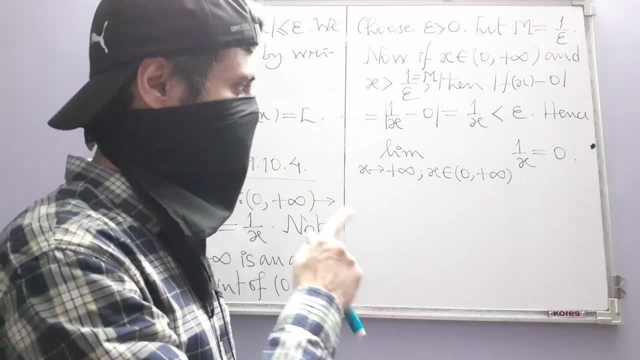 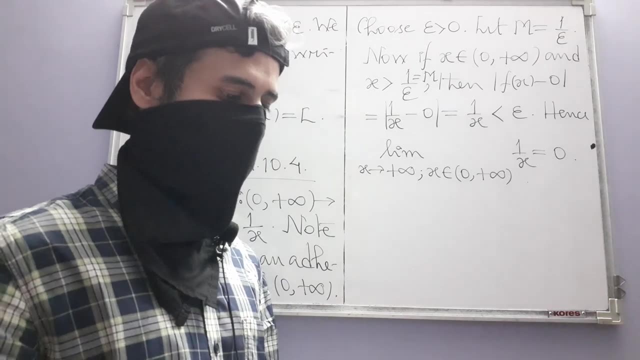 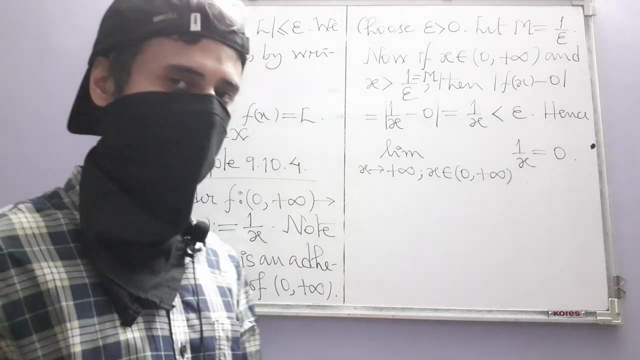 algebra of limits of x, naught And many other things. They turn out to be true for limits at infinity as well. But the thing is that, for instance, it turns out that all the limit loss still continue to hold even for this type of limits, But the thing is that we won't be using these limits at 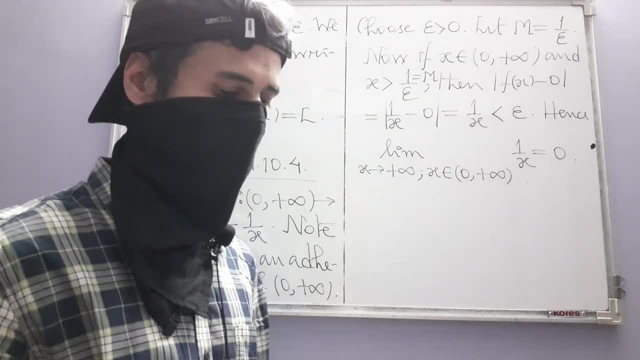 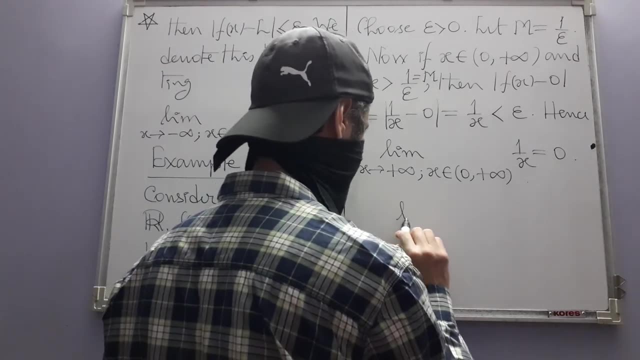 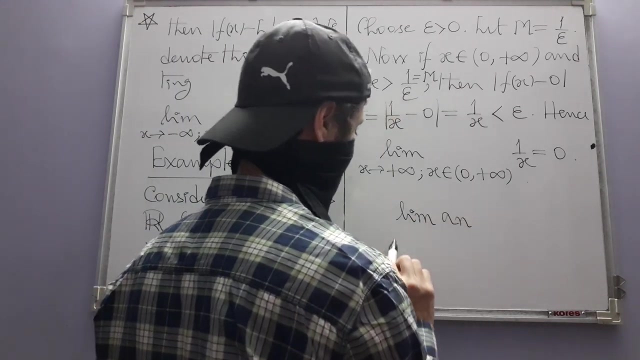 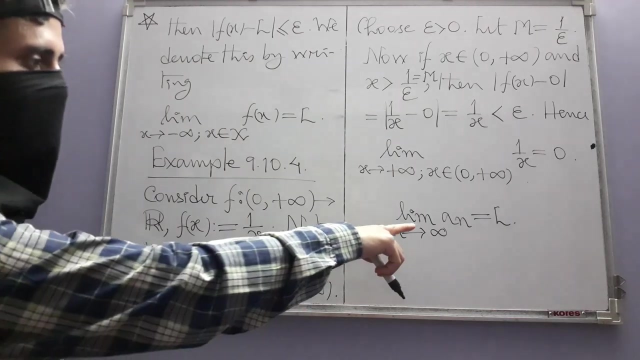 infinity much, So we won't bother about them. There is one more thing, however. You see, we already have seen way before seeing these things: limits of functions, limits of sequences, limit of a sequence of real numbers, a, n being l, And in all such limits n always approaches. 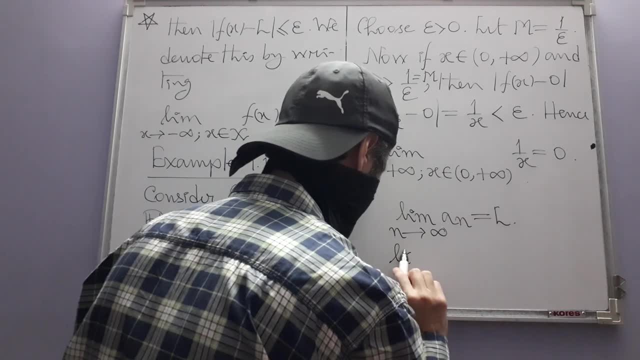 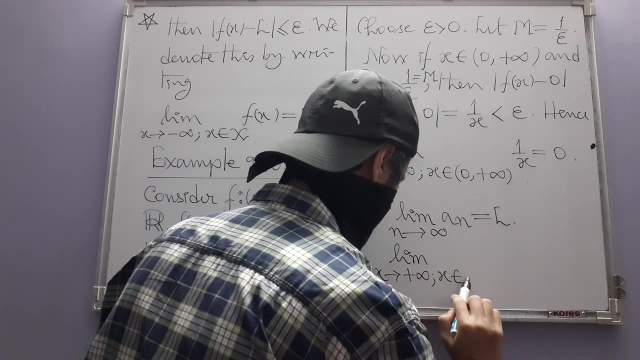 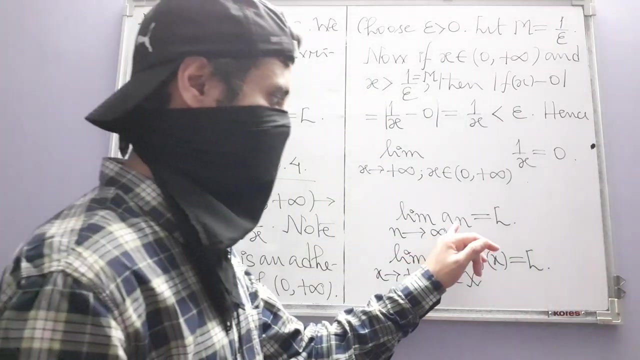 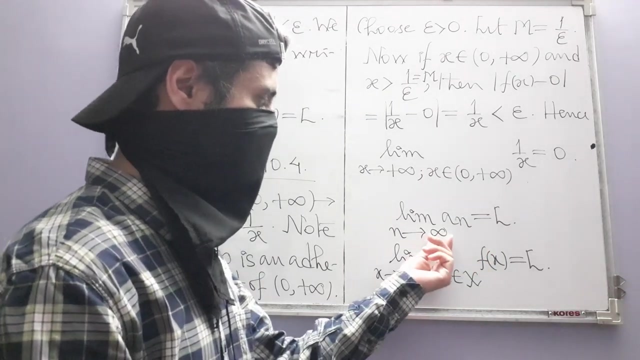 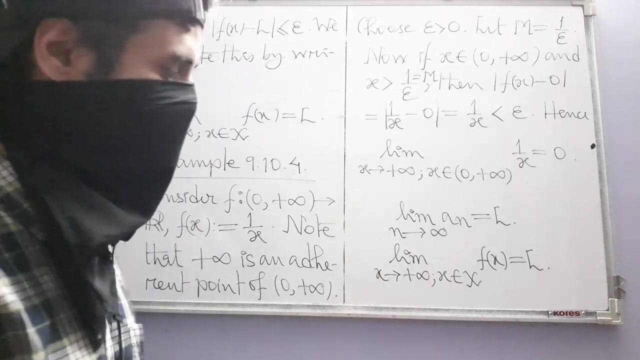 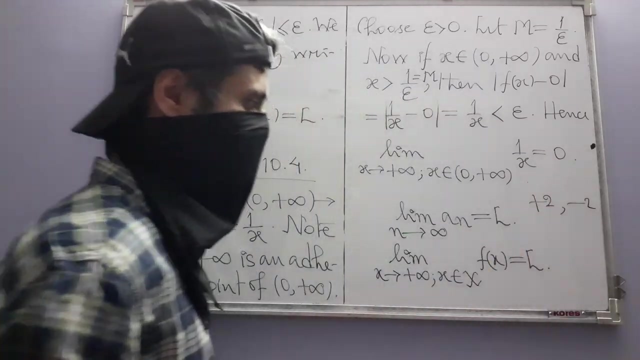 infinity. Now we have a similar thing. the difference is that there we had a sequence, here we have a function, here we have plus infinity, here we have infinity. is that a difference? no, because infinity is a simpler notation for plus infinity. it's like 2 and minus 2: 2 is actually plus 2, but we do not write the plus. 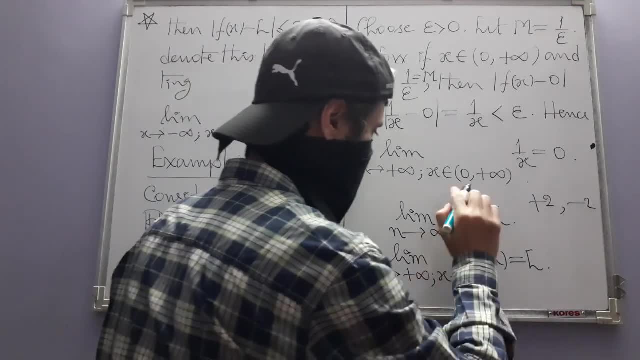 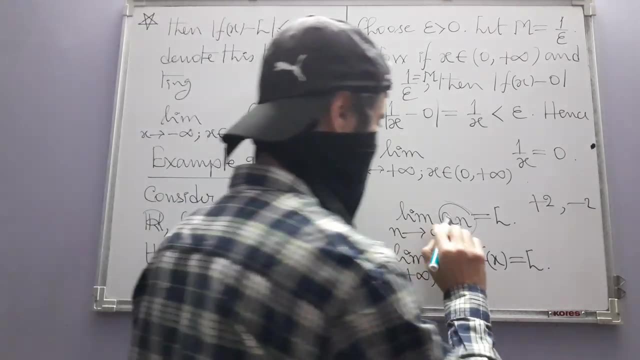 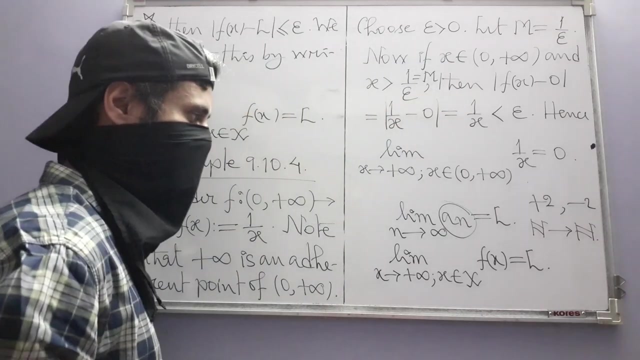 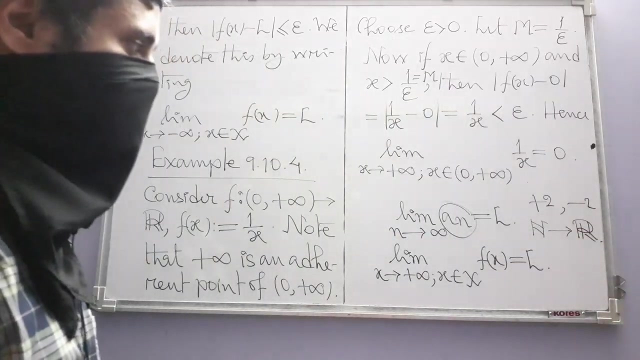 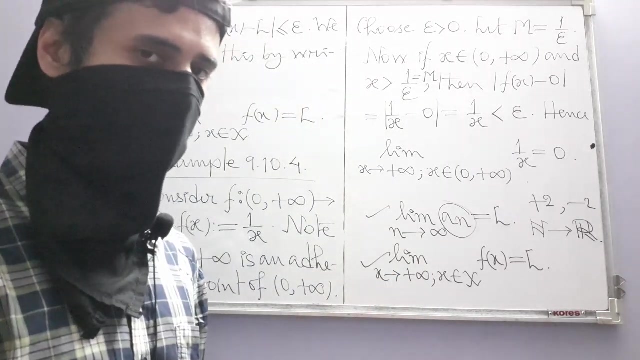 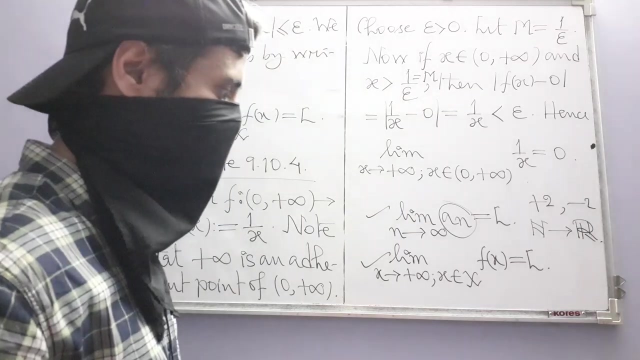 now. is a sequence also a function? yes, it is a function. for example, this sequence is actually a function from the set of natural numbers, oh sorry, in into the set of real numbers. so are these two notions somehow related? and the answer is yes, they are actually the same thing. i mean, when in place of fx you have an, you will see that the 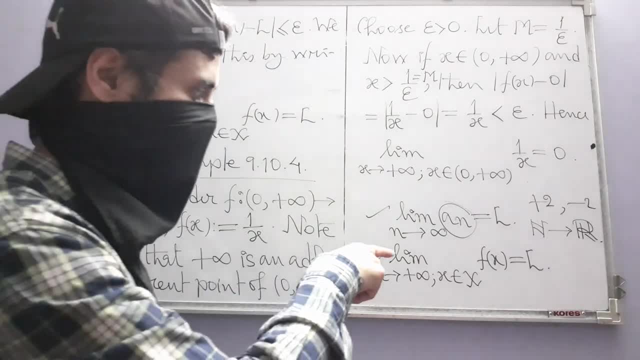 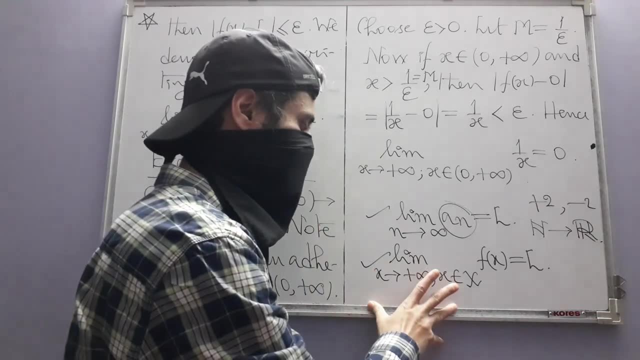 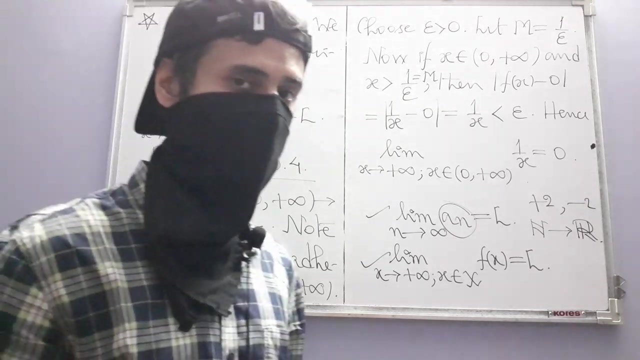 limit that this definition gives you is nothing but the limit that we have already seen for sequences. this is the only exercise in this section and it's the last one which we will solve, of course, in the community section when the time comes. that means next sunday, and with this, this very small section is over, and 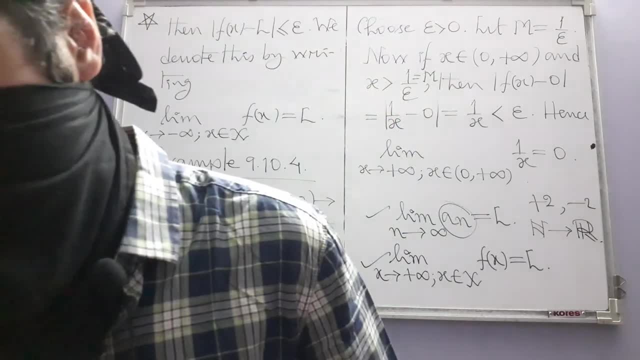 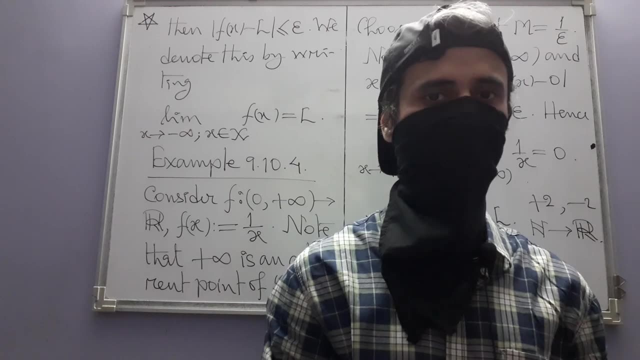 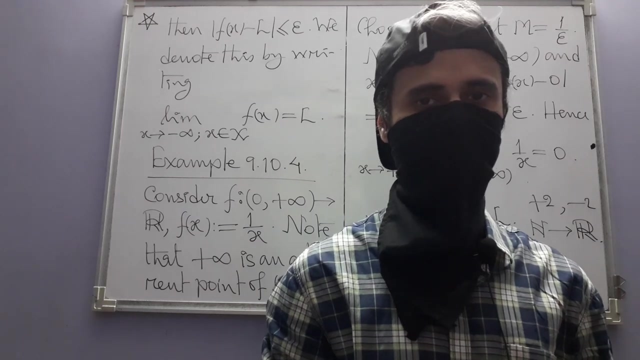 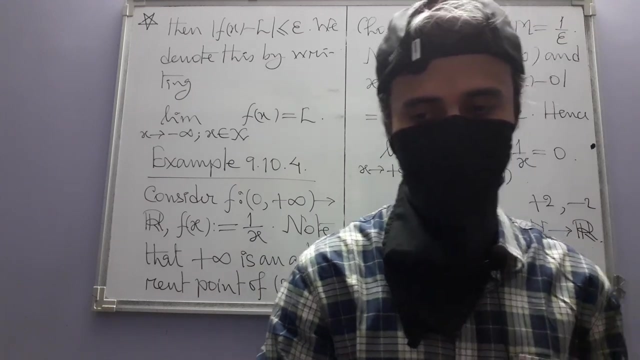 this chapter is also over. after this we will start differentiation, which can be called the heart of calculus. i mean, we are doing analysis, but after all we are doing calculus, only much more rigorously than how we do calculus in school. but anyway, that's just it for tonight. so 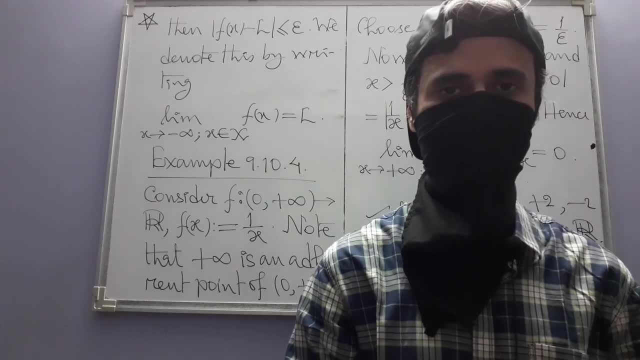 see you in the next upload. until then, this is me, lucifer, from a mathematical room. have a nice night.